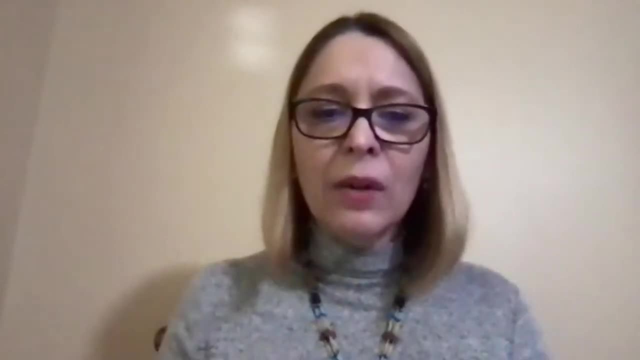 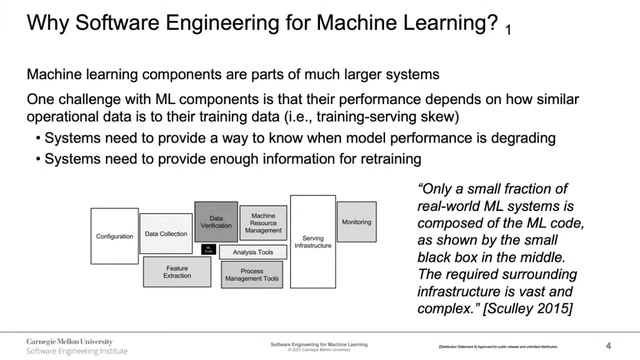 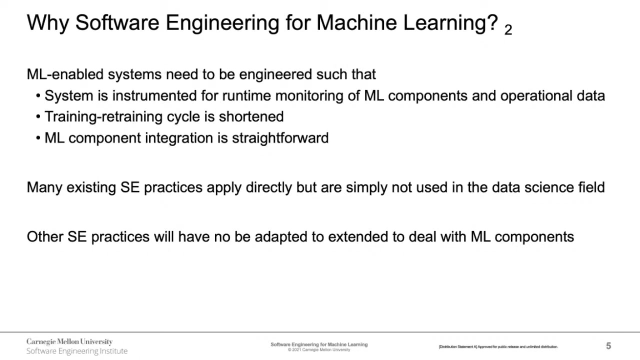 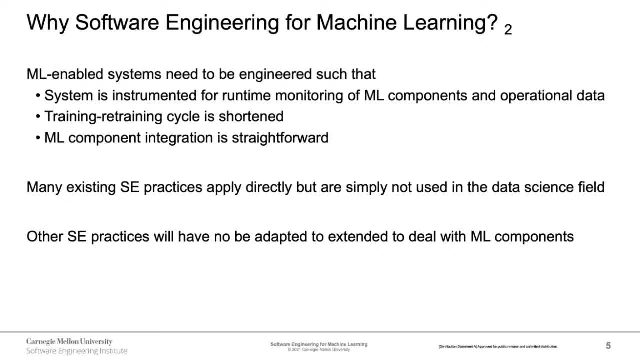 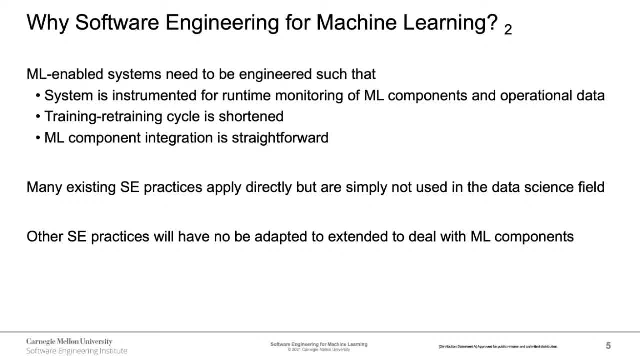 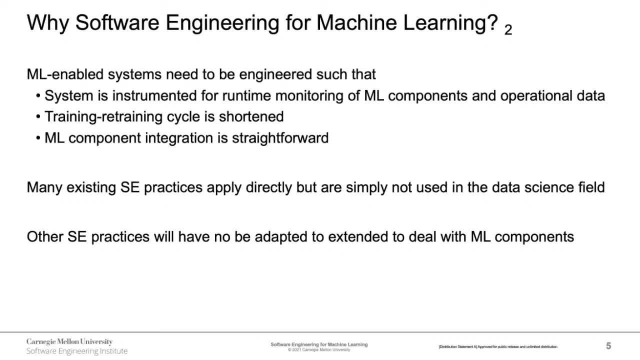 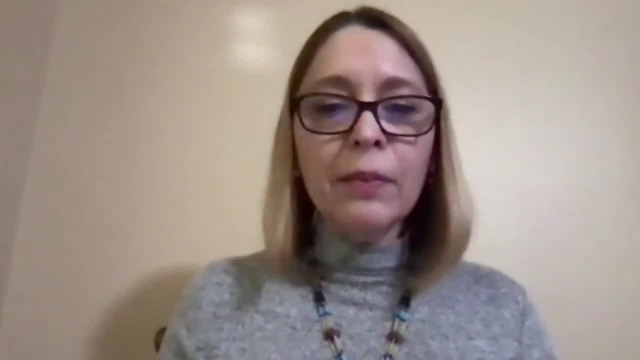 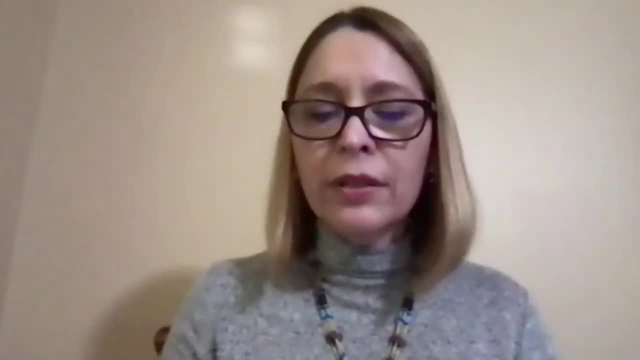 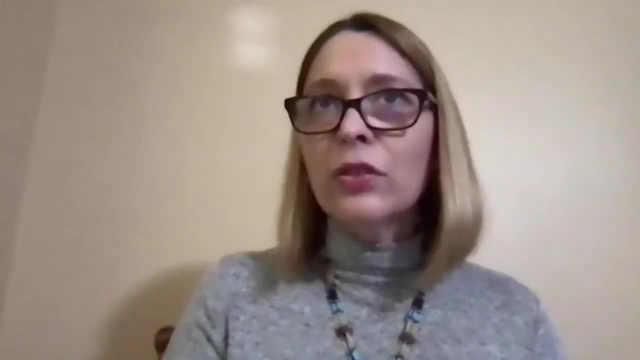 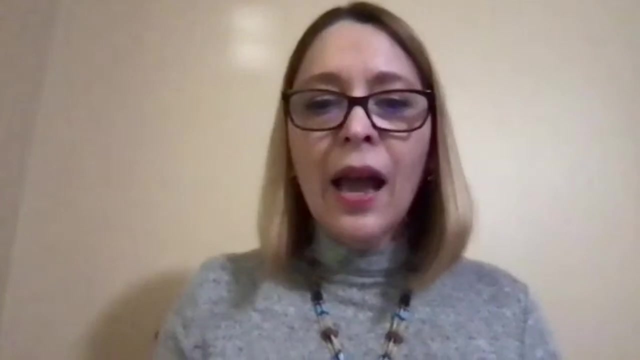 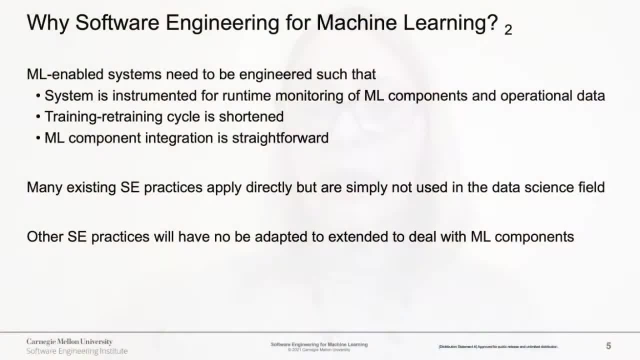 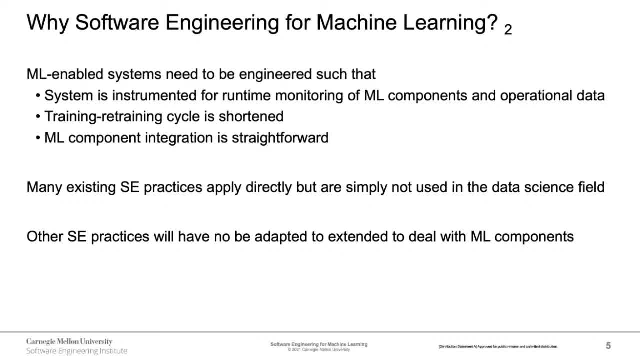 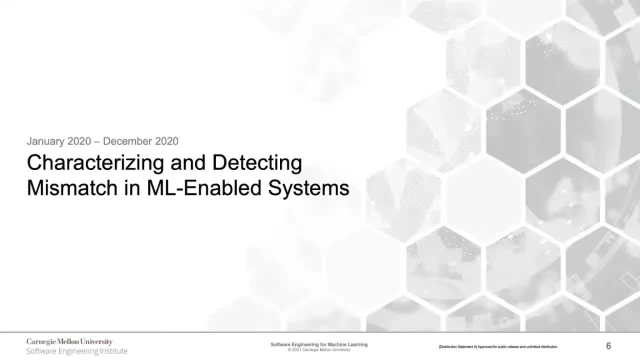 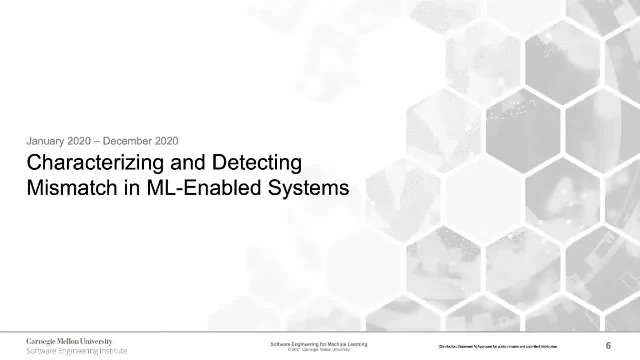 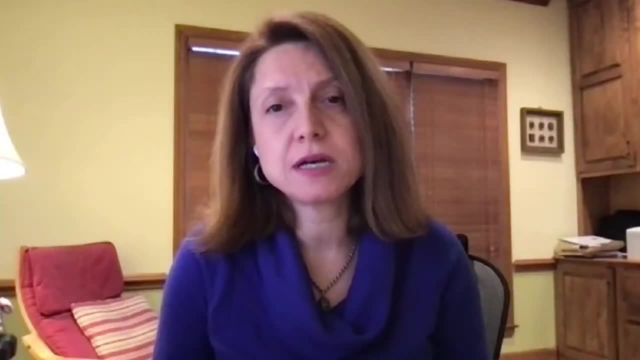 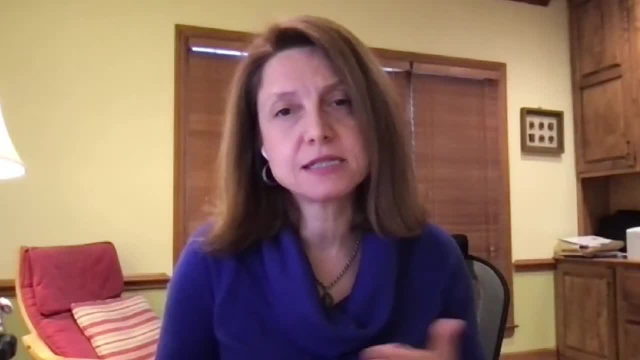 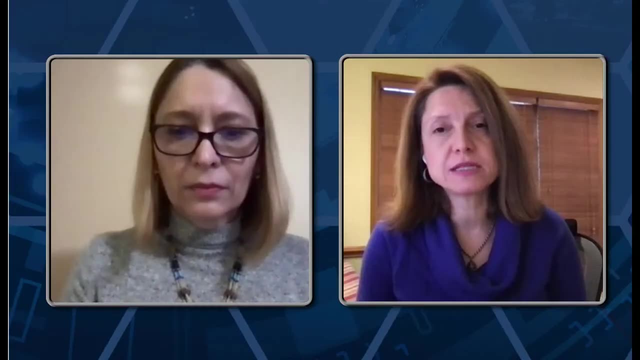 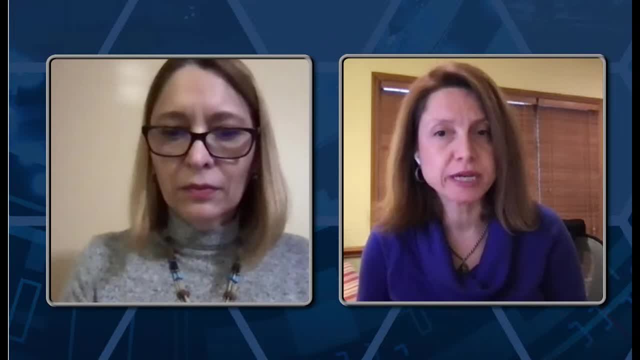 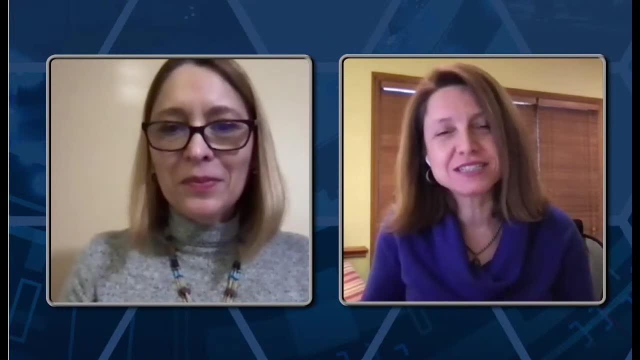 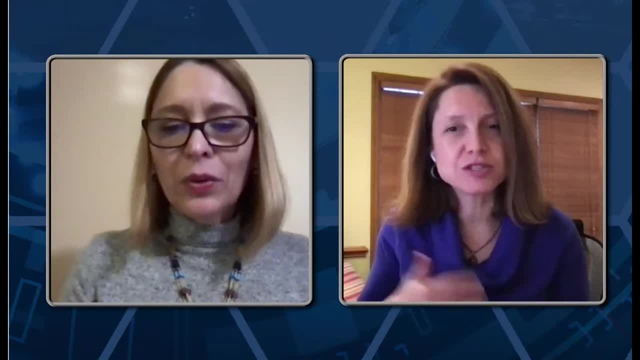 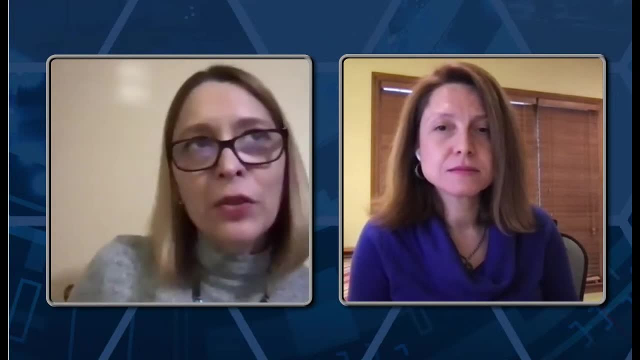 Thank you for watching, as at the SCI, but there's that: how software engineer can help ML and what are some of the practices that software engineers need to be aware of. Yeah, so let me actually let me use the unit testing example as also as an example of something. 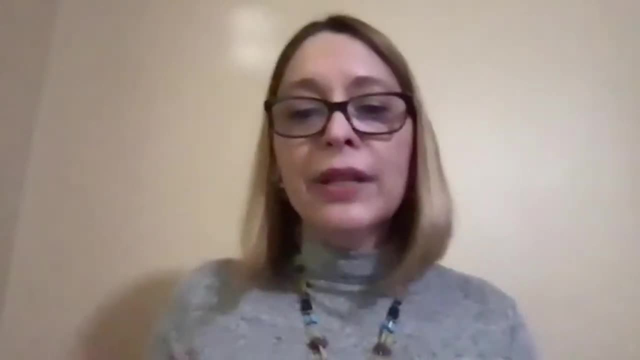 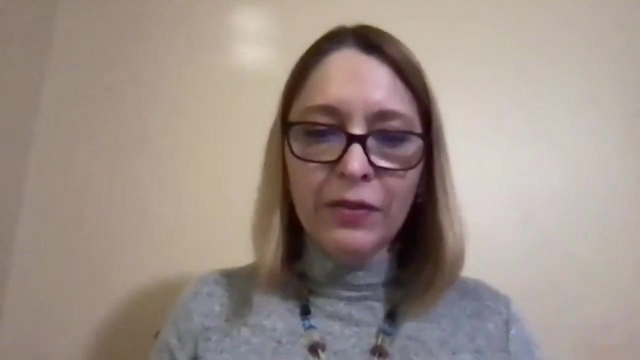 that software engineers need to keep in mind. So when software engineers, when we develop unit tests, we basically say, okay, these are the inputs that I want to test against. If the output of this particular component is five, then it passed. 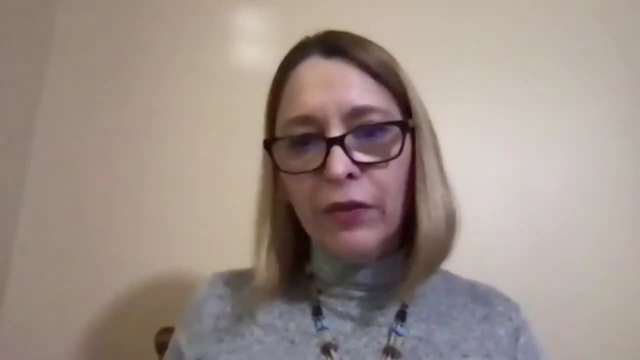 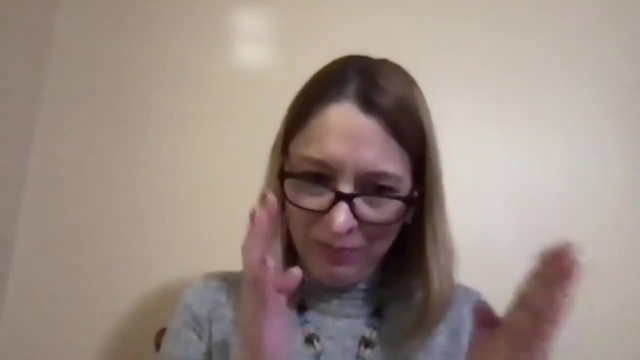 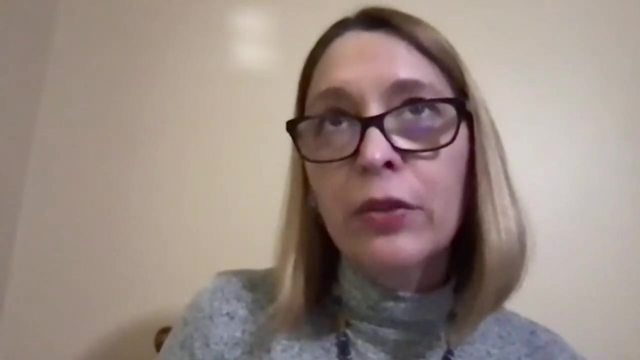 If the output of this component is minus three, then that's a problem, that's a fail, And so we're really used to these deterministic answers like this component produces this output. But we really need to be aware of the nature of machine learning components. where, right now, 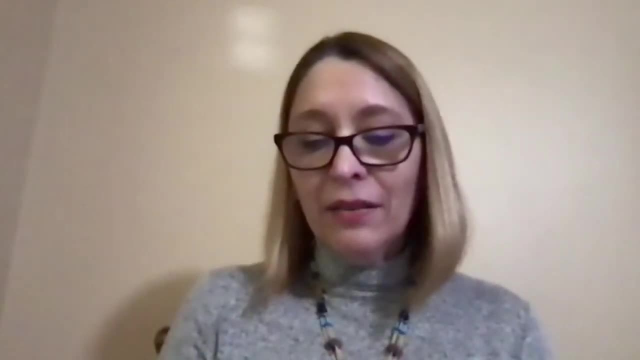 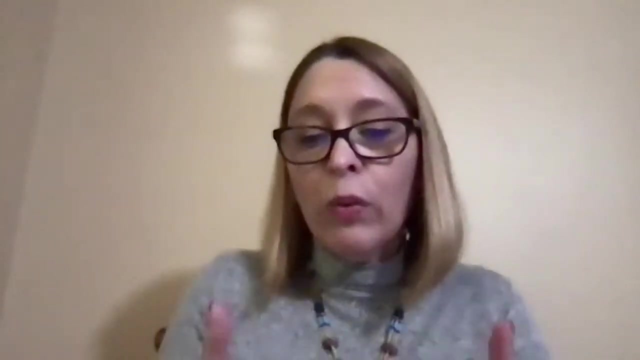 based on what it's seeing right now. that model might produce a five or it might produce a seven, And those are still valid answers because, for example, what we are expecting to see is a range of things. So, for example, for a software engineer, 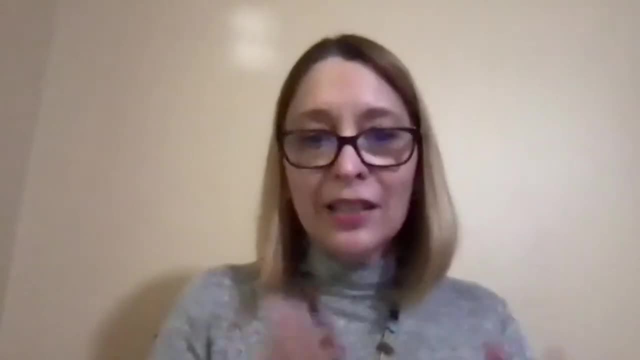 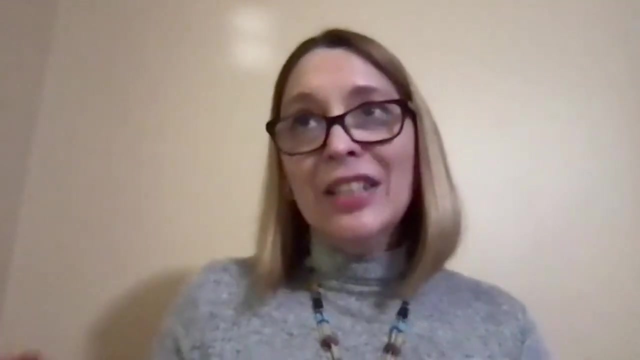 being able to express those outputs not in deterministic terms, but, for example, in ranges, or, for example, by talking to a data scientist. I could say: okay, you know what? the output doesn't have to be five, six, seven, eight. 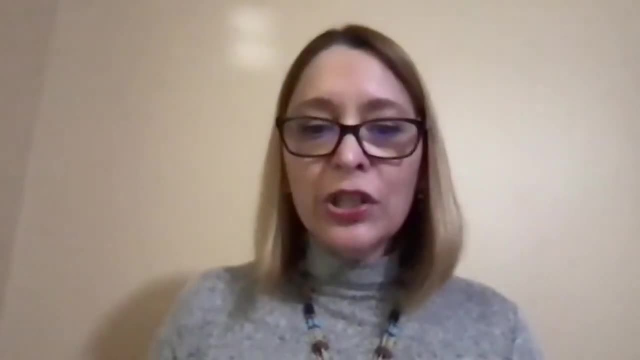 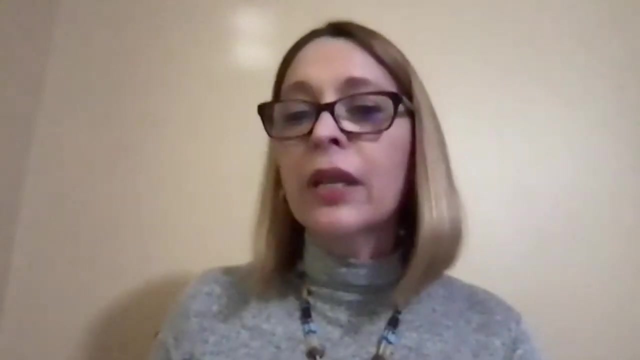 but I really do expect these outputs to be in this order. So just changing into that mentality that it's not always going to be deterministic And, for example, being able to write unit tests which are very different, is one thing, one example of a practice. 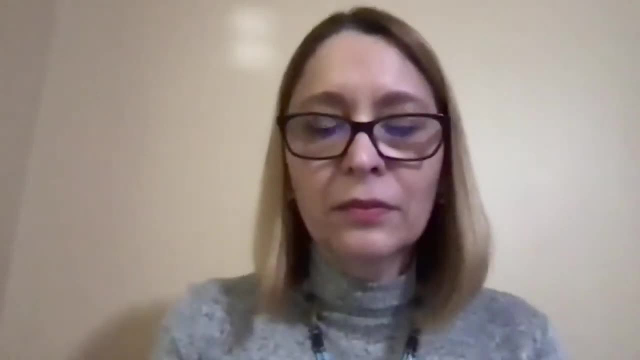 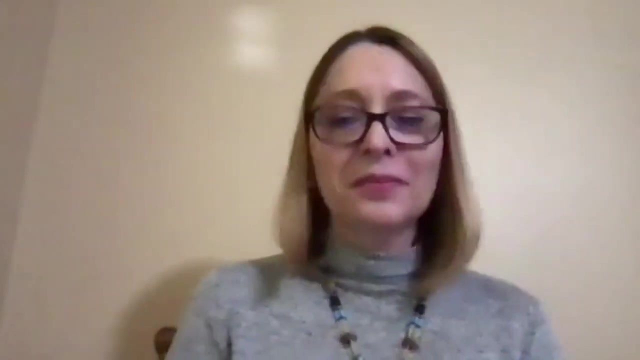 So I think bottom line, what you're saying is some of our known assumptions will definitely not hold, and we do definitely want empirical evidence to be able to look at, which is actually the project that you're just going to talk about. So thank you. 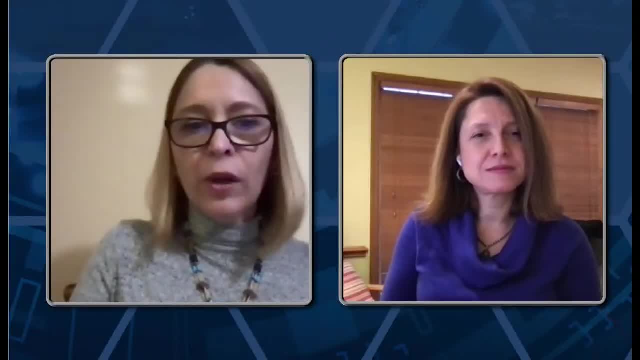 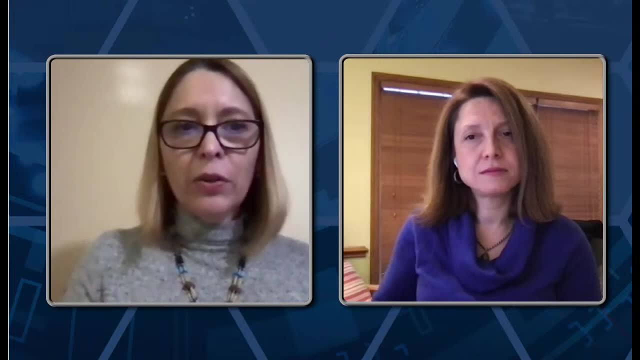 Exactly. Thank you very much. Okay, so let me start with this project. Like I said, this project just ended and I'm happy to say that it successfully ended. So you're going to hear a term. we use a term called ML-enabled system. 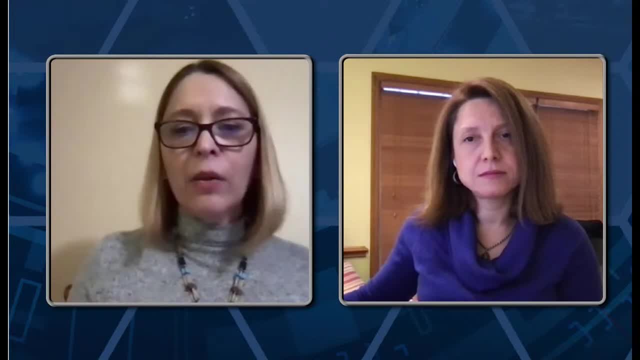 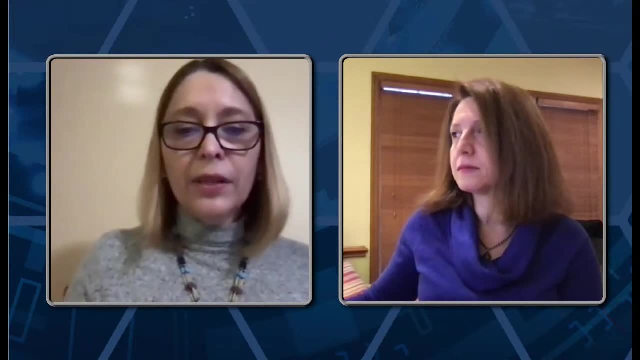 What we're defining in ML-enabled system is a software system that relies on one or more of these machine learning components to provide required capabilities. So, first of all, these machine learning components. it's basically a trained model that is wrapped as a special type of software component. 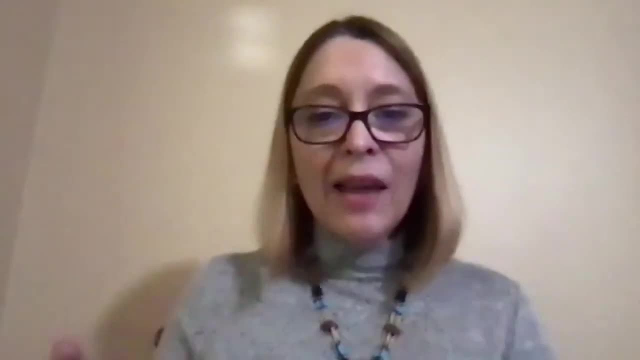 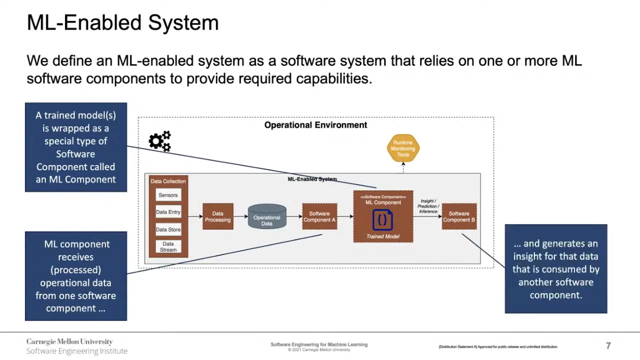 that we're going to be calling an ML component. That ML component is going to receive some kind of processed operational data from one software component and it's going to generate an insight, a prediction and inference that is going to be consumed by another software component. 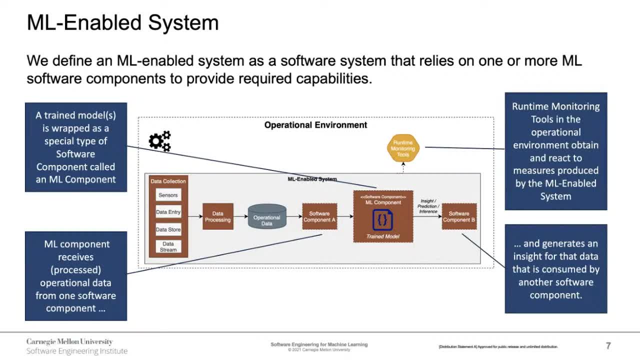 And on top of that there are going to be runtime monitoring tools in the operational environment that are going to be measuring the accuracy or the performance of that machine learning component. So that is an ML-enabled system. It's not a standalone model, It's not something that runs on a desktop in a corner. 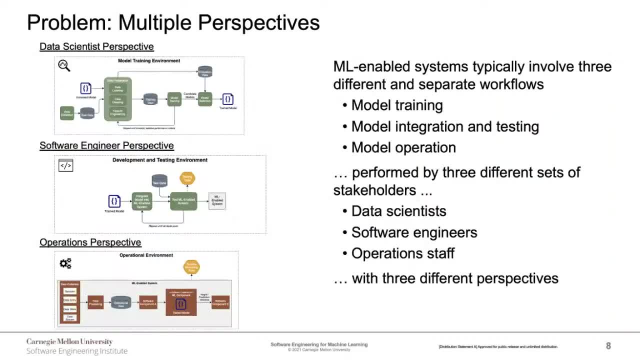 It's a machine learning component that is part of a much larger system, And one of the problems that we had been seeing that really triggered our research in this area is that is this problem that we're calling the problem of multiple perspectives, If you look at how these systems are developed. 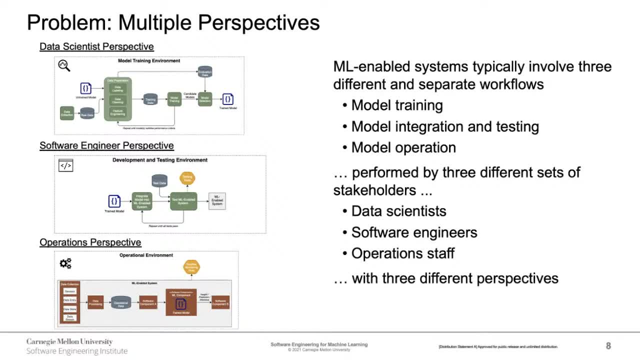 they're developed by three different teams with three different knowledges and three different workflows. So, for example, you have the data scientists that are typically trained in statistics, in machine learning, and at the end of their process they go from raw data all the way to a trained model. 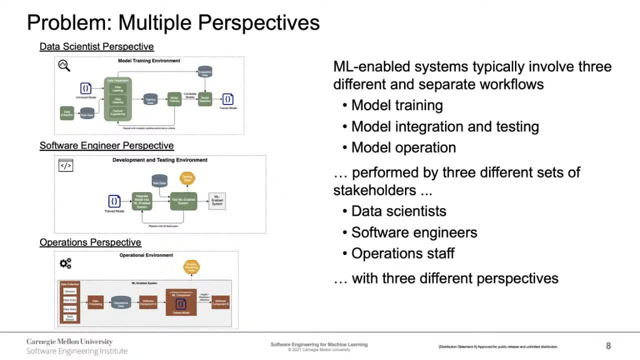 That model is then passed onto a software engineering team for integration into a larger system and testing And finally, that system is then deployed and then is monitored by an operations staff. So these are three different stakeholders, sometimes three different languages, which is something that we observe in our research. 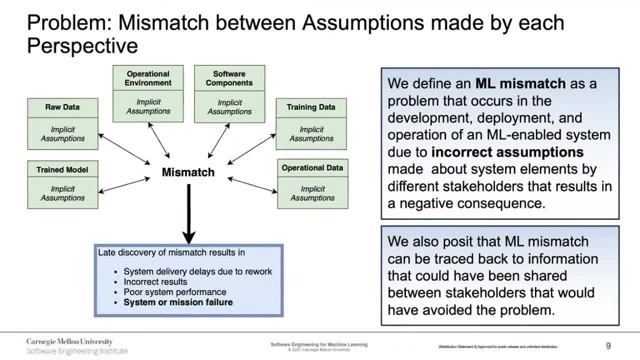 and three different perspectives, And the problem with this is that, because these teams often don't work together and sometimes often don't communicate, they tend to make incorrect assumptions about other parts of the system, And we call these implicit assumptions. So, as a data scientist, 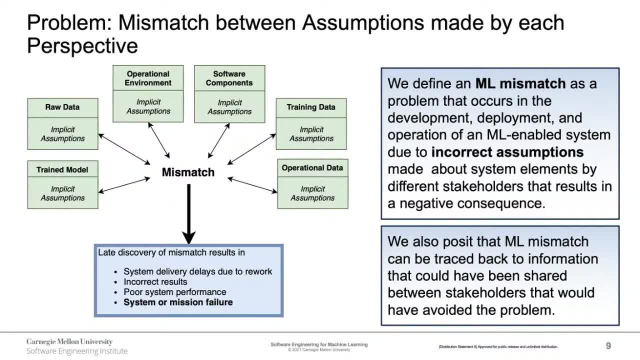 I could make a very wrong assumption about the environment in which the model is going to execute. As a software engineer, I can make a completely wrong assumption about the language that the model was developed in. So this is what we mean by mismatch. So we define mismatch as a problem that occurs. 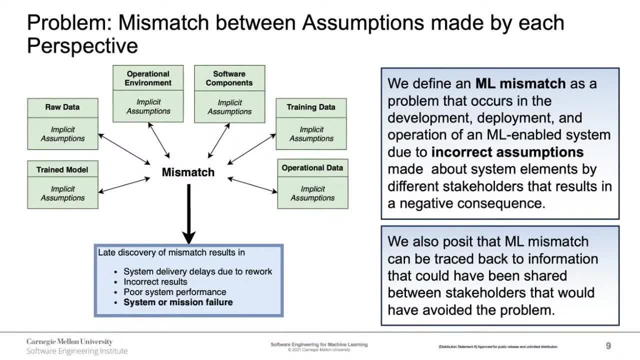 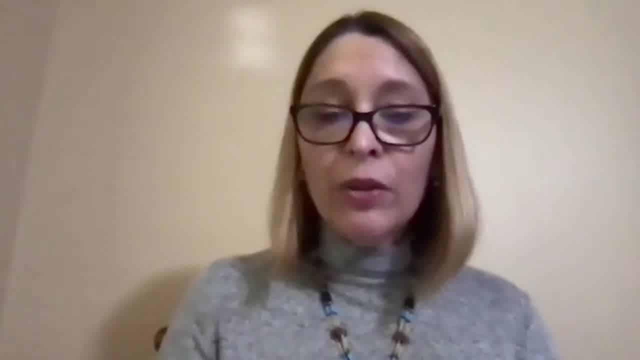 in the development, deployment and operations of a machine learning system, And that problem happened because of incorrect assumptions that different stakeholders made about different parts of the system, and that resulted in a negative consequence In addition to that, in addition to that, 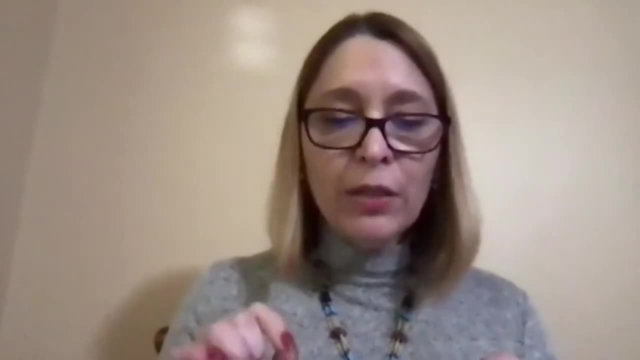 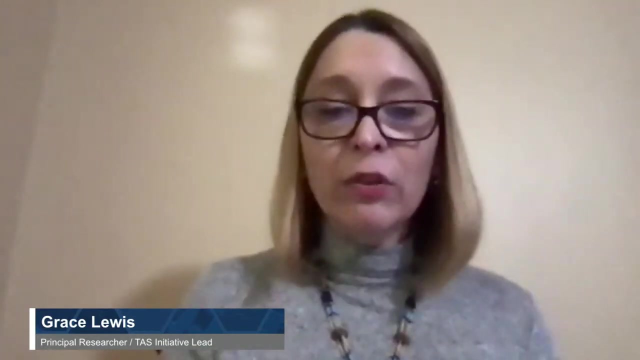 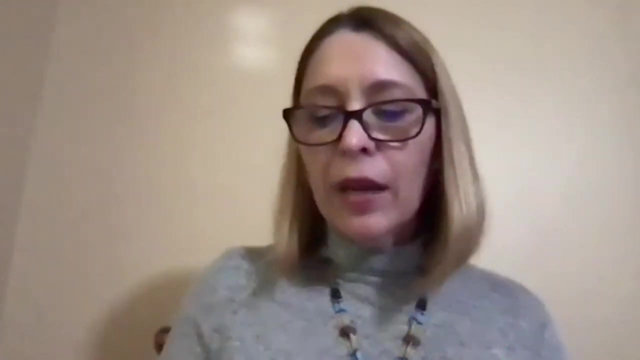 we also posit that ML mismatch can be traced to. there should have been a piece of information that should have been communicated and was not, And if that piece of information would have been shared, that problem would have been avoided. So what are some examples of mismatch? just to get some clarity. 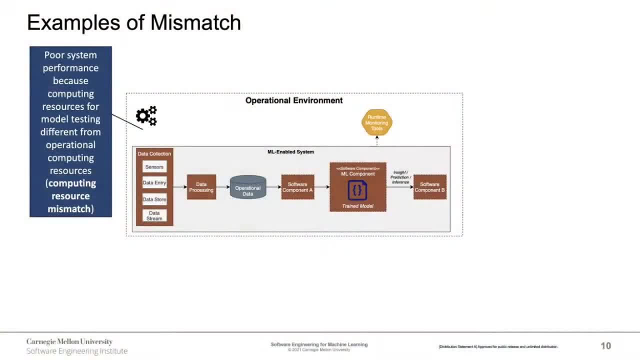 about what we mean. So, for example, there could be a computing resource mismatch, So the poor system performance, because the computing resources that were used, for example, for model testing, were very different from the computing resources available in the operational environment. Or you can have a data distribution mismatch. 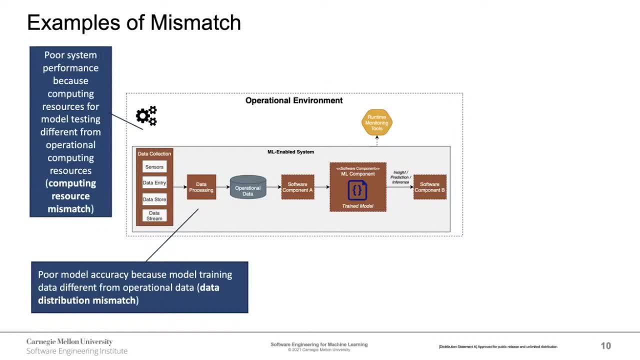 which is actually very common, which is that you have poor model accuracy because the training data really doesn't match the operational data, Or you can have an API mismatch where you have to generate a ton of blue code because the machine learning component is expecting completely different inputs and outputs. 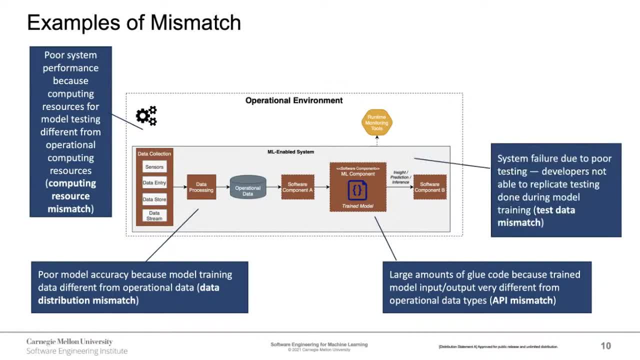 than what is provided by the system in which it's going to be integrated, Or you can have test data mismatch, which is, you know, what the software engineers really couldn't. are they going to be able to do this? They're not going to be able to do this. 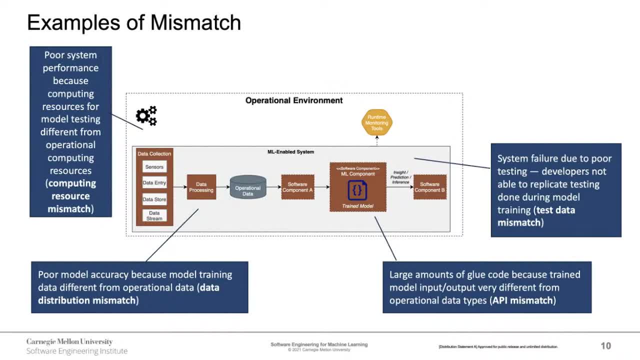 They're not going to be able to properly test the component because they have no idea how to do it, Or there could be a monitoring mismatch, which is basically, or a metric mismatch, which is sure. we have tools for monitoring in the operational environment. 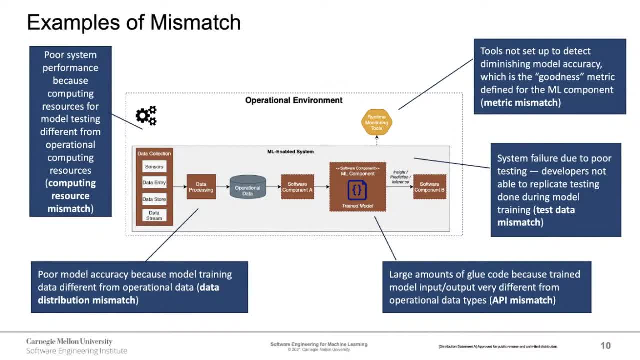 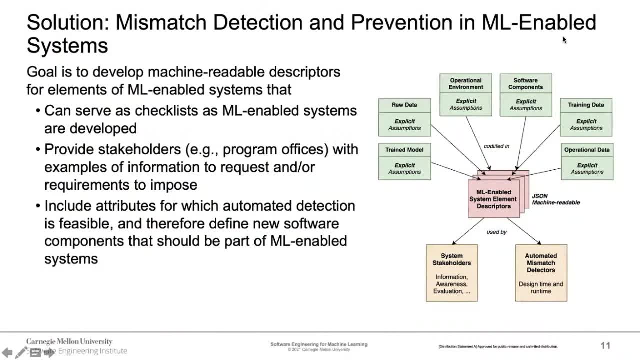 but they're not really capable of measuring that, whatever that goodness metric is for the machine learning component, which is typically accuracy, for example. So what is it that we developed in the context of this research project? So we developed a set of machine readable descriptors. 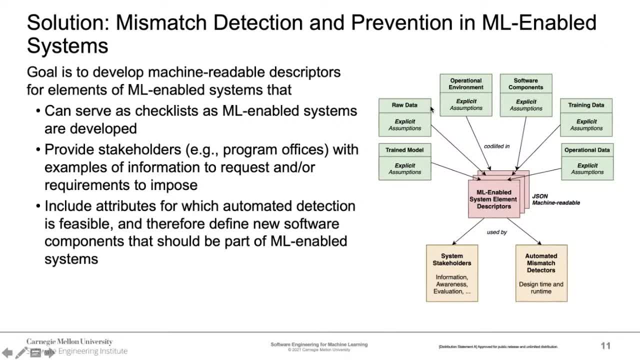 for elements of machine learning enabled systems. So, basically, we developed descriptors for the different elements that you see here in green And they're machine readable. and you'll see why in a second. And why did we create this? So, first of all, we want them to serve as checklists. 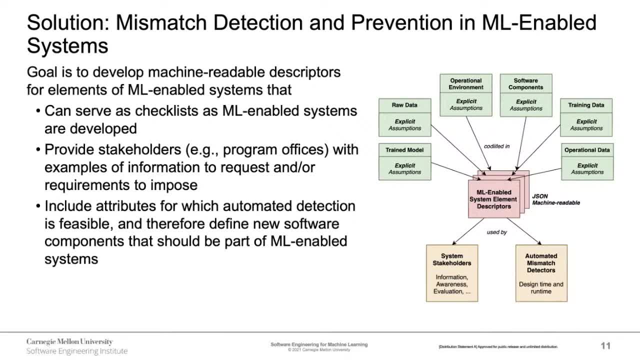 So, for example, let's say that two different teams or three different teams are part of the machine learning system development. You can imagine, for example, that the data science team would create the descriptors, for example, for the train model and the training data. 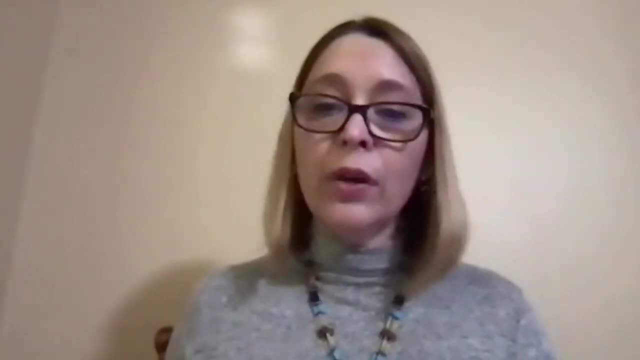 It could be that the operations people- because the raw data is coming from the operations environment- provide the descriptors for the raw data. The software engineers provide the descriptor for the development environment. But basically these serve as checklists. So, for example, when a model 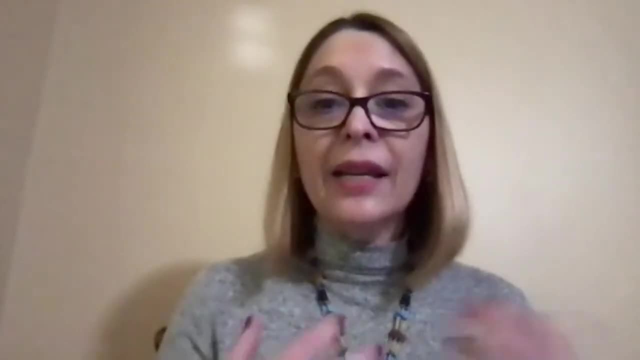 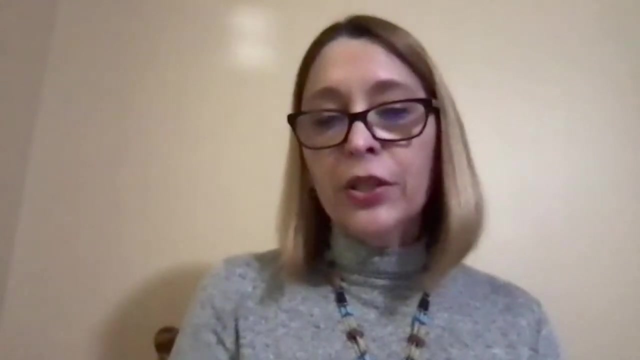 when a train model is handed off, we can make sure that all the information that I need in order to avoid mismatch has been included. Similarly, it can provide stakeholders with examples of information to request and or requirements to impose. So, for example, if I'm an organization. 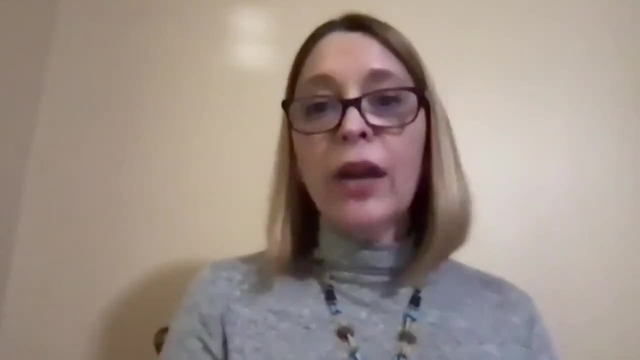 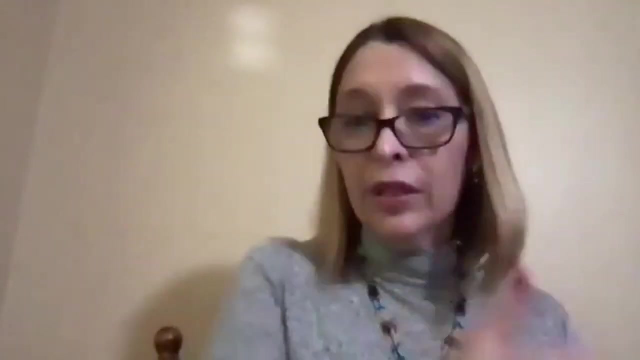 this is very typical in the Department of Defense, where I have contractors, for example, developing models. I can say: yeah, when you deliver your model, make sure you also accompany it with these particular descriptors. And the third one, which is the one 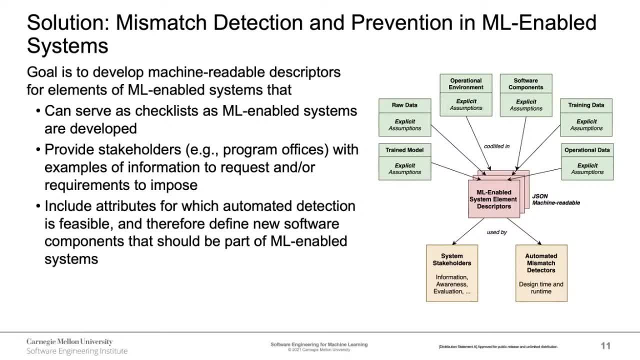 that we're very excited about and hopefully we can continue working on that, which is what we want, is that we want these descriptors, we want them to be able to be leveraged by tools that can do automated mismatch checking to make sure that everything is in agreement. 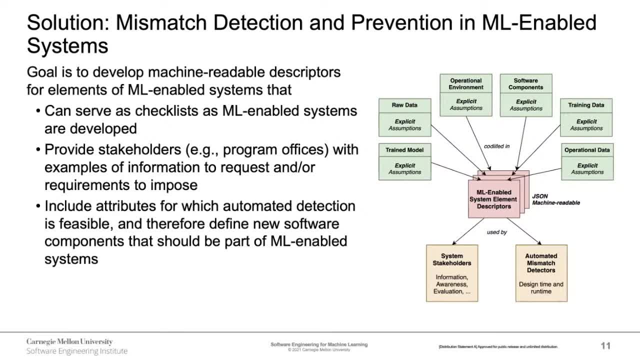 And the reason also why that is important is because if we want to be able to detect mismatch, for example, at runtime, it also dictates different system elements that also need to be present in order to do mismatch detection. So, as seen in the diagram on the right, 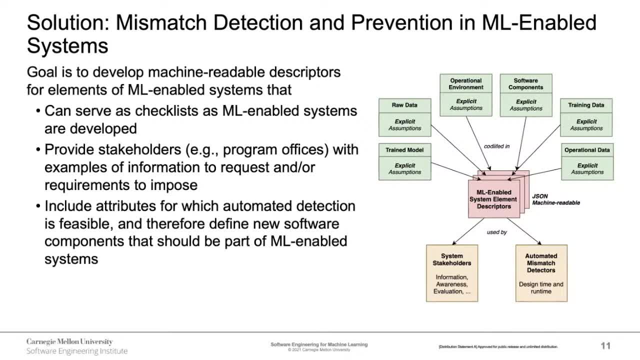 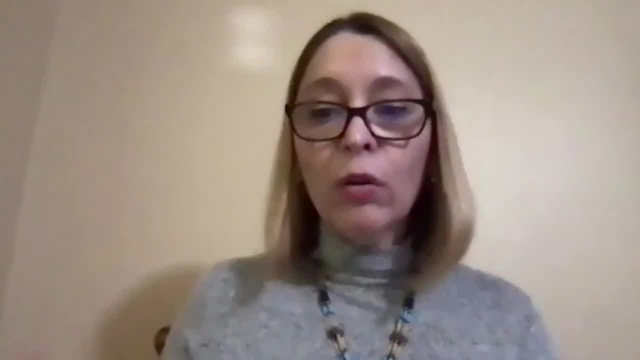 we expect them to be used by system stakeholders, let's say, in a manual way, for lack of a better word, so just for information, awareness or for evaluation or things like that. But we definitely also. the end goal is automation. We want to be able to use these descriptors and tools. 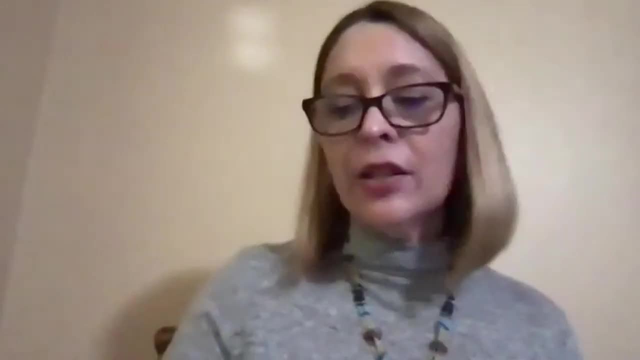 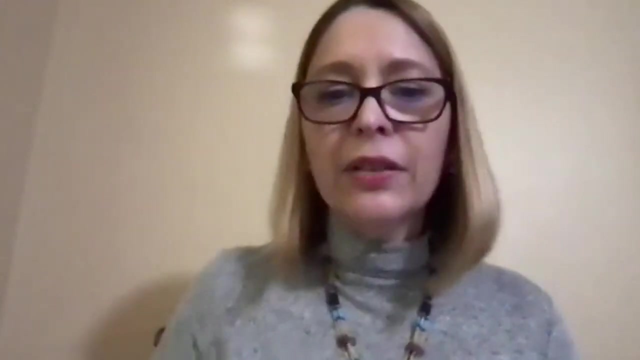 that can, at design time and runtime, say hey, there's a problem here, there's a mismatch. I see that there are questions. Ipek, go ahead before I go into the study. I think this is a very good time. 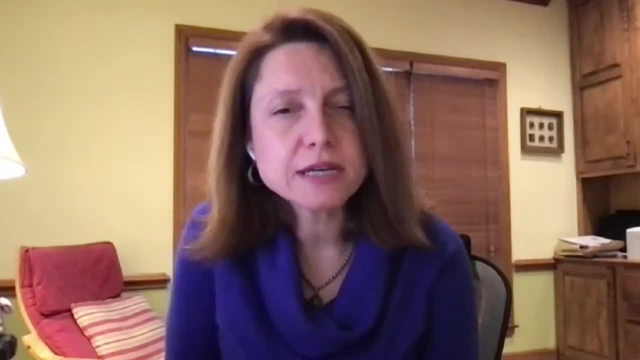 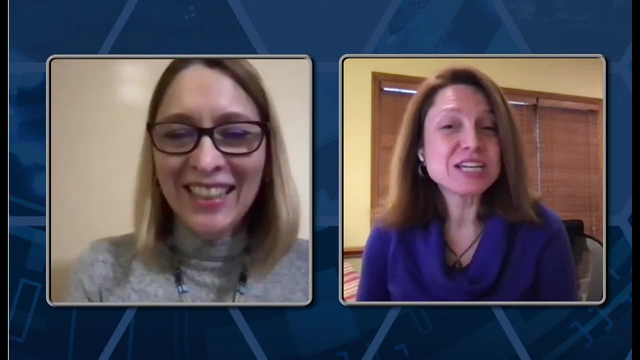 Yes, so there's actually a question from Matt. I will take them in different orders because I know about the study and what you'll talk about. I'll take advantage of it. The question is: can you give a very quick overview of the types of systems, organizations and environments? 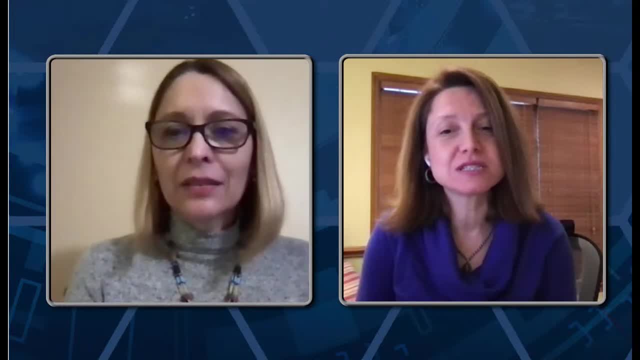 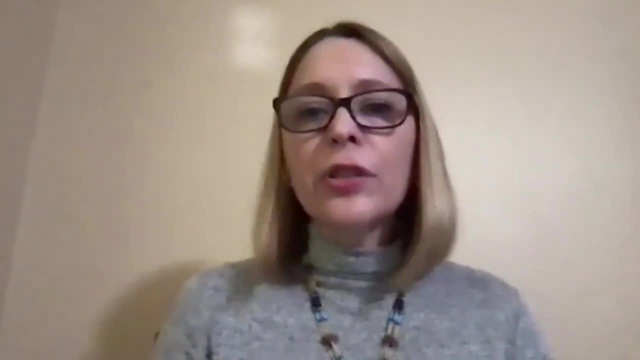 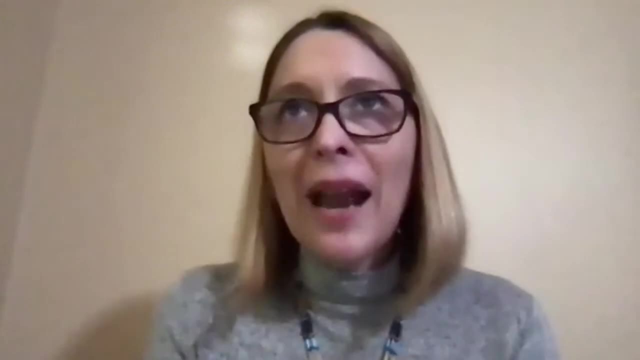 that was included in the study and, in particular, did that include systems that followed CI-CD pipelines and lifecycle? Yeah, so unfortunately there's not a lot of because of the IRB. I can't report on specific systems, obviously, but I would say that we had a good representation. 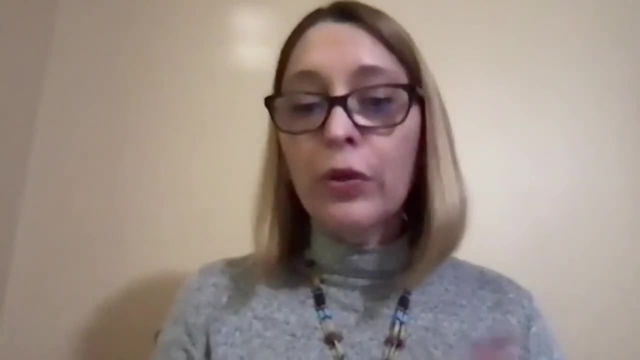 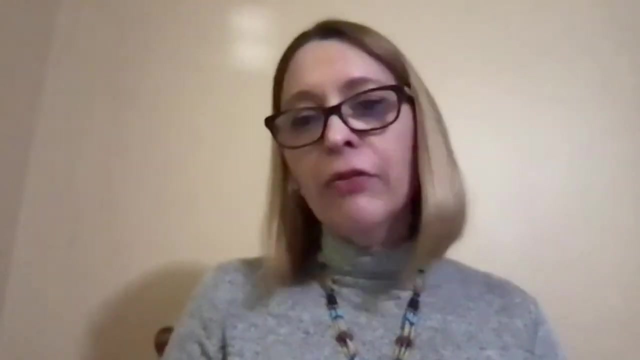 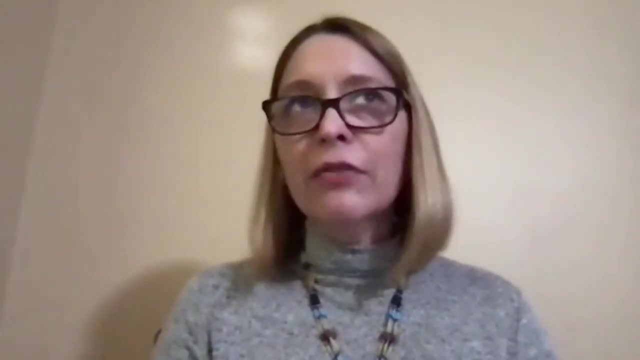 I'm going to talk about that in the study. We had good representation from industry, both large industry as well as small, basically startups. We had also a very good representation from Department of Defense, both the government and contractors, And I would say very, very different. 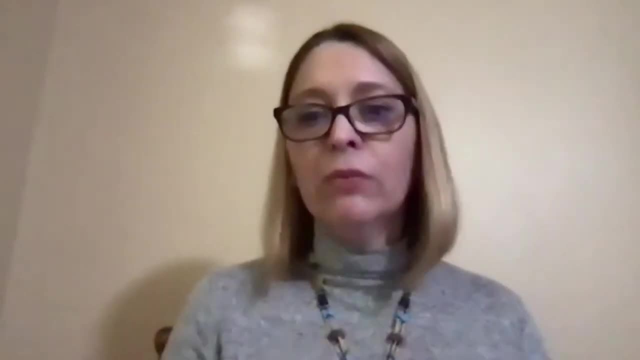 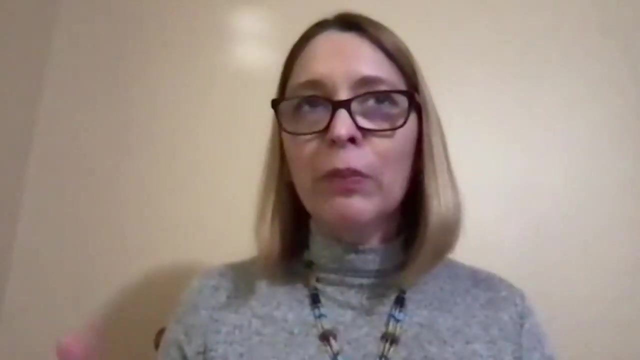 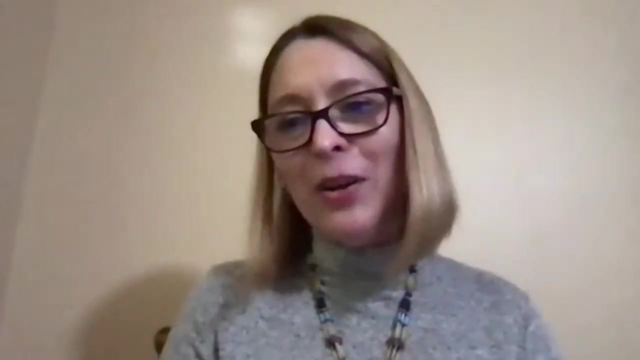 types of systems, going from very massive systems, like we interviewed people, for example, from the large industries- I'm sure you can imagine what those are- But, for example, we also interviewed people from startups, where their product is one system but that system has to perform very well. 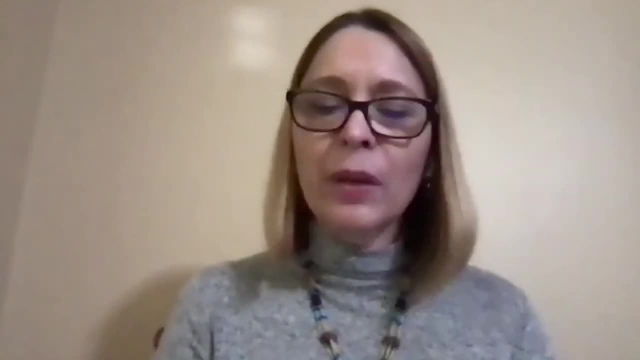 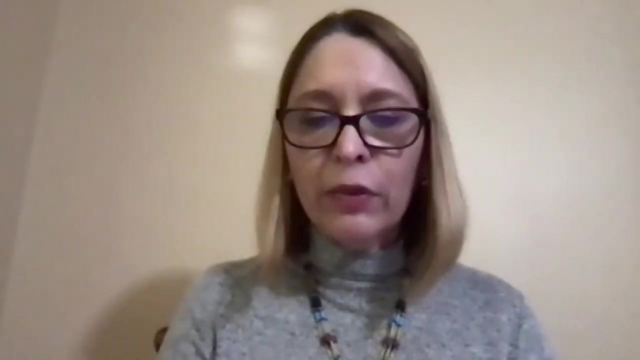 There was also representation from the larger companies that tend to be the ones that have more automated processes- and actually the second project is going to talk a little bit about this- where, for example, models are trained on a daily basis just because they can. And or, for example, there were also small companies where models are really retrained, for example, and don't really require it because it's just like one product. you know what I mean. They don't have very complex CI-CD pipeline. 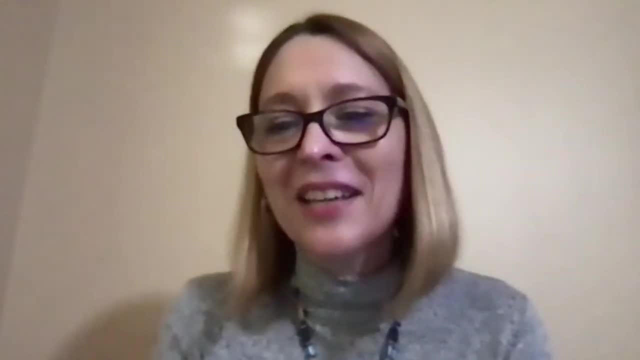 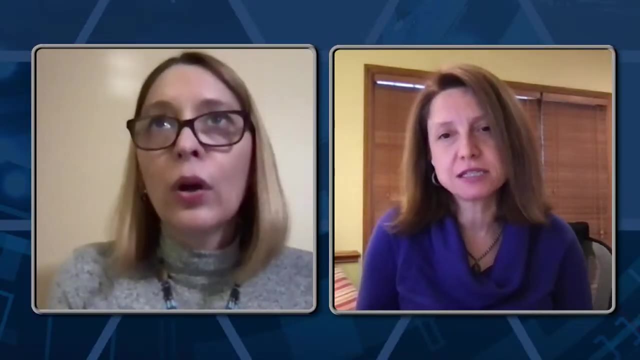 But I want to save some of that for when I talk about the study. But all of them were organizations following modern software engineering practices, up-to-date tooling, CI-CD lifecycle and awareness of all those. So I think that's common Right. 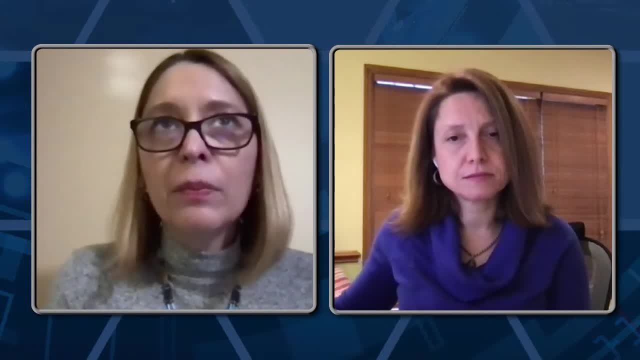 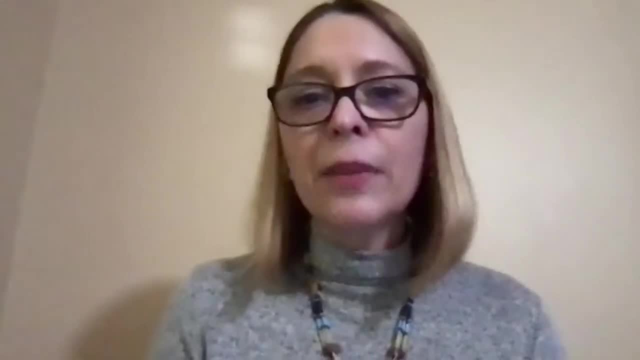 I think that's common across Correct, And also both for the interviews as well as the survey. one of the requirements to participate in both is that you had to be part of organization that was developing systems that fit into our definition of ML-enabled systems. 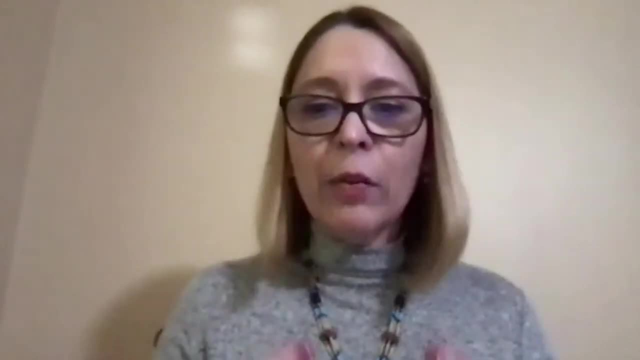 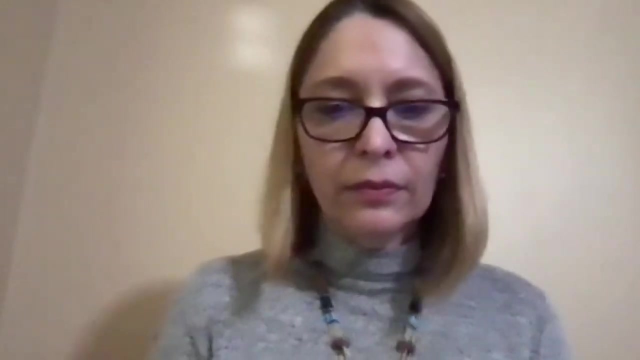 They had to be a part of a team, of a group, of an organization that was developing those types of systems in which the components are part of a much larger system. And I'll tell you the next question, but you might maybe prefer to answer it while you get there. 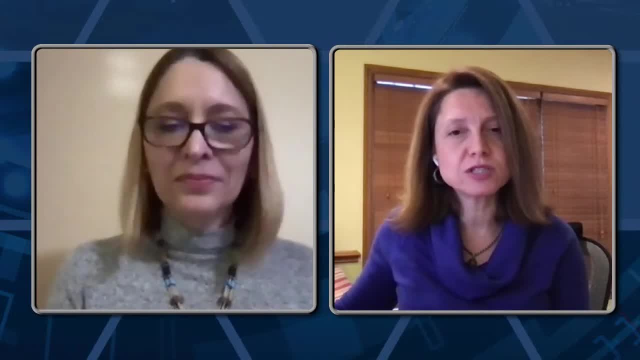 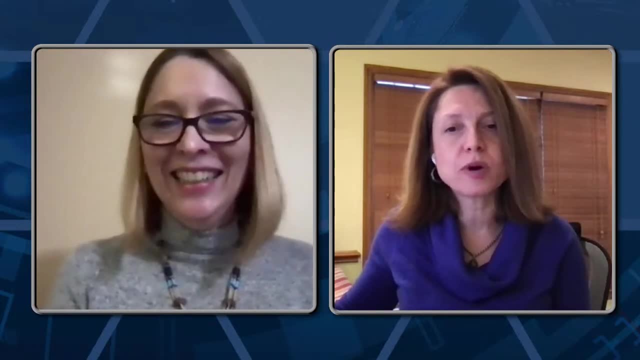 because we do talk about programming languages and their mismatches. So the question is from Dwayne and he asks: is R an absolute necessity for hardcore ML or can standardizing on Python improve ML mismatch? So thanks, Oh my gosh, you can answer now. 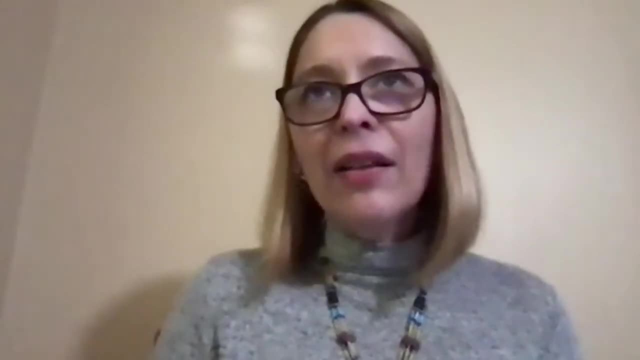 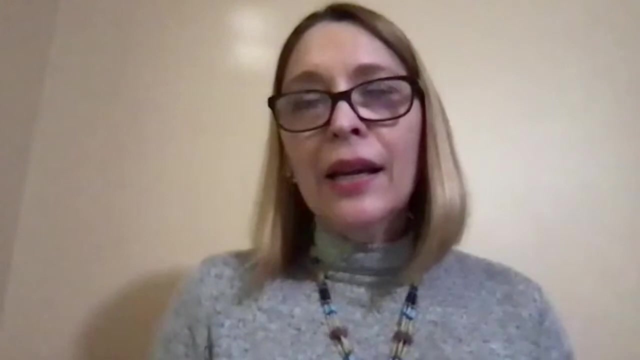 or you can answer when you get there. but I wanted to chime in on this. I'll answer when I get there. but you know what? that is such an it-depends question and I hate to give those answers, but really it depends on skill. 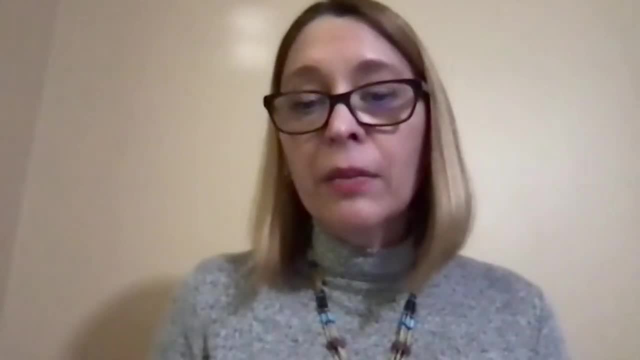 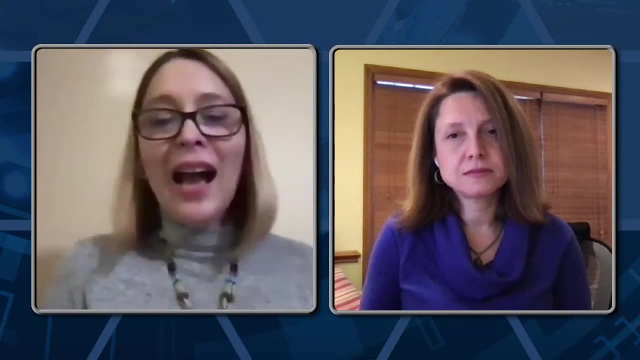 Now, from a robustness perspective, I will say that Python is a much more robust language And if it were my preferences, that's probably what I would do. But R, from a statistics perspective, is a lot more. I would say it's a lot more complete in terms of libraries. 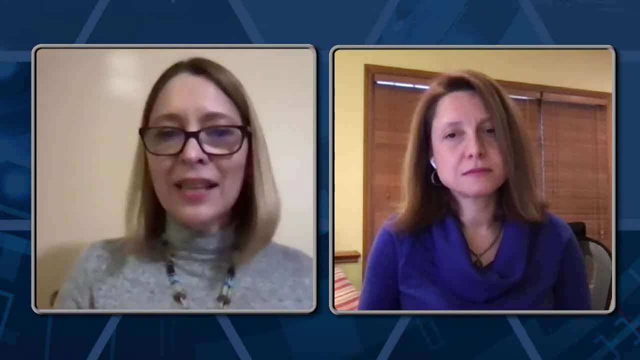 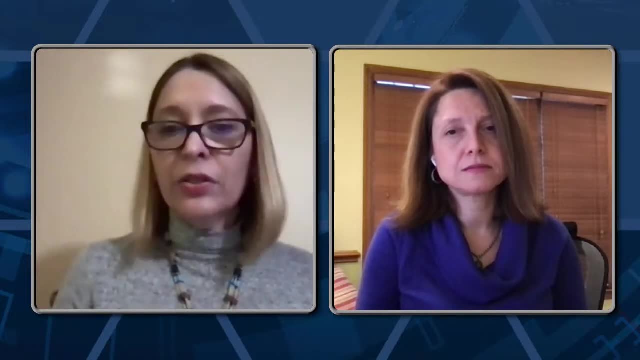 so it's kind of one of those I don't know. it's one of those, like I said, it-depends questions. However, and even though I'm going to talk about this, there were so many mismatches that we had in the study. 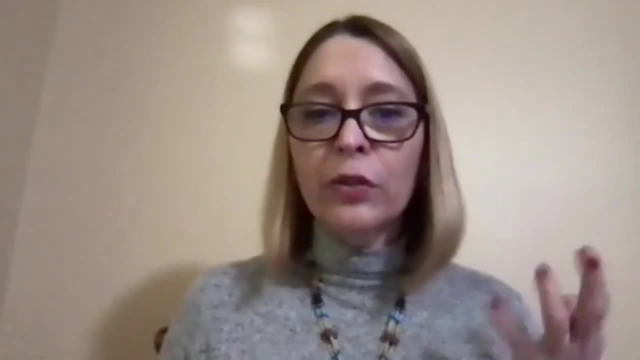 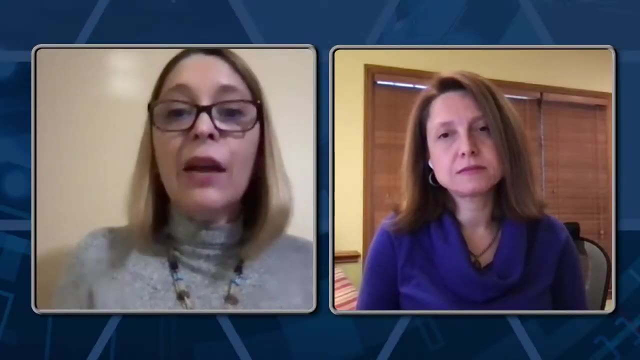 related to supporting problems, and you'll see why in a second. So, for example, if you have data scientists develop a model in R and then it's just handed over to the software engineers and now they have to reimplement it in Python. 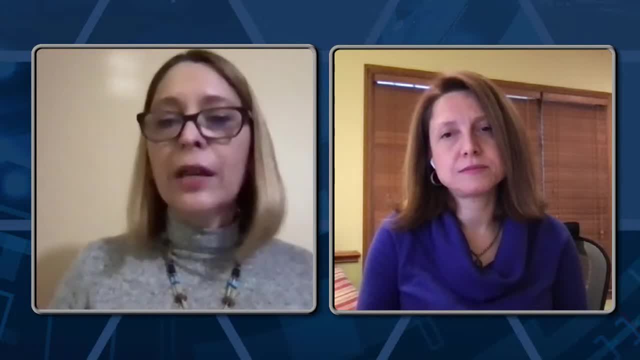 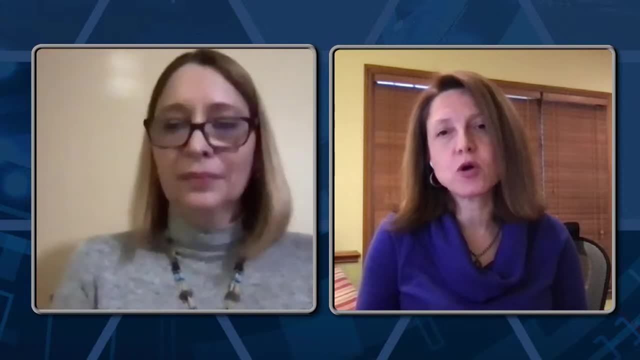 there's so much room for error. So we definitely did see mismatches such as that, And programming language is definitely that's where the devil is, in the details and that's where you actually get all the system problems, and so we saw some of those as well. 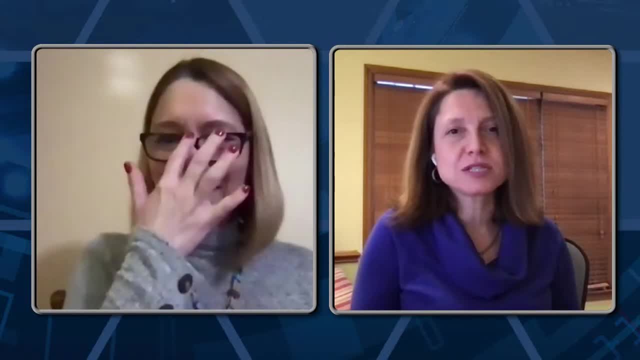 So I won't- Correct Drill you any further and we'll get to some of that. Okay, We'll get to some of these conversations as you explain more about our data. Absolutely, Thank you for the questions. I really appreciate it. 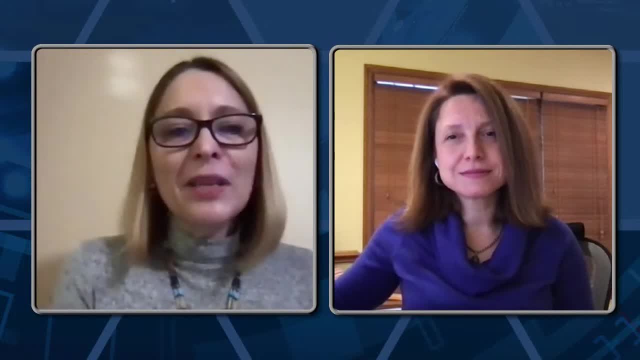 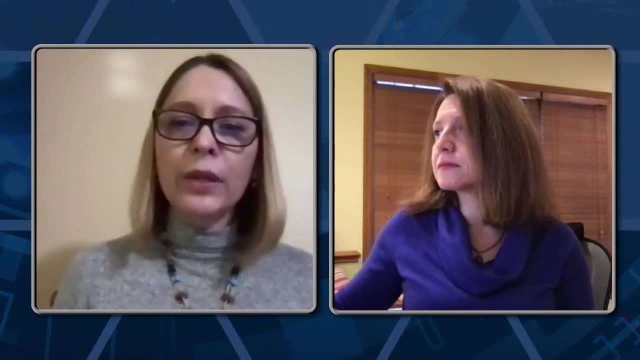 It's so much it's good to have like those little breaks. So now this. let me talk a little bit about the study protocol that we followed. We divided the study into two phases. In phase one, what we did was that in parallel, 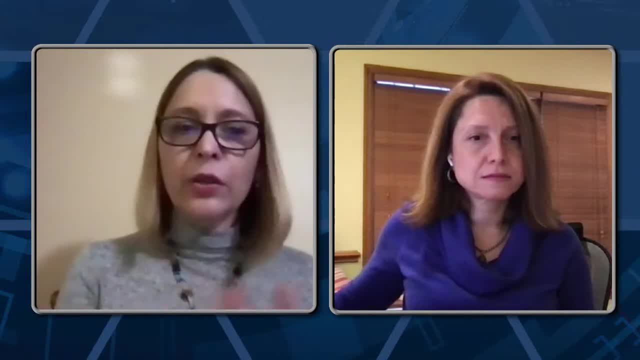 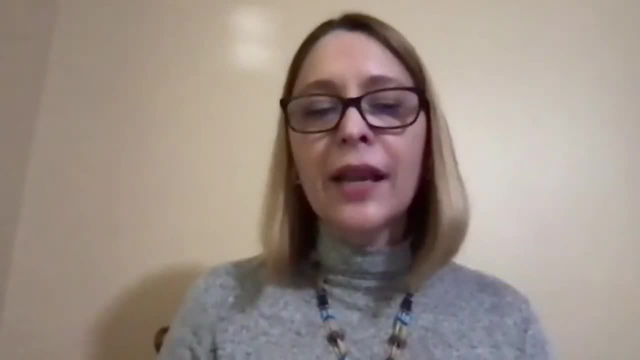 we conducted a set of practitioner interviews. I already told you what type of practitioners these were, And the goal of those interviews was to elicit mismatches and consequences. So basically, it was asking the same question over and over again is: can you tell us an example of a mismatch that occurred? 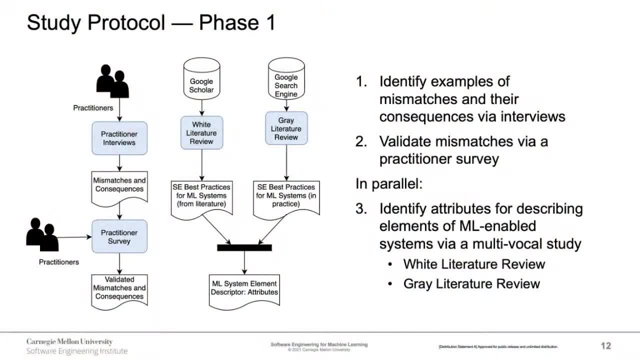 because you made an incorrect assumption, or somebody that you worked with also, or made an incorrect assumption, And we gathered a series of mismatches and consequences. I'll show those in a second. And then we followed that with a practitioner survey where we basically said: 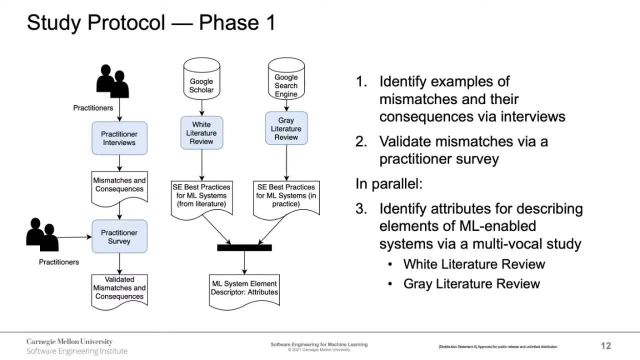 how important do you think it is for you to know this information in order to avoid mismatch, And so definitely out of that survey came instead of validated mismatches and consequences, and I'll show you some of the results in that. In parallel, we conducted a multivocal literature review. 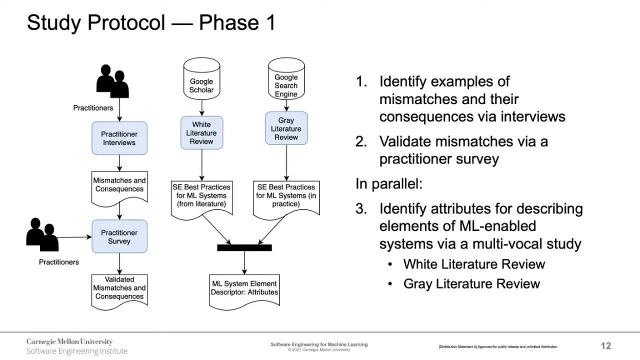 combining both white literature and gray literature, where we basically mined these literature, this literature, for best practices for ML systems, particularly looking at pointers to like this is how you should document systems: this is information that needs to be shared, So really mining them for best practices. 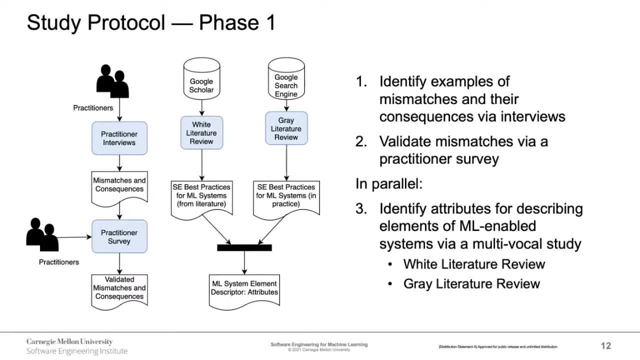 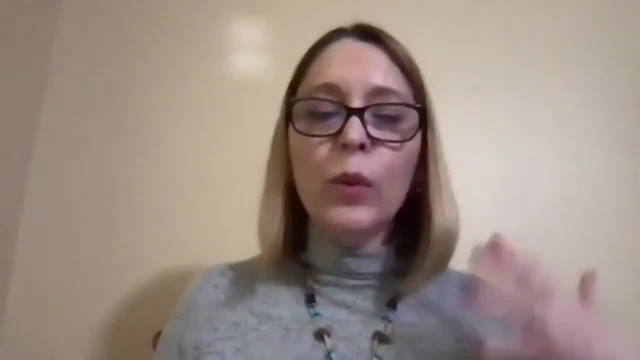 in terms of information sharing, And out of that came what we're calling system attributes. and you'll see that in a second Phase, two of the study consisted of: okay, we have a set of validated mismatches and consequences, We have those system element descriptors in attributes. 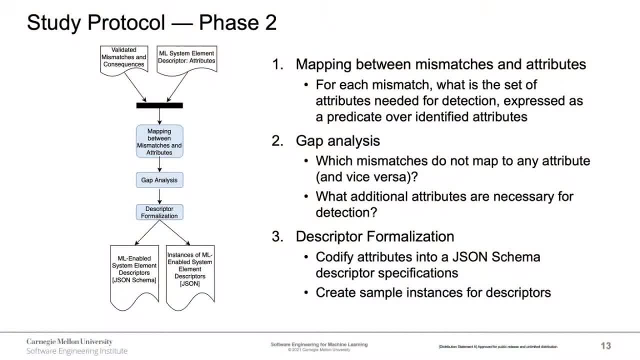 Now let's do a mapping between the two, Which are the system elements that I would need to know in order to avoid this particular mismatch, and do that mapping. And then we did a gap analysis where we basically said, okay, sorry, I'm doing this. 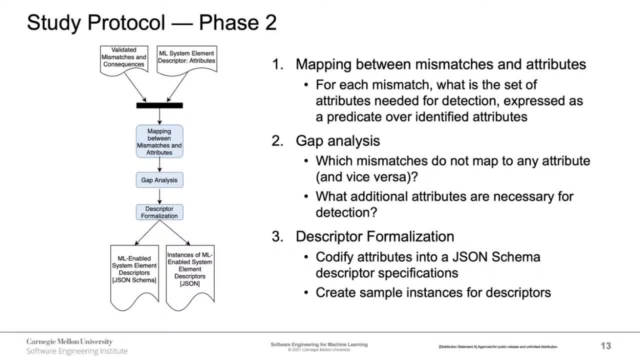 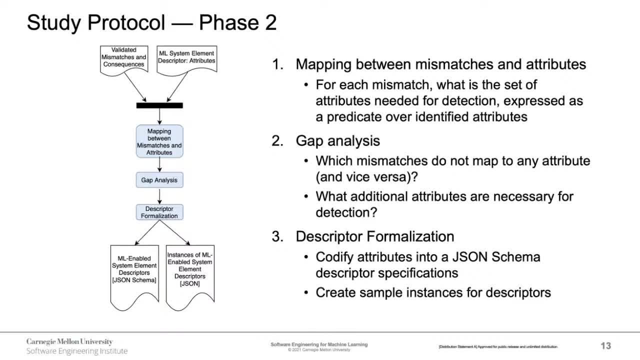 that there are no system attributes that could be able to detect that particular mismatch, And the other way around are there attributes that came up as best practices but don't really map to any mismatches, And so what we did is based on our knowledge. 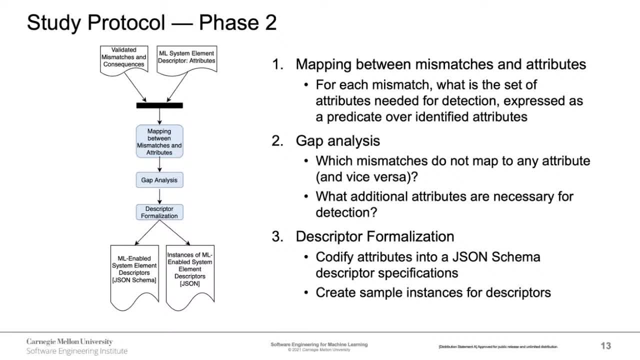 and in addition to other literature that we reviewed, we said, okay, let's fill in these gaps. And then, basically, we created a set of descriptors, a set of seven descriptors that we defined in JSON schema, just because, as I said before, our end goal, 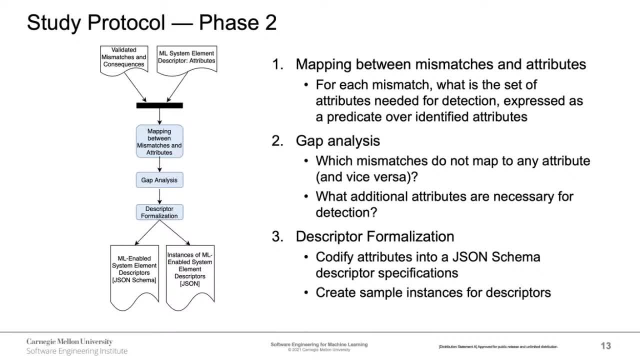 just because, as I said before, our end goal, just because, as I said before our end goal- is really automation. So what I'm going to report on today is that this, only this, only this part, and hopefully in the next. 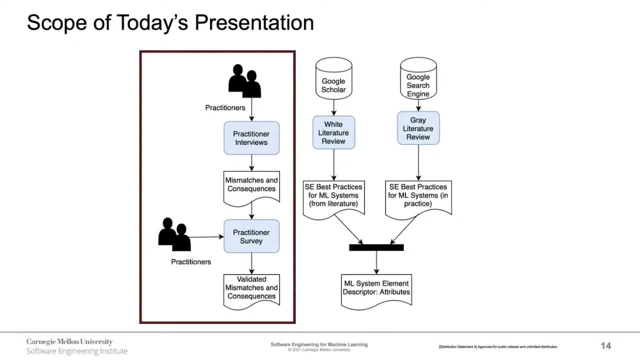 hopefully in a follow-up webinar I'll get to talk about the other phases, But we're going to talk simply about the phase one: the mis- and the elicitation of mismatches and consequences, and what we are seeing are the main causes for mismatches. 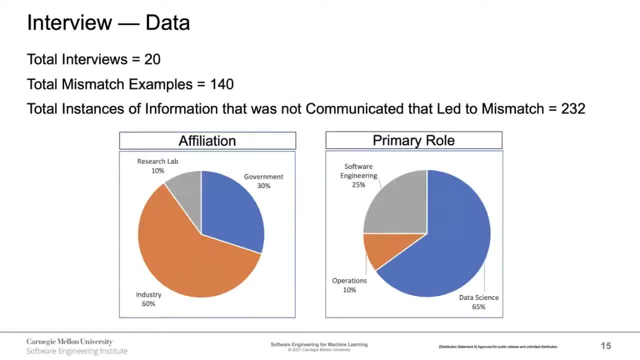 at least among the people that we interviewed and surveyed. So, as far as interviews, we conducted a total of 20 interviews and those from those 20 interviews we did very, we followed very, very sound practices and we came up with a total of 140 mismatches. 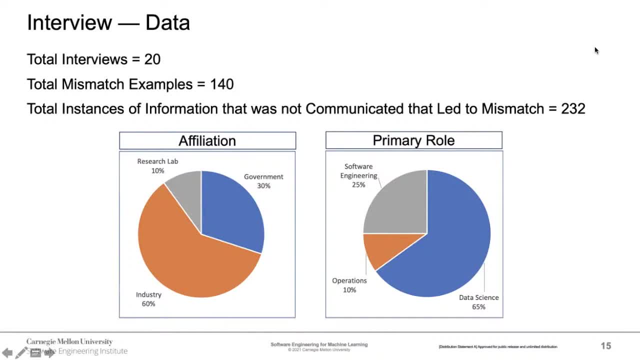 that led to 232 distinct examples of information that was not communicated. that led to mismatch. This goes back to the question that was asked earlier as far as affiliation- 60% industry, 30% government, 10% research lab and primary role- mostly data scientists. 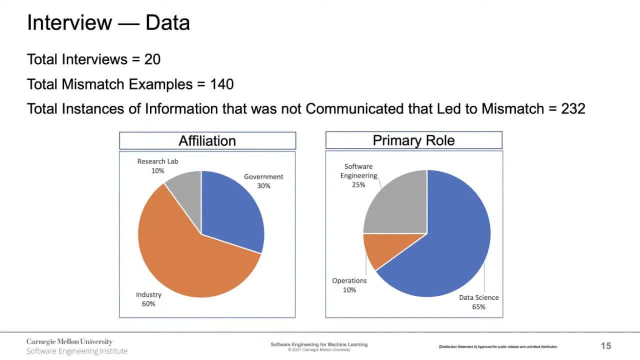 and actually this is some in full disclosure. this is one of- we believe this is one of- the threats to validity that is very data science heavy, which is why we want to repeat this study. we would like to repeat the study with a more distributed and a better distribution of people. 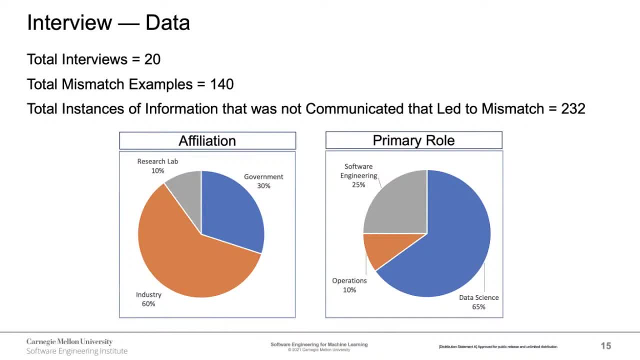 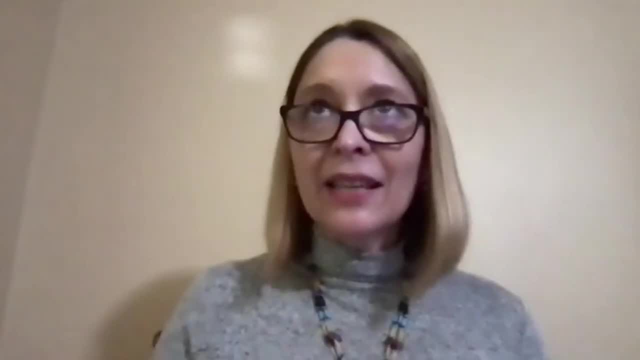 especially so we can get more of the operations perspective. That said, it was very hard to get people in the operations role. It's again a lot of people are, which shows that a lot of people are still kind of in the model development phase. 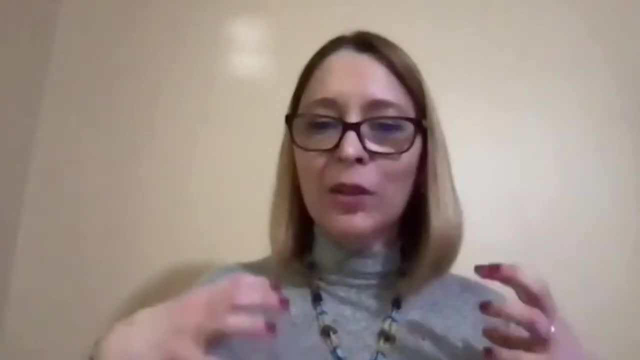 and they're really having gotten done a lot of research and they're really having gotten done a lot of research into that operations phase where they're monitoring a machine learning system and doing those things. So, yes, it's a problem with the data. 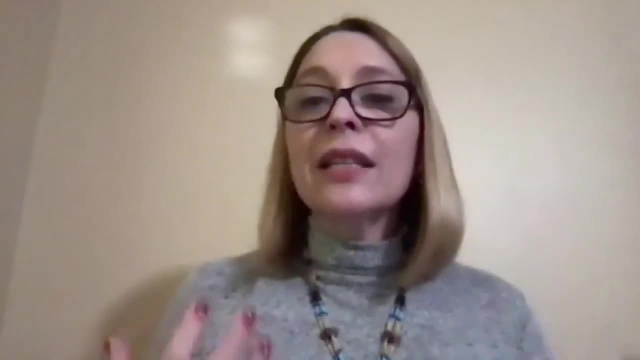 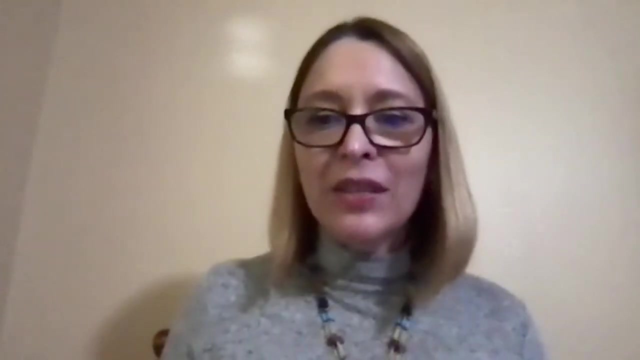 but also it was simply. it's almost like it's not a known thing, not a known thing, but how would I say this? It's operations. people are not typically associated in the type of development of these systems, which we think is a problem. 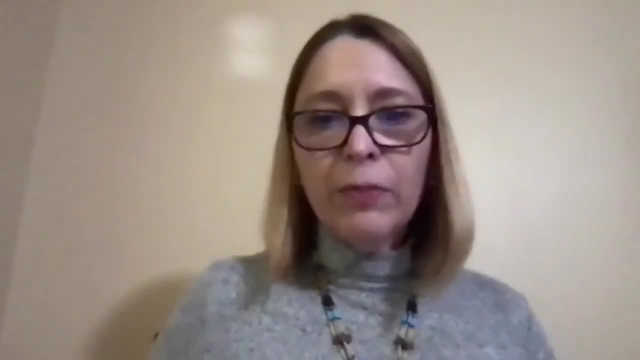 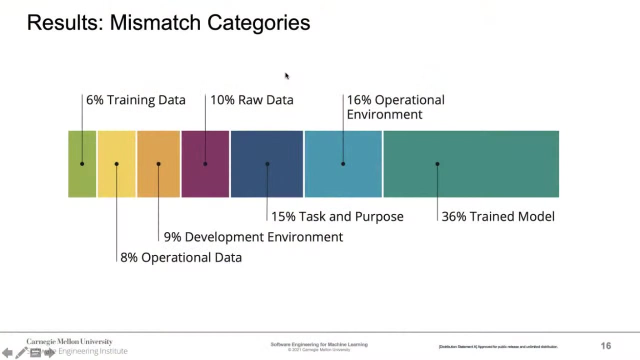 So basically, when we took all those examples of mismatch, what it came down to was this chart that you're seeing right here. So 30% of the elicited mismatches had to do with incorrect assumptions about the trade model, followed by 16% that incorrect assumptions. 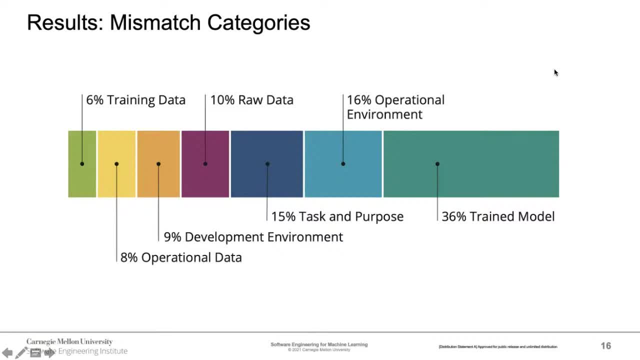 about the operational environment, 50% about task and purpose and the others in smaller amounts, And what I'm going to do is I'm going to go into detail into one of these and for each one of these, I'm going to give you a breakdown. 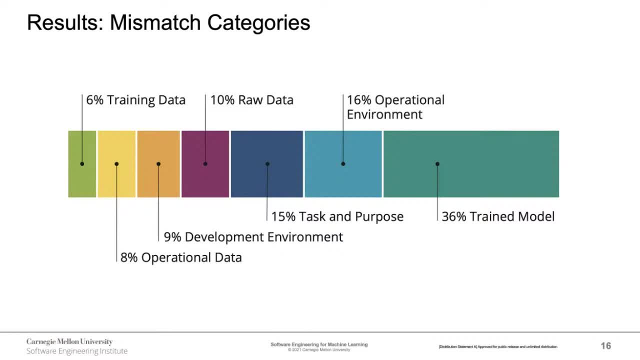 of what were the sub-categories and also give you an example of a quote from one of these, and also give you an example of a quote from one of these, and also give you an example of a quote from one of these, And I'm going to go into detail. 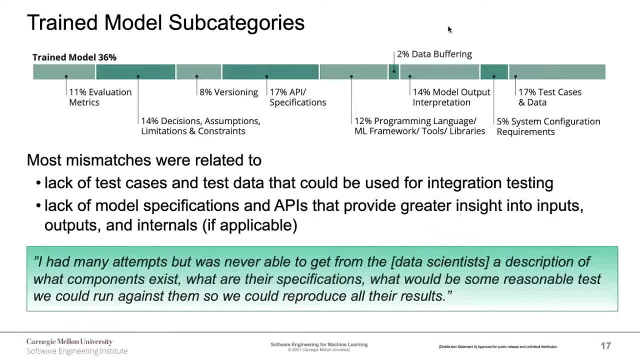 into the interviews that I'm sure that many of you will be able to relate to, because we definitely were able to relate to it. So, as far as training model, it was an even split between test cases and lack of test case. information related to test cases and test data. 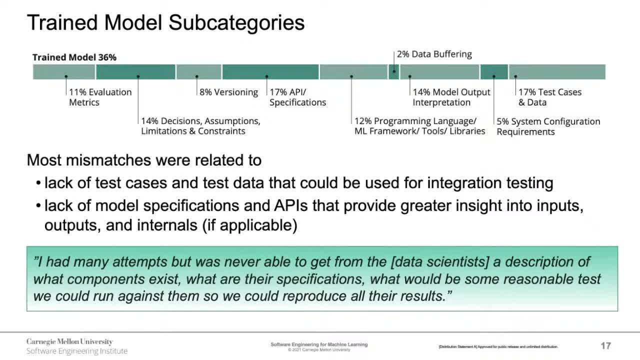 and lack of information about API and specifications. that led to the most mismatched examples. So this example comes from a person in the software engineering role that basically said: look, I was really never able to get from the data scientist a description of what the components were. 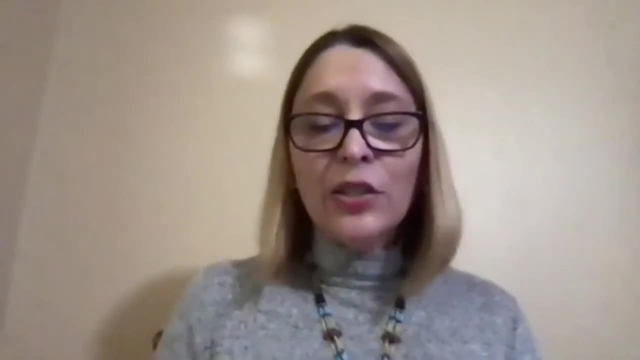 what were their specifications? were there any tests and so we could reproduce the results? So this was a typical example where, again, a model is kind of like. I mean, it's an idiom, but kind of thrown over the fence. 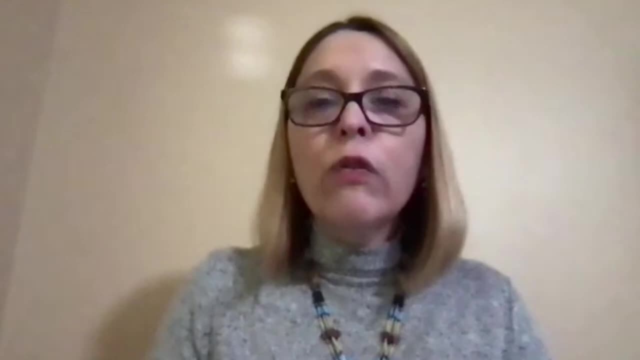 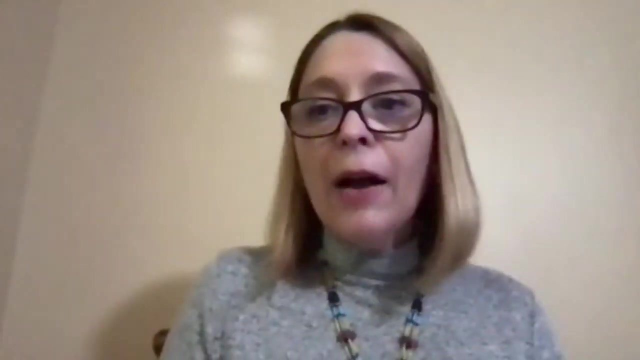 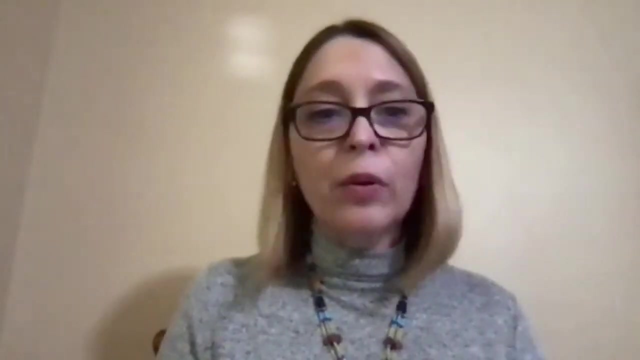 and it's like: okay, integrated into the system and there is no formal specification or even informal specification of that model. that would help me integrate that model into the system. Other examples of subcategories included, for example, lack of evaluation metrics, for example. 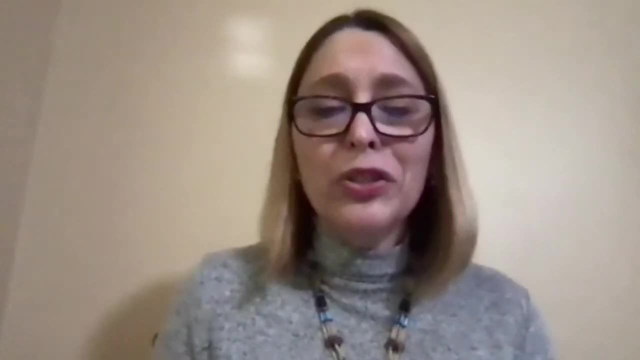 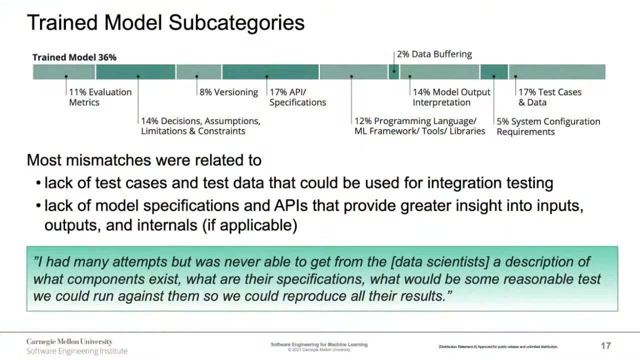 the operations. people put the model into production, but they weren't sure exactly what it was that we're supposed to be monitoring: Programming languages. this is exactly the example that I talked about before. that, for example, the software engineers had no idea. 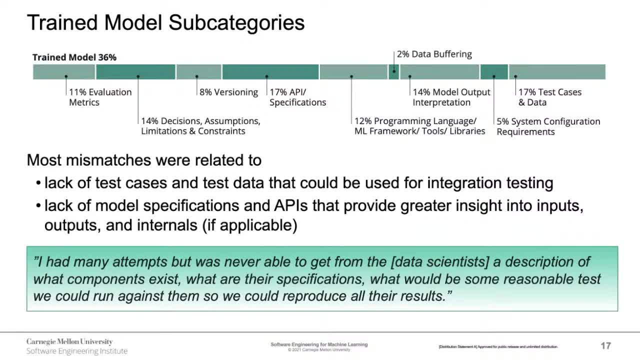 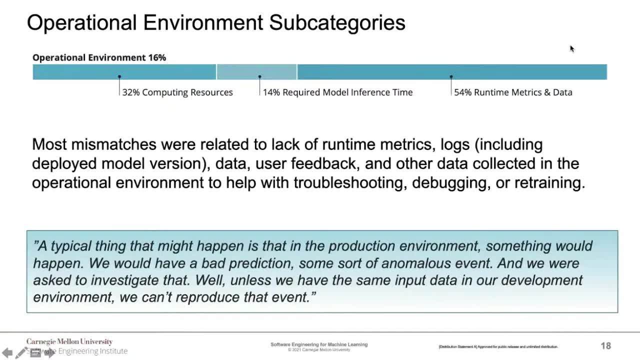 that the model was gonna come in R and that totally messed up their schedule. So, yep, those are some of the subcategories under train model. As far as operational events, this was the second highest category. A large number of the mismatches were related. 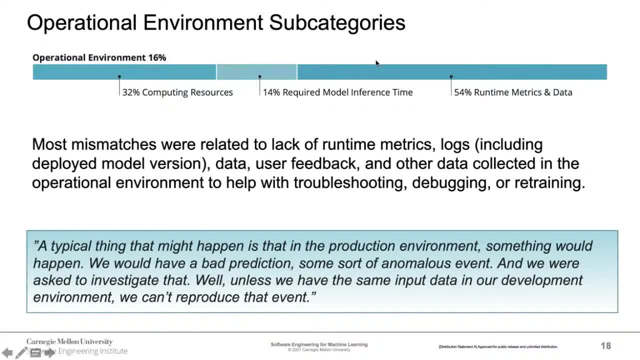 to runtime metrics and data Basically. again, the model was put into operation and either the operations folks had absolutely no idea what it was that they were supposed to be monitoring or the other way around, the data scientists just assumed that this was something that the operations people 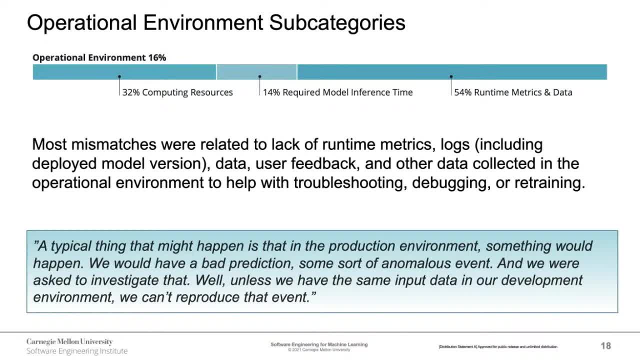 know how to do and they were collecting all this runtime metrics and data that they needed, And so this is a quote that comes from one of the data scientists, from a data scientist where, basically, the models were into production. the model produces a bad prediction. 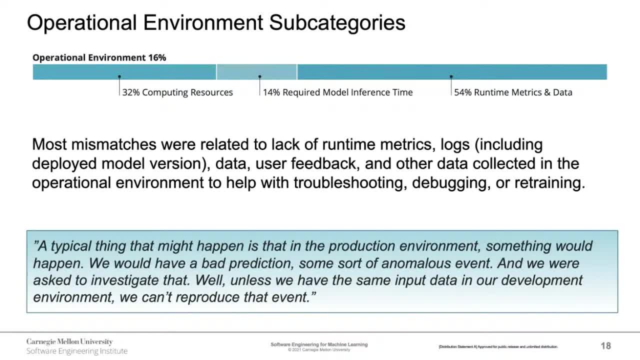 and the. for example, the operations team comes to the data science team and says, hey, the model isn't working. and they're like: okay, can you show us what data you were collecting? where are the logs? and it's like: well, 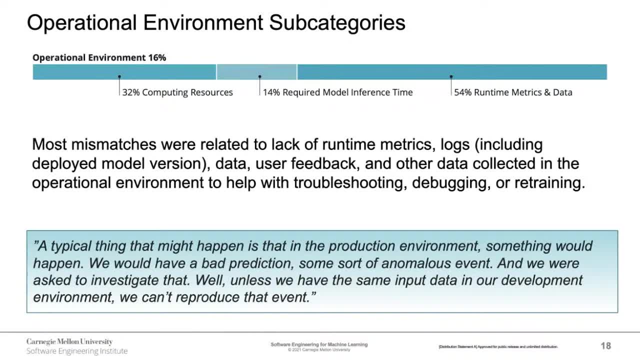 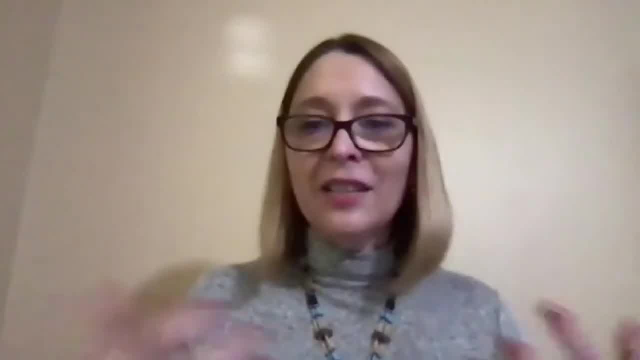 unless you tell us, you give us some more information, we really can't reproduce that event. So it's this idea again, and this is the whole idea about mismatch: if this information was shared, you know, if operations and data scientists were acting, 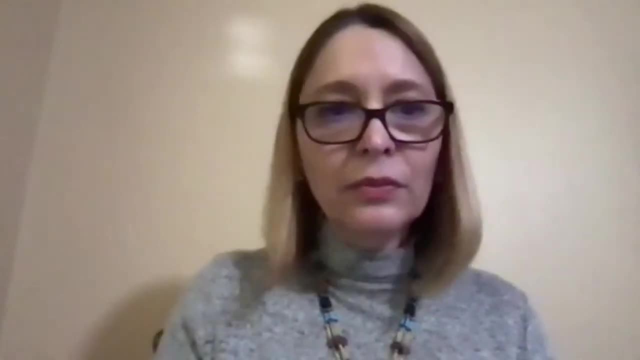 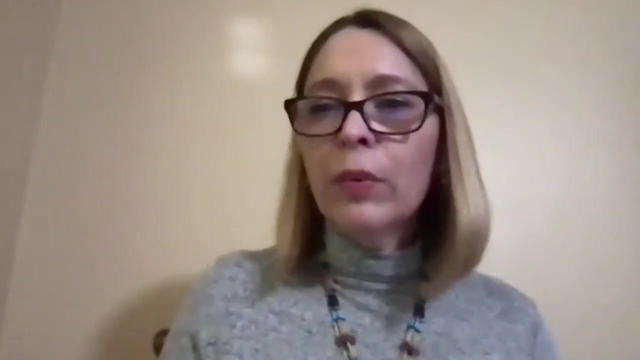 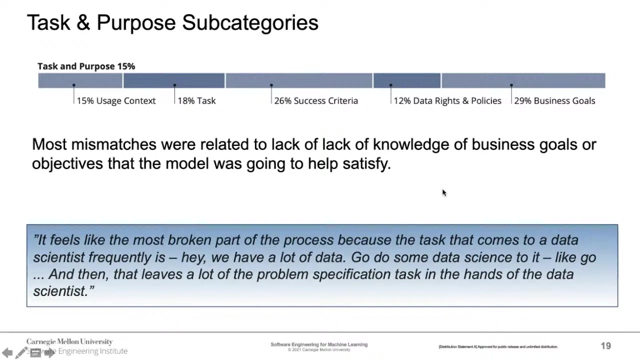 with the same information, this mismatch wouldn't have occurred. Next is task and purpose. This basically a rough way to think about task and purpose is almost like the model requirements. So, basically, what are things that need to be communicated, especially communicated, for example: 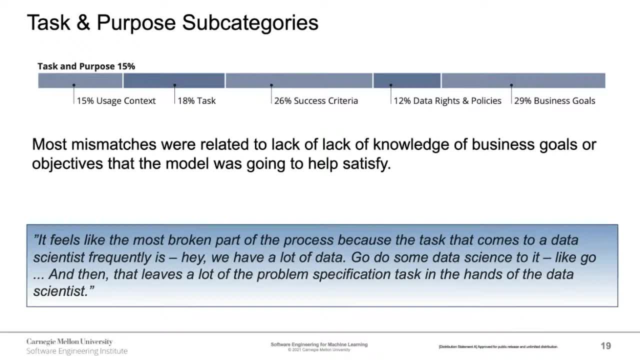 between project owners and data scientists so that data scientists build the right model. So, for example, 29% of mismatches had to do with lack of business goals, and I really love this. I really love this quote. it's a quote that made me laugh a lot. 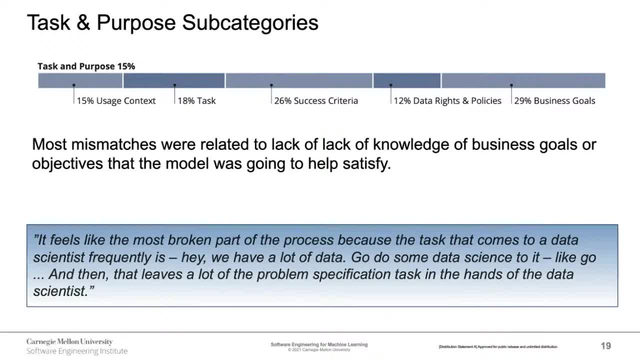 but we heard it. we heard the same quote from many people. it's just that this one, this person, just said it in the right words. this was a data scientist and she said that she felt like the most broken part of the process was exactly this task and purpose. 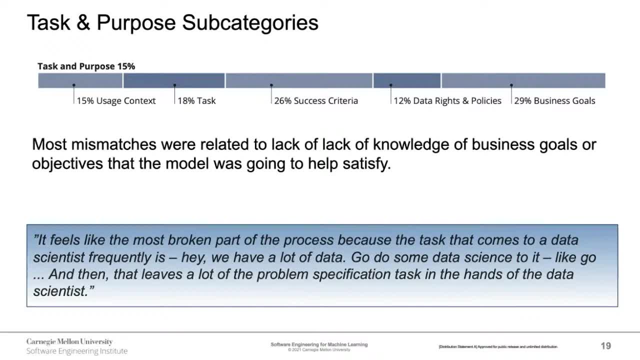 because a lot of the time, you know, somebody comes to a data scientist and says: here, here's a bunch of data, go do some data science on it, and they're like, well, okay, but you know you've got to do it with what purpose. 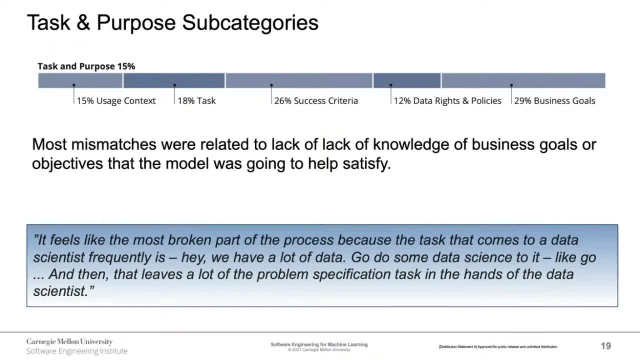 and then what happens is that the specification of the problem is left in the hands of the data scientist, and so there's a lot of churn and a lot of going back and forward. you know, the bring me the rocks in there, right. 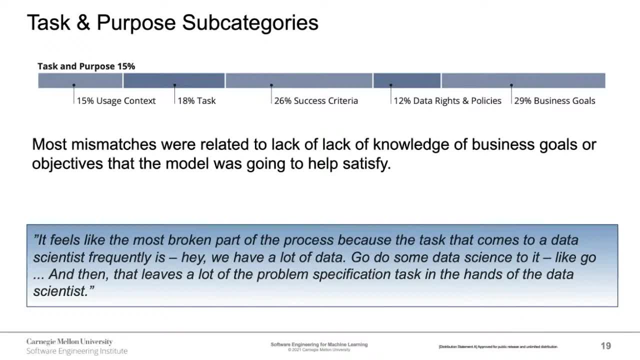 Is this what you want it? No, it's not. Is this what you want it? No, it's not. So there's a lot of going back and forth and again. if this information was explicitly shared from the beginning, we wouldn't have these problems. 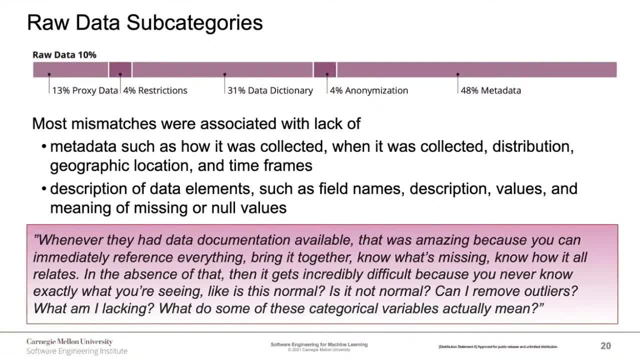 As far as raw data, just to clarify what raw data means. raw data is the raw data, is the data, the data that's used. the raw data it's not the training data, it's the data that. it's the data sets that come as is. 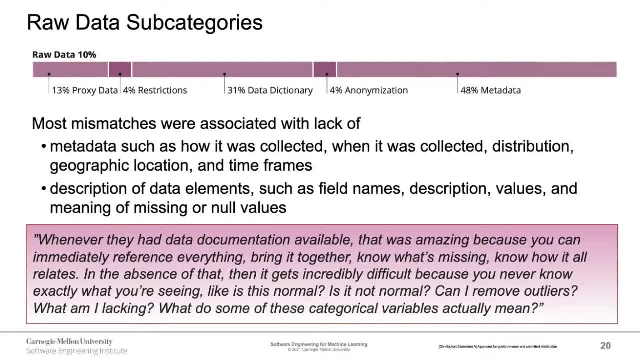 and that the data scientists have to transform- or the data engineers, depending on your organization- has to transform into training data, And really most mismatches had to do with lack of metadata. So one thing is to have, for example, a data dictionary. 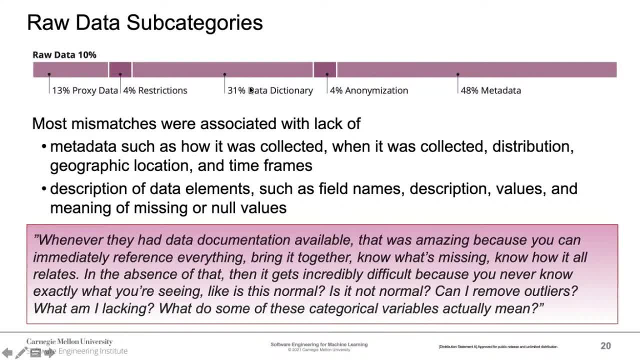 which is the second- this over here, that was the second most popular- where a data dictionary is kind of like the traditional data dictionary that most of us in the software engineering field know right Now. this input is of this type and this is what it is. 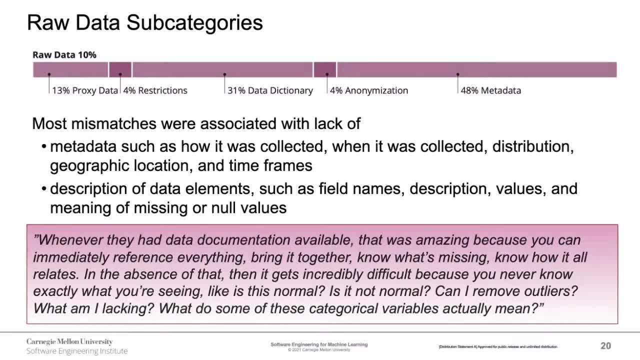 and these are the values and all that stuff. But metadata was the one that is most important because it's basically okay, it's great that I know what the data is, but for me to do my job, for me to do my data cleansing- 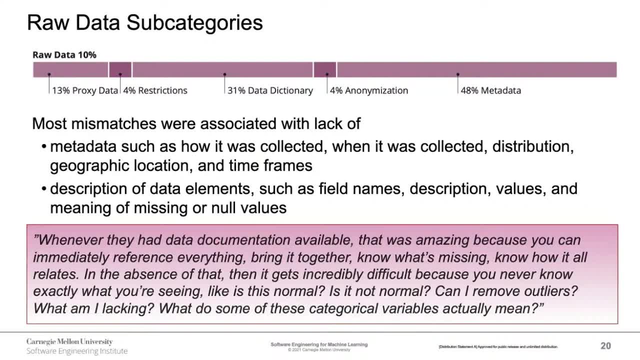 for me to do my data preparation, I need to have some more information. So, for example, where is this data coming from? When was it collected? What do these missing values mean? What is it? is what I'm seeing? is that normal? 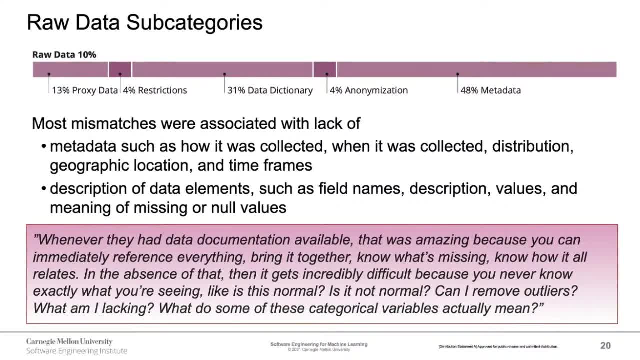 Is that an outlier? Am I seeing seasonal effects in this data? So being able to have that metadata can definitely help the data scientists do a much better job, and that is something that they felt that is not often shared. Once again, here's some data. 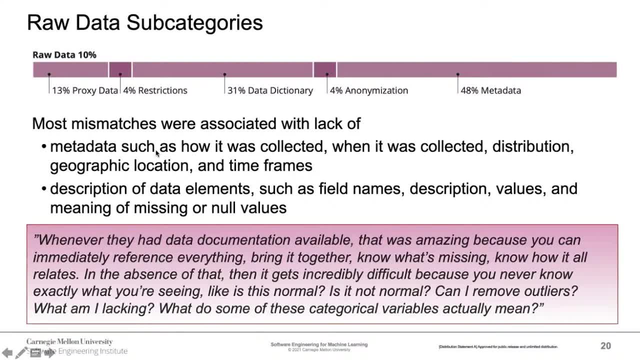 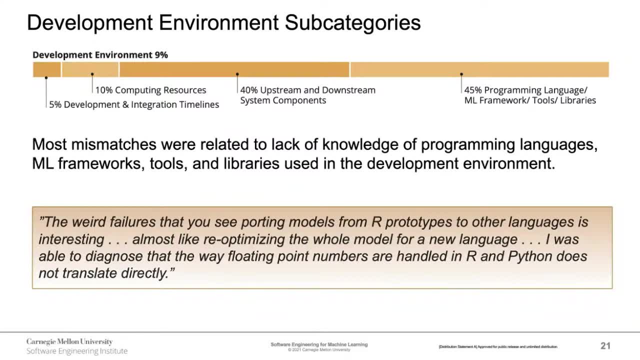 go do some data science to it, right? So that's related to some of the raw data subcategories. As far as development environment, definitely the number one mismatch had to do- and I guess you guys predicted it- what had to do with programming language. 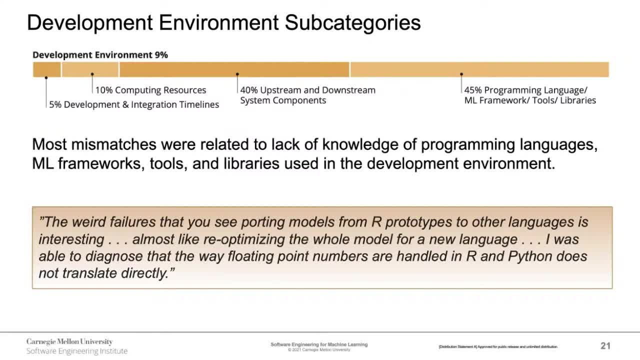 not knowing, not sharing information about the programming language that was used to develop the model or, the other way around, the ML framework, tools and libraries. And, for example, this was a quote from a software engineer that said that some of the weird. 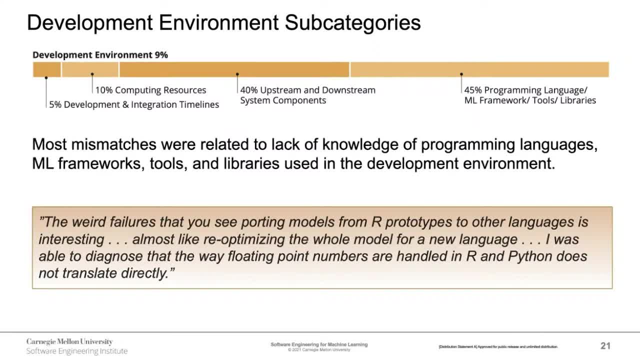 they saw so many failures trying to put models from R to, for example, Python And, for example, there was one specific instance that was shared with us where they were trying to reproduce the model in Python and it just wasn't. they weren't getting the same answers. 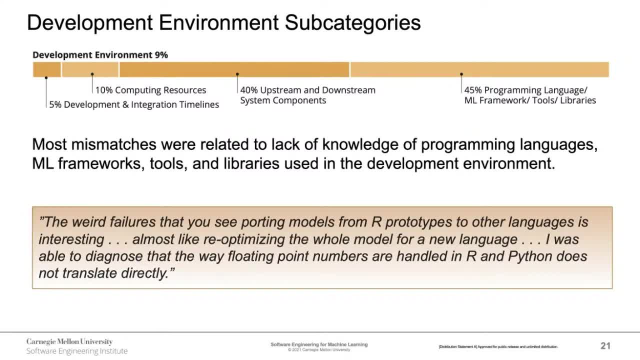 and they realized that there was an underlying, very low level difference between the way two different libraries were handing floating-quote numbers. that was causing the differences. So again, ideally you want to be in an environment where you don't have to do any porting. 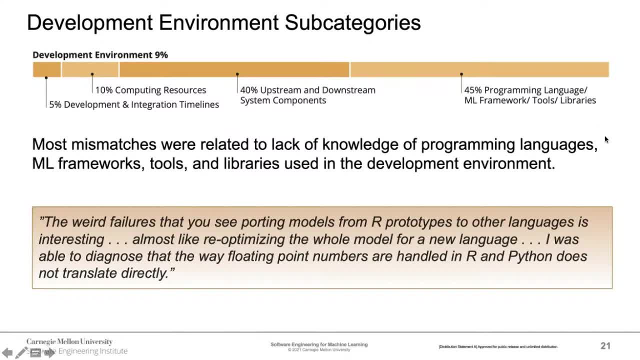 but again, if there has to be some porting done, that's something that has to be shared from the start so that people can make decisions on whether, yes, we do have to port and we have to put that task of porting into the schedule. 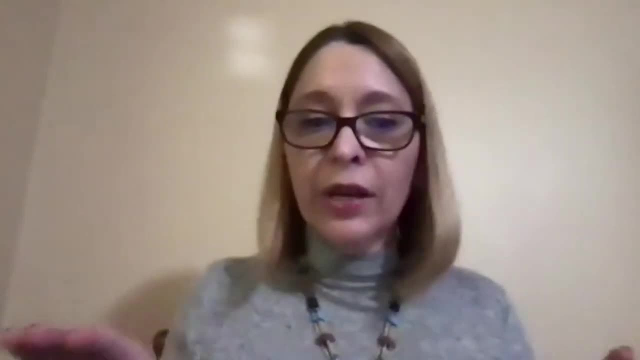 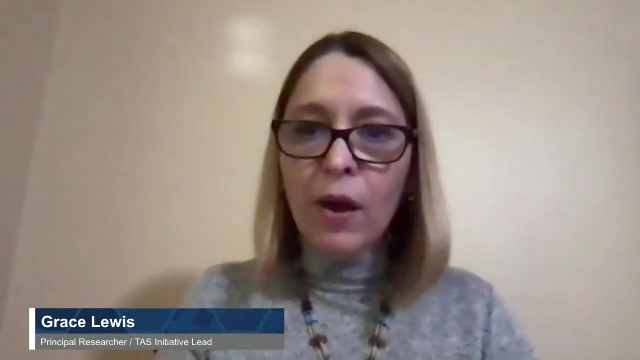 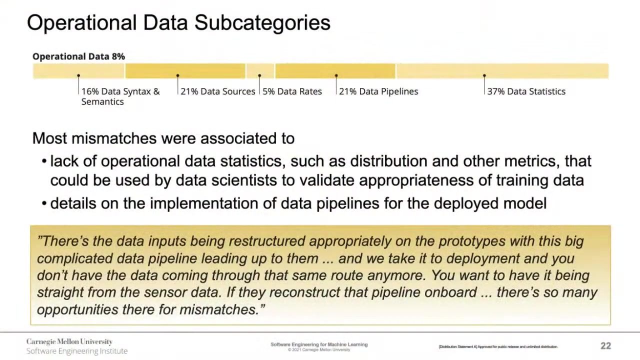 or we're just going to agree that this is the language that we use, period. So, going to the next category, operational data, this is the data that the model actually encounters at runtime, And most matches had to do with lack of data statistics. 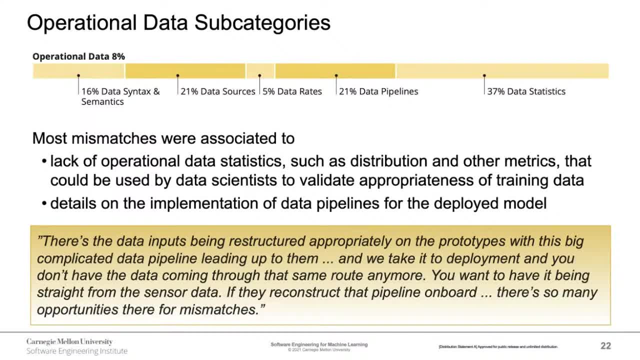 and this goes back to the training serving skew, which is that the data scientists train the model and, for one reason or another, the model wasn't trained with data that really represented the operational environment. So number one was data statistics. having much more information about the statistics, 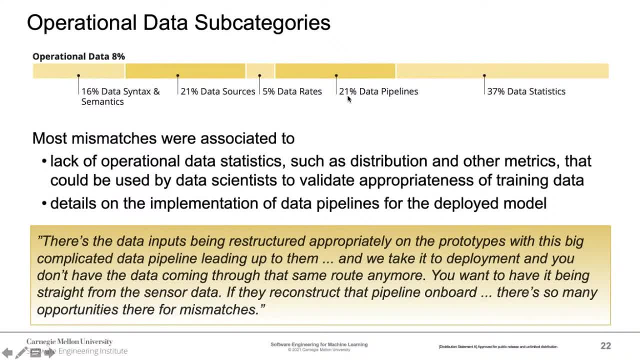 of the actual operational data that the model is going to encounter and, I guess, tied for second is this idea of data pipelines and data sources. Another thing that we saw as problematic- and this was constant in some of the interviews- was this idea of not knowing what part of the data pipeline 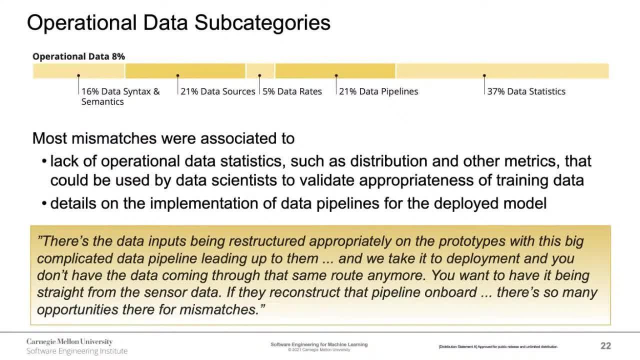 is outside of the model and what part of the data pipeline is inside the model, and this is something that shows up again with respect to training data and so, for example, having information about data statistics, about what exactly do the data pipelines look in the actual operational environment and, for example, 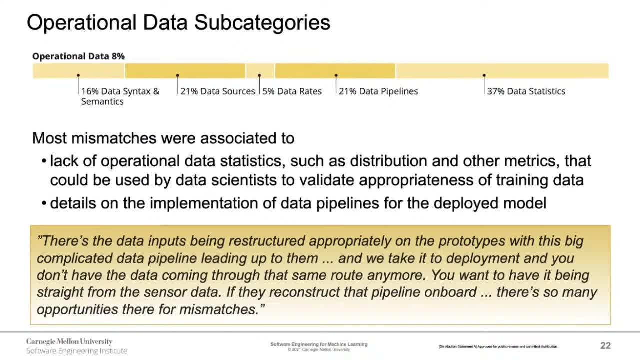 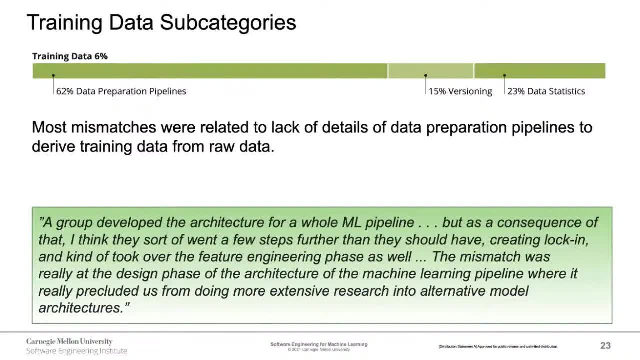 what the actual data sources are, that is there definitely some information that should be shared, because that that allows, for example, data scientists, when they're building their models, to make much better decisions. the next category was training data, and this is something that showed up both in the operational data and the training data, but most of them had to do with just 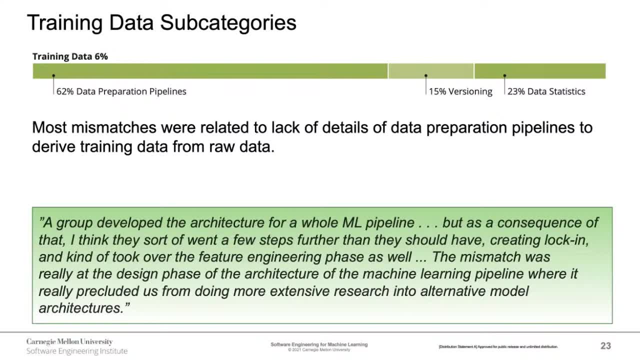 um data preparation pipelines, the fact that, for example, when, when, the when the model is going over to, you know, hand it over. when the model is handed over um, all the data preparation code is either often not not handled or was done in an ad hoc way and therefore has to be reproduced in the in the 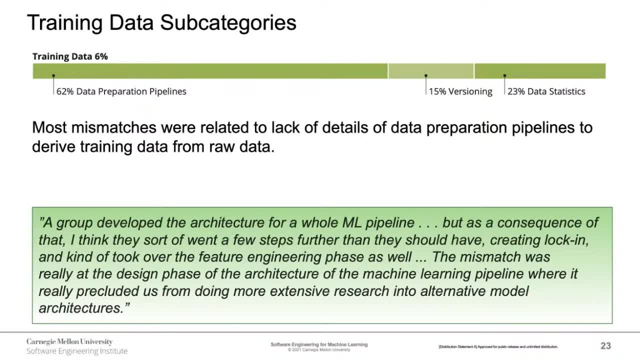 in the development environment in this case. and so, for example, this particular quote- it's a it kind of this quote is interesting because it touches on a, on a different, on several mismatches. but basically, um, they said that a group developed the architecture for a whole machine learning. 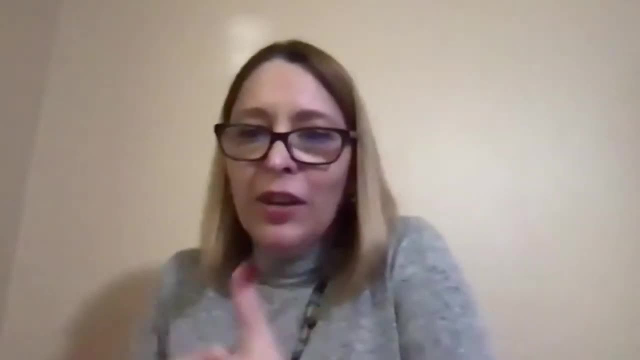 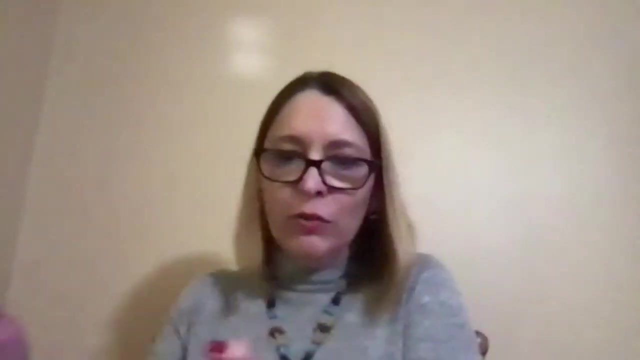 pipeline and but the pipeline went a little bit into feature engineering as well, so that that boundary between this is the data pipeline and this is where the modeling starts, was a little bit too much into the right so, for example, and that precluded them from doing, from using, uh, doing. 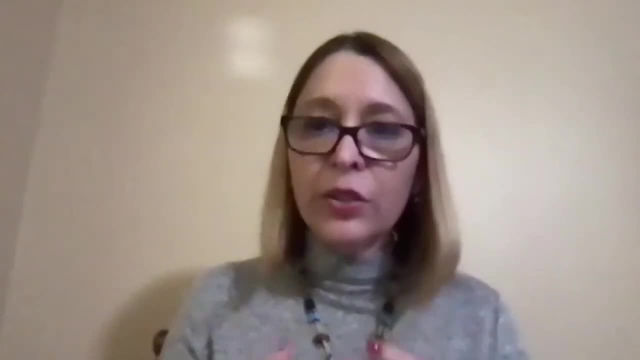 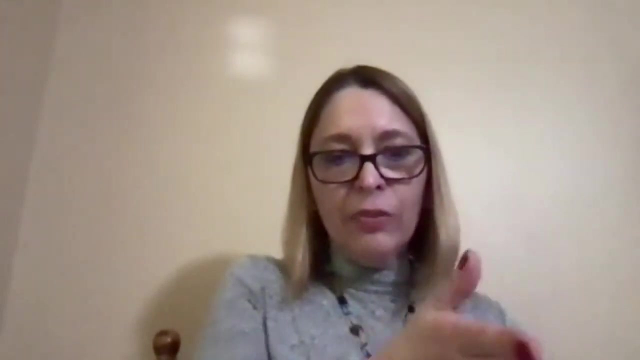 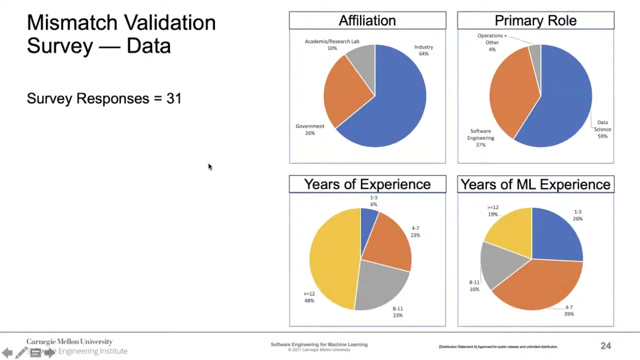 like different alternatives, for example, into into feature engineering, and they were kind of like locked into an architecture, um, like i said, very specific quote, but it shows why it's important. separation between: this is the data pipeline. this is, this is the model component, um, and talk to you for some questions here. yes, i was going to stop right here. this is, this is perfect. 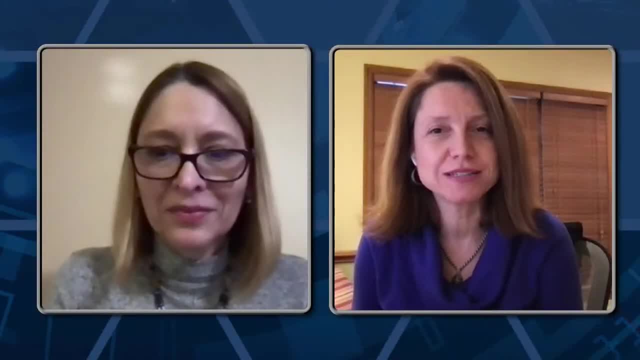 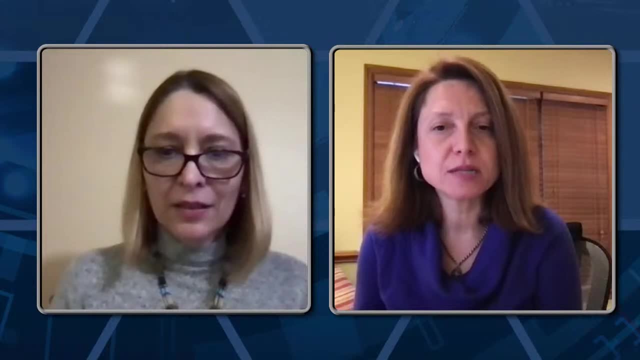 okay, uh, because there's a very good discussion and questions going on in the chat. i don't want you to miss it. so one is: uh, she can't asks whether, if we can repeat what an ml mismatch is, in particular, is it between practitioner opinion and empirical evidence? so let's clarify again for the 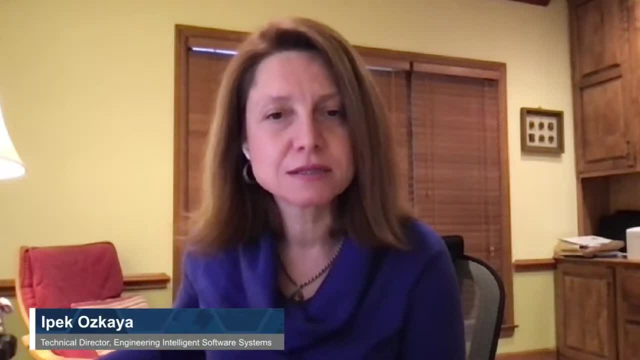 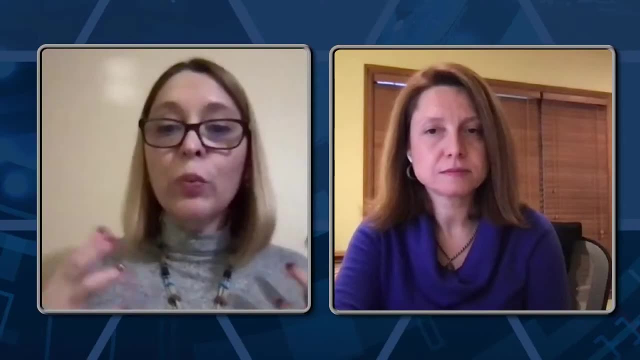 audience so that they can follow the rest of the question. um, i think that's a very good question. um, i think that's a very good question. um, i think that's a very good question as well. absolutely, so. what we define as machine learning mismatch is a problem that occurs when you're trying to put a model into. 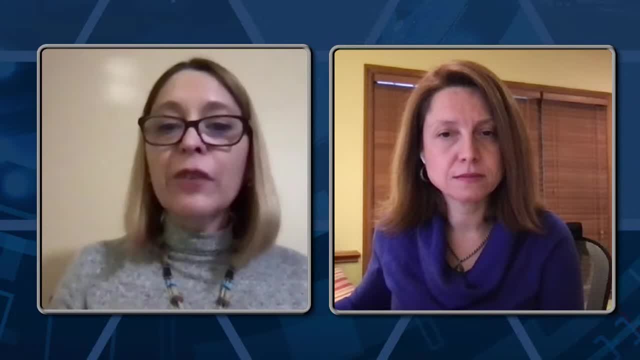 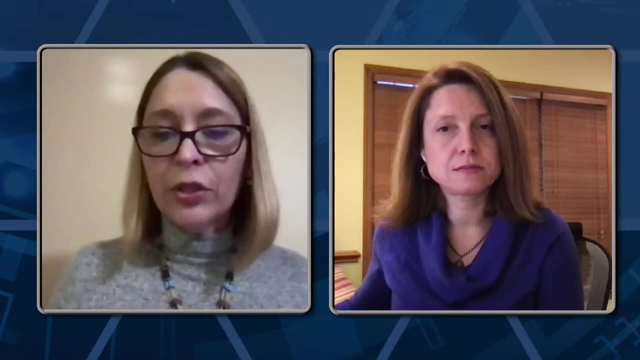 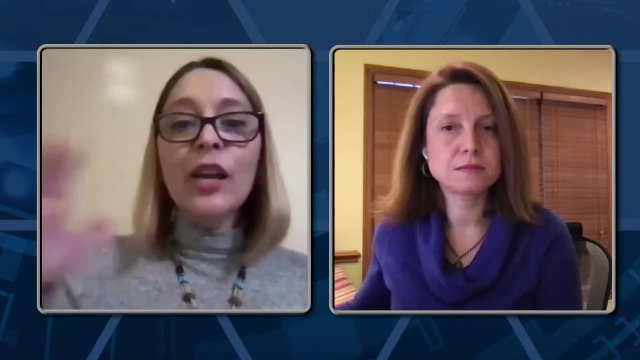 production and that. and that problem occurs because different stakeholders made incorrect assumptions about other parts of the system. for example, as a software engineer, i made a totally incorrect assumption about the language that the, that, the uh, that the model was developed in. or as a data scientist, i made an incorrect assumption about what was the account of the 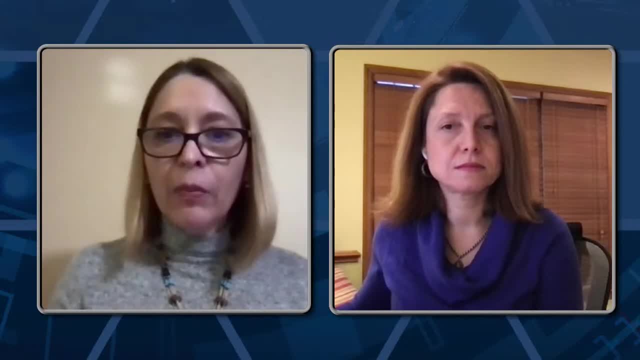 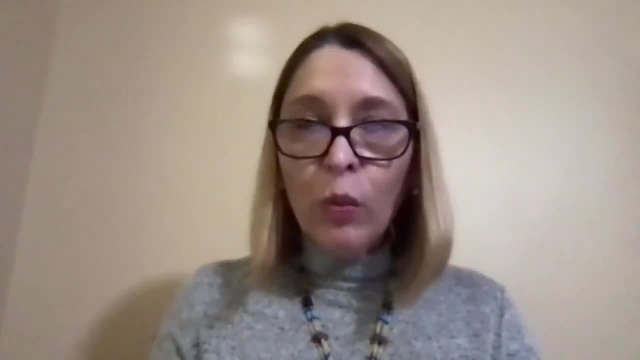 expected accuracy of this model or as an operations part of the operations staff, i made a very incorrect assumption about what was the data that i was supposed to be logging in the operational environment. so that's one part of mismatch and the the further explanation of mismatch is that for our study, the idea was that we would every every example of mismatch, including 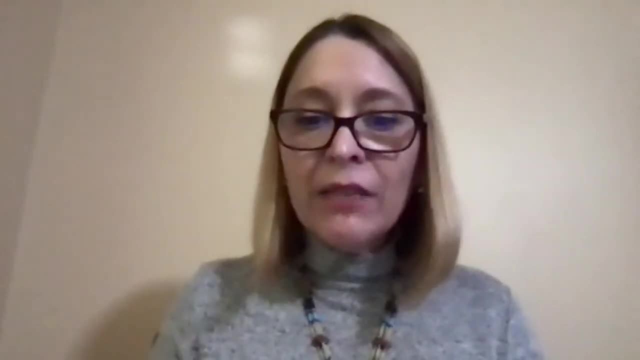 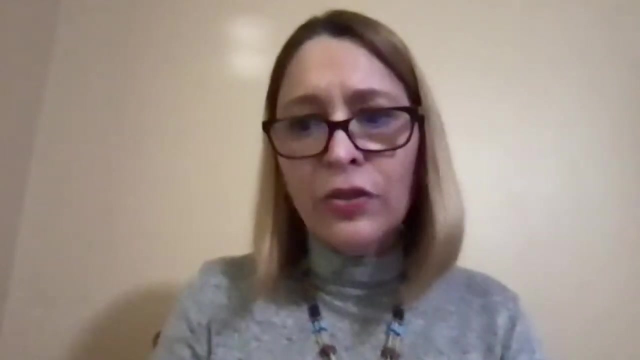 the ones that i just mentioned could be traced back to a piece of information that, if shared, would have avoided that mismatch. so it's not. it's not mismatched between empirical and and practitioner, but rather mismatch between different stakeholders that participate in the development of this ml enabled system. hopefully that answers the question and, uh, as our audience. 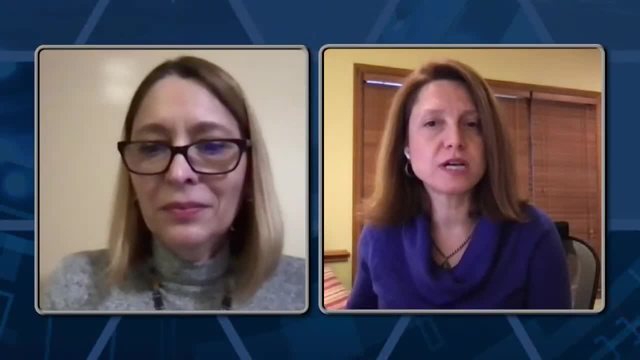 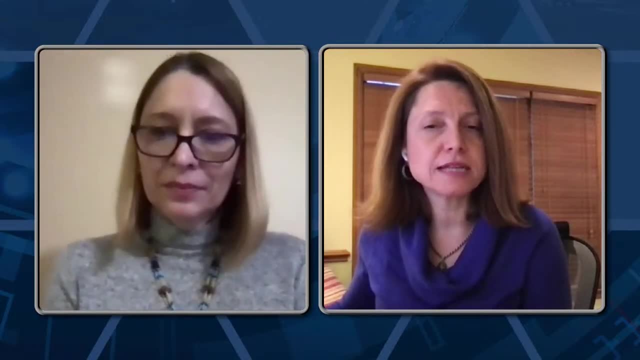 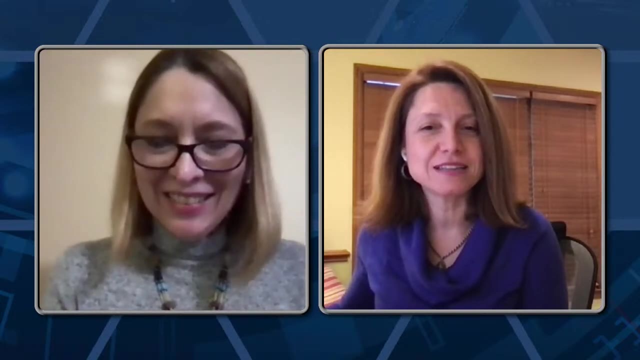 will also find out as we go about. the idea is that you can actually formalize and maybe automate parts of it so that you can be more consistent among the information shared. so next question is from matt from sunny pittsburgh, pennsylvania, and he asks: did you find situations where the fact that 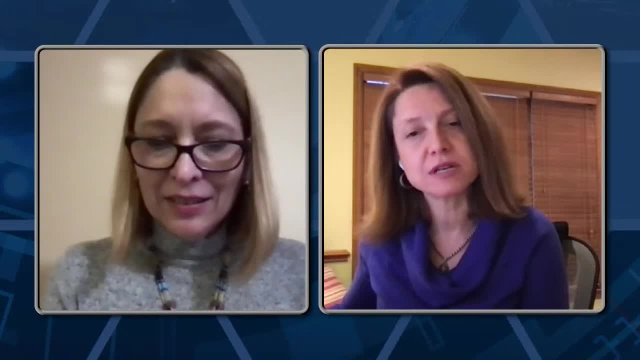 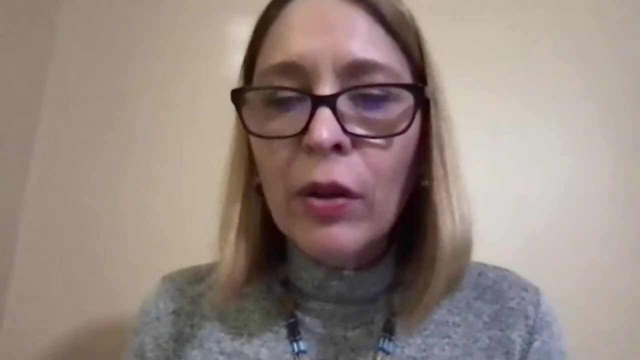 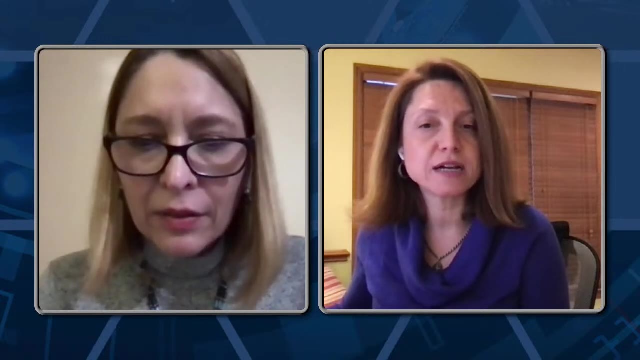 this was a system with an ml component added additional requirements on the ml model that weren't obvious until the system was deployed. repeat, repeat what you said. after ml component. i missed the last part of the question, i'm sorry. uh, let me repeat it all. did you find situations where the fact that 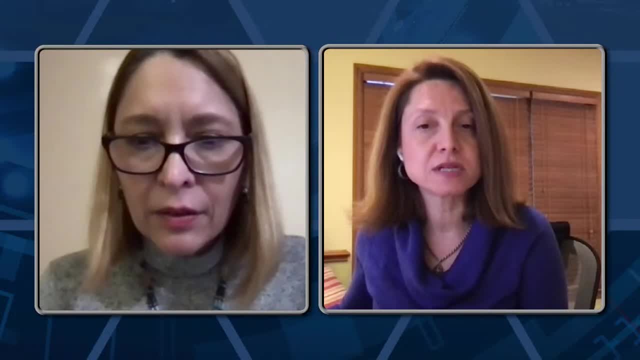 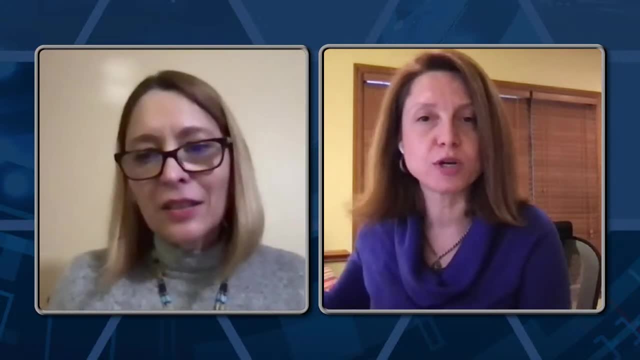 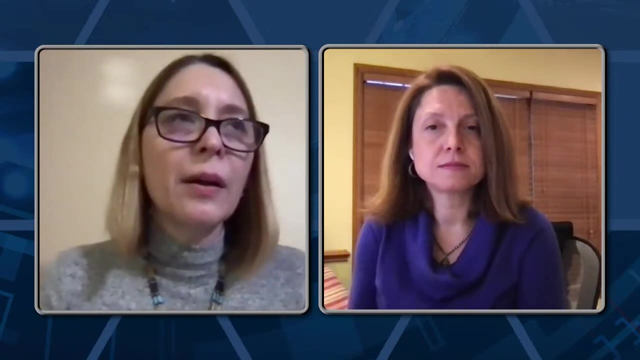 there was a system with an ml component added additional requirements on the ml model that weren't obvious until the system was deployed. it's really going back to what you could observe in deployment versus what you could gather during the requirements phase. yeah, so, so here. so here's one. here's one of those. um, actually, yeah, this is. 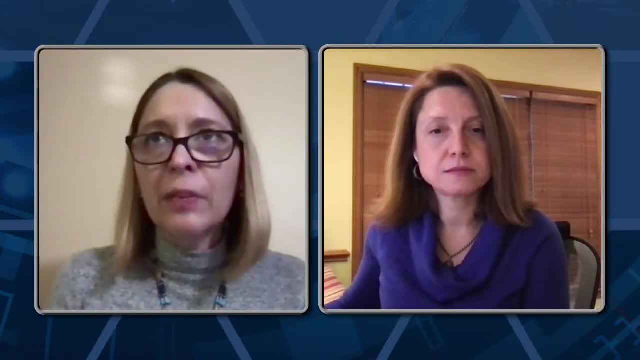 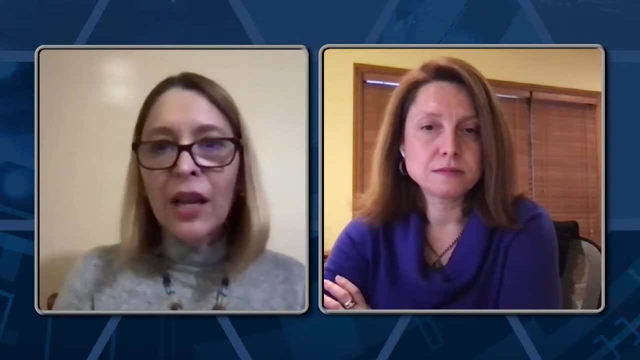 that's a very good question. so here's one of those. going back to the very first question that epec asked me, that said: you know which practices change, or with the, which practice have to change or which practices can be used the same, and all that stuff. so requirements engineering. 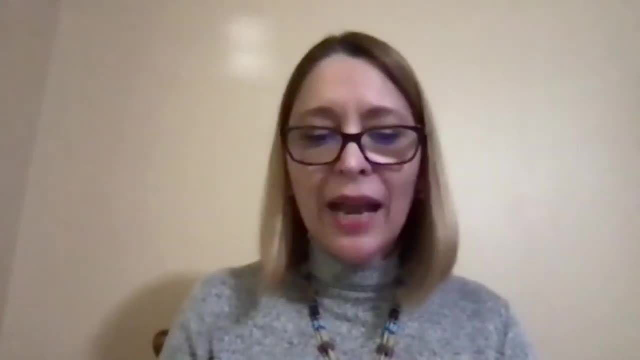 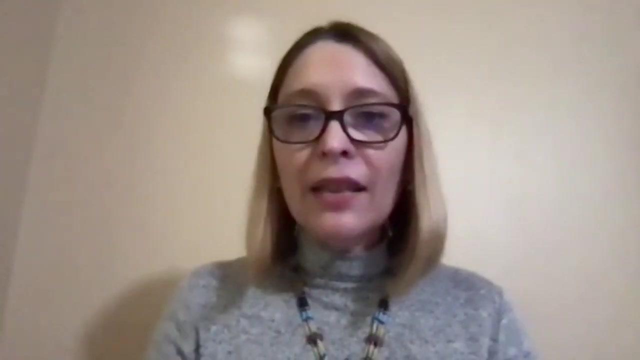 for these types of components. actually, it's actually quite an active, quite an active um area right now, obviously because of the you know the interest in machine learning and i would say, from a requirements engineering perspective, all the techniques that we use to gather requirements are exactly the same right, because in the end, going back to what a machine learning component 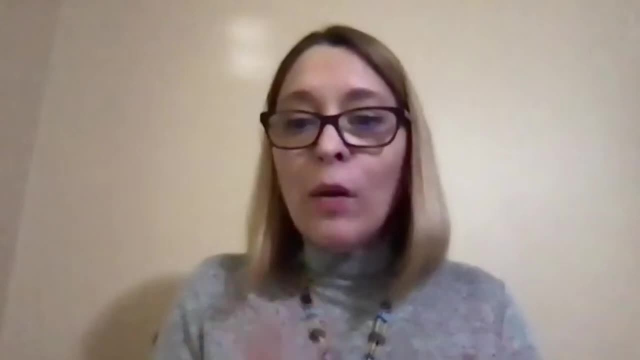 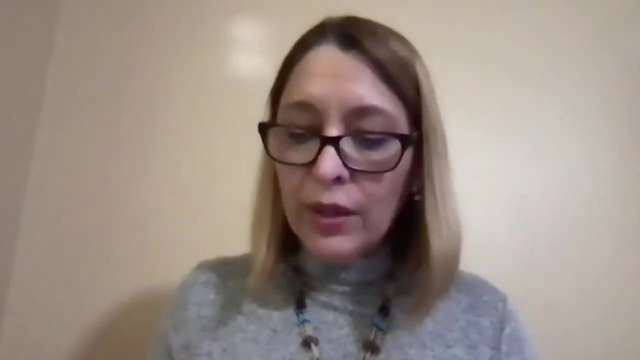 is? it is a piece of code, it's just a special piece of code. but what changes are the questions? so let me give you an example of that, of that. so, for example, a question that we might not be used to asking during requirements engineering would be: what is the risk of having a? what is the risk of 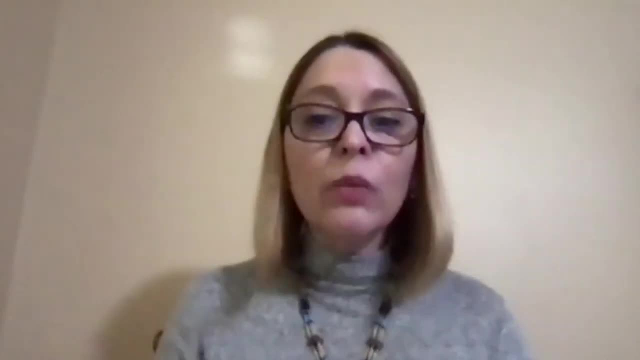 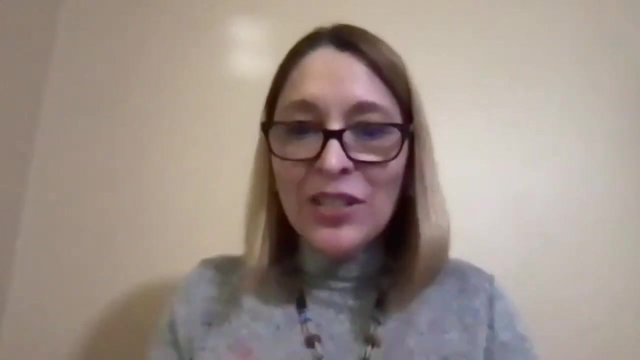 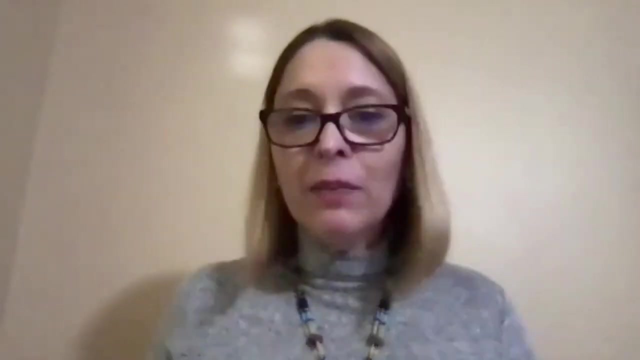 the model, producing a false negative. that is a question that we normally wouldn't ask for requirements engineering, but for this type of system it's very important to ask because, again, as software engineers, we have to live with the fact that these models are going to degrade over time, that they're very dependent on data and that any changes in the data are going to change. 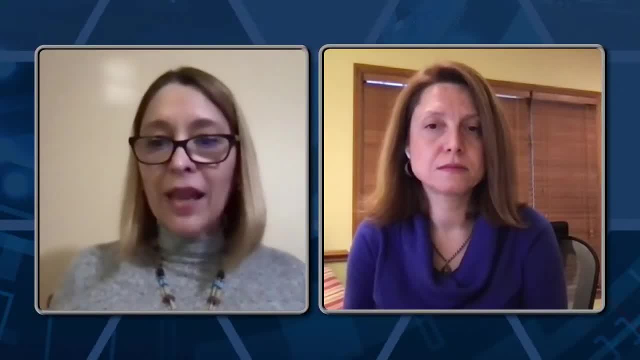 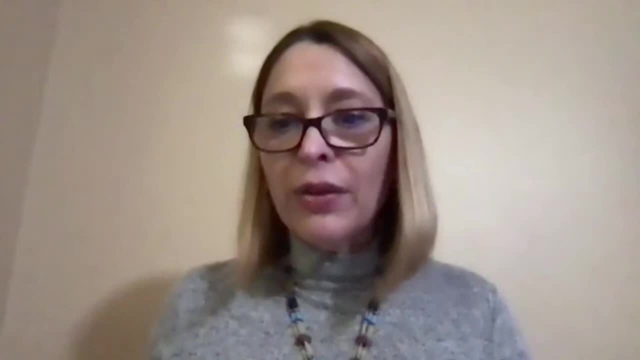 the performance of the model. so that's an example of something that where this requirements engineering, now a specific thing that you wouldn't know until after the after the model is developed. so the examples mostly, to be honest, mostly had to do with with monitoring, and this goes back to why. 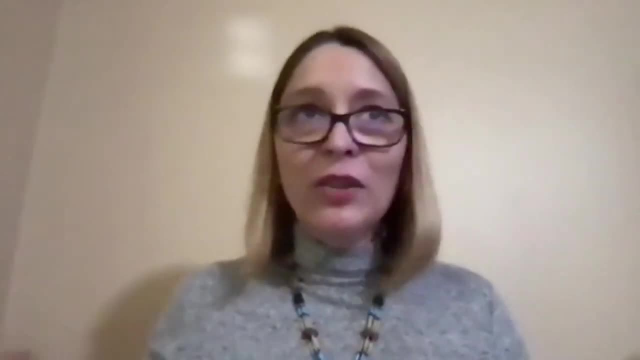 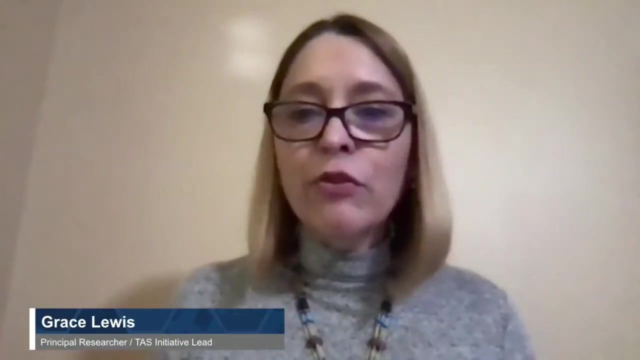 we think it's so important. i get, we, we, you know we, the model was performing, it was, it was doing great. all of a sudden it starts producing a bad prediction and the data scientists have no data to work from because nobody thought about logging this particular- i think this particular information or 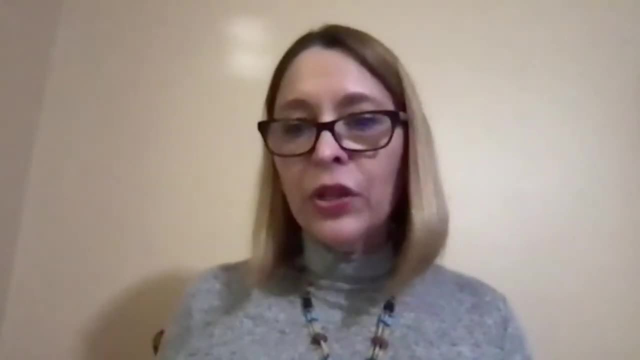 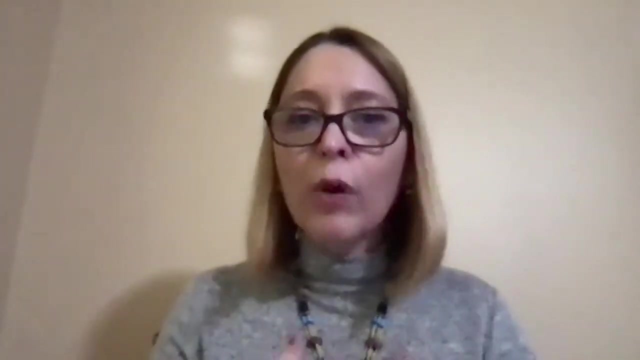 this particular um, a combination of input outputs. so yeah, there are lots. there are lots of. i can think of many examples that i don't want to get into, but there are a lot of examples that i don't want to get into them, but the whole point behind what we're trying to do is to make all that. 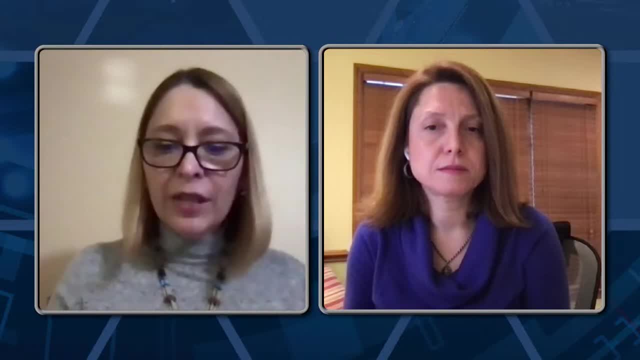 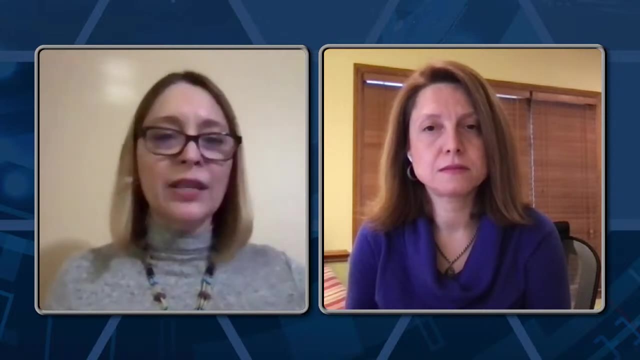 information explicit, so that that doesn't happen. if different parts, if different stakeholders are filling out different descriptors for the system, all that information is being shared, and so a data scientist could say, ah, i understand, now, this is this is what the operational environment is. or the software engineer can say, okay, this is, this is how the model was tested. this is all the testing. 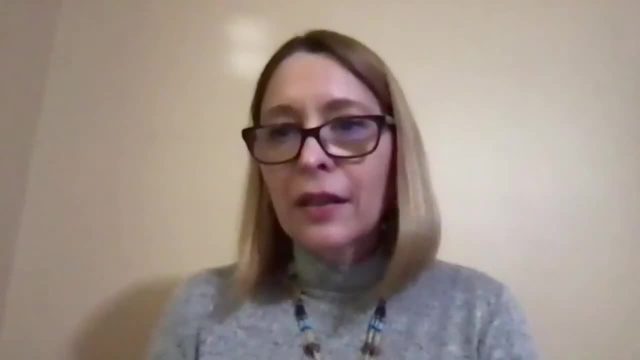 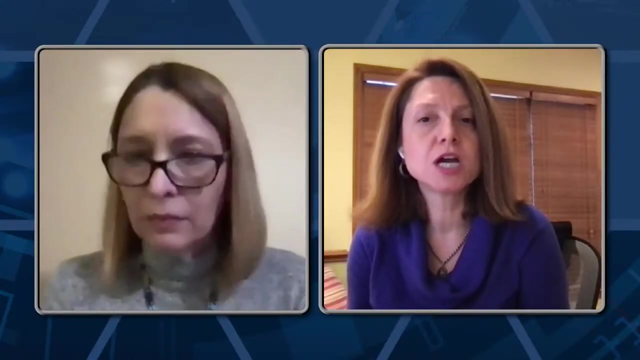 that has already been done. this is how it was evaluated, etc. and some of the mismatches that were very worse between- uh, the mismatch between trained model and the operational model could get into requirements practices, but some of the data science practices could also actually already be able to. 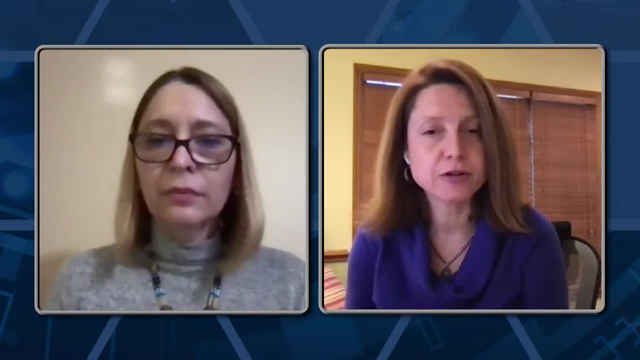 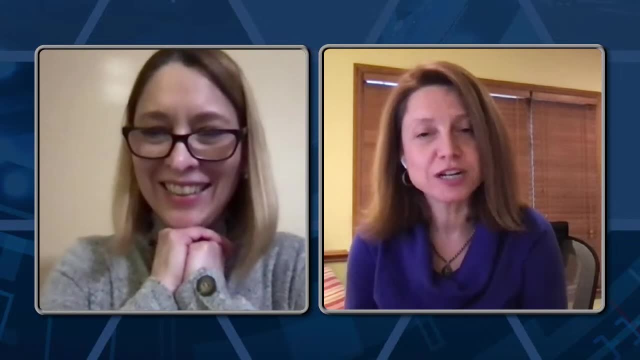 detect those. so there's aspects of both that are actually involved, but i agree it's an excellent question. the next question is one that is, uh, both near and dear to both your heart and my heart. grace, because it's related to architecture. so, and there's a couple of plus ones for this, 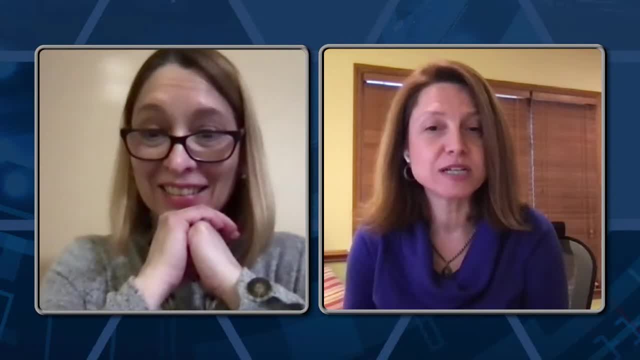 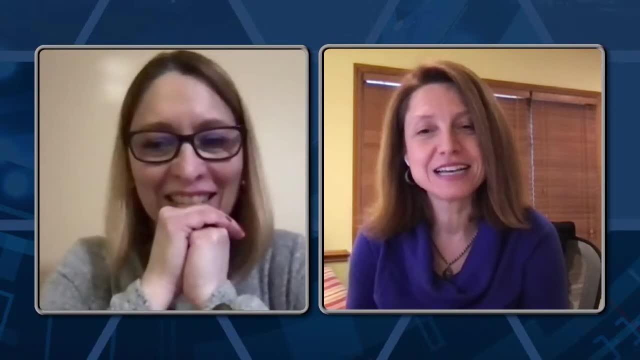 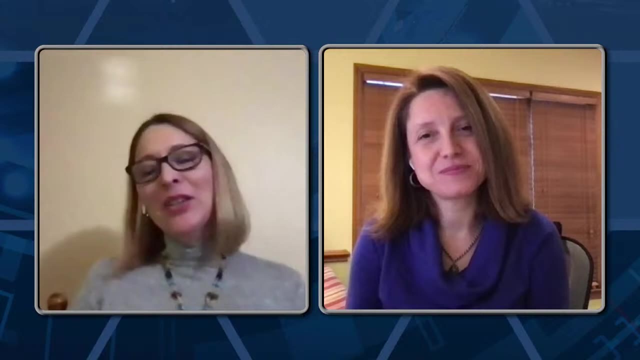 which goes: did you see any mismatches, as, uh, of expected quality attributes versus as architected quality attributes- example, performance latency scale needed to be handled but was only built for half of that. so like, oh, absolutely, absolutely. oh, there's okay, i'm gonna. i'm gonna like leave it to two, but because we, i, i don't want to run out of time before i get to my 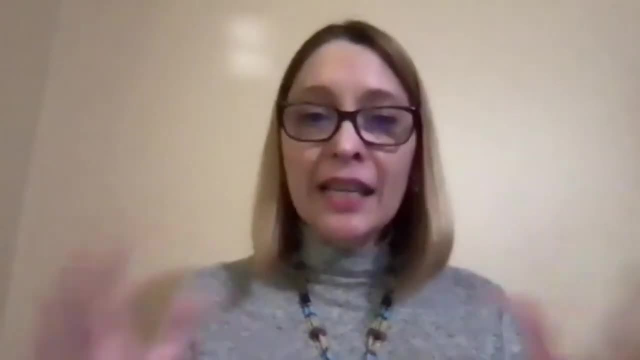 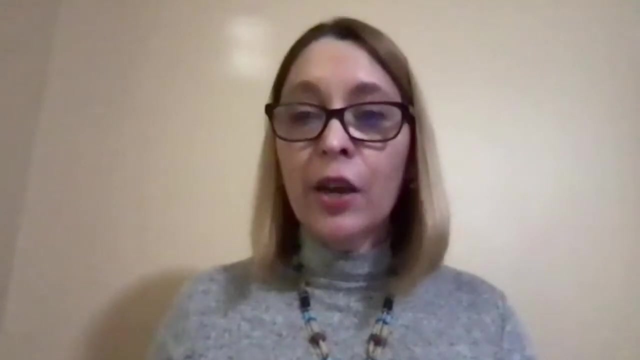 slides, but, for example, um and again, this is data. scientists are great. they're they're great people to work with. they are super knowledgeable. i, i would never know all the things that they know, but they're not trained in software engineering. they don't. they typically don't know what quality attributes are. 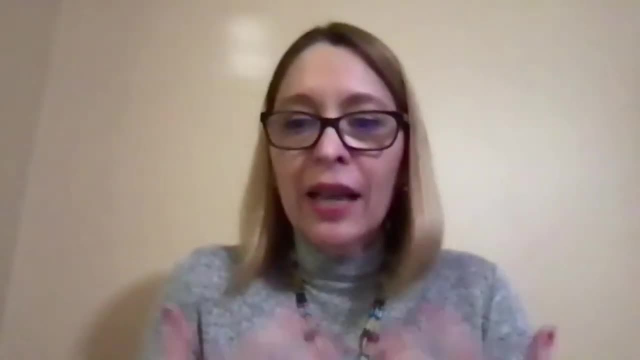 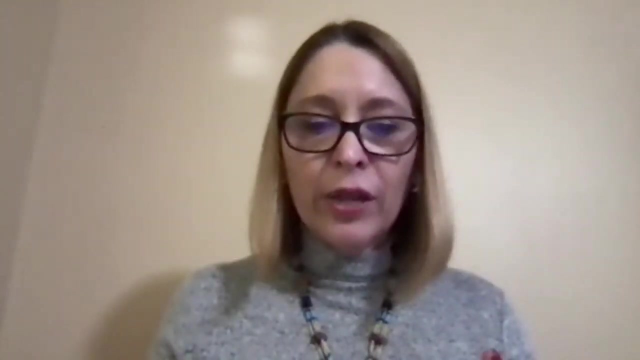 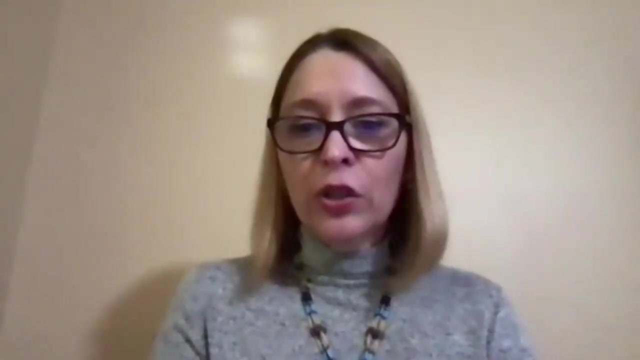 they typically don't, don't. yeah, they don't understand. they. they are very good at building their model about meeting: um, you know, 95 accuracy. once they reach 95 accuracy, they're very happy. they say, okay, the model, here it is. but for example, uh, you can imagine, okay, here's a situation, you, you, 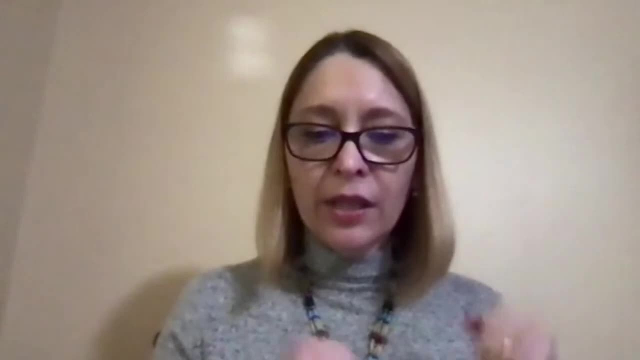 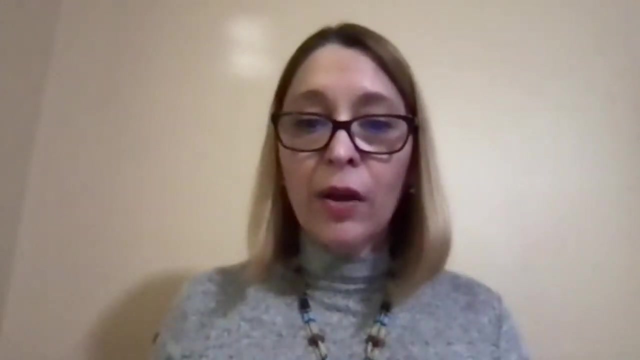 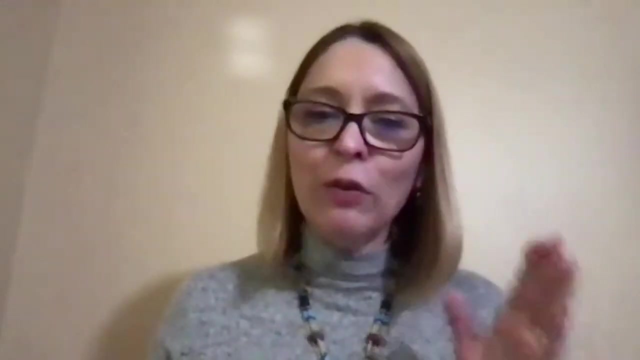 develop. you develop a, a machine learning, model 95, accuracy. you put it into production and, all of a sudden, the, the data rate, the data, the data rates for how the data is coming into the model. the model just isn't isn't, it's just not capable of of performing. see, here's the thing: performance, the way, the data. 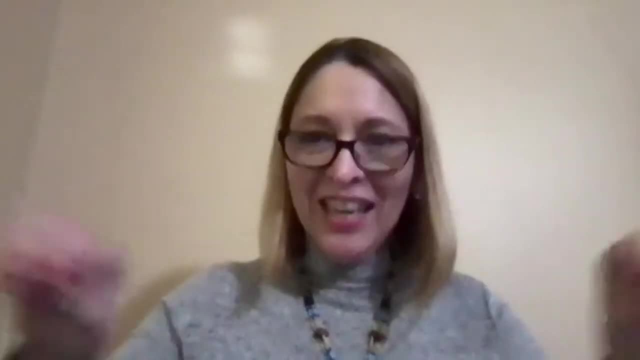 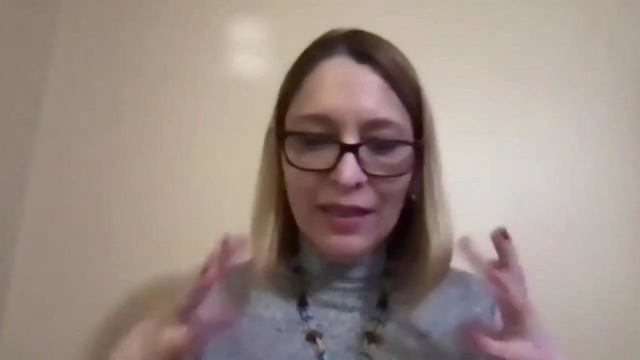 scientists use it and performance, the way we use it as software architects- is very different. so, um, the data scientist talks about accuracy, right, so let's just use accuracy. so, for example, all of it, you know this, it it's just, it it's not performing. i mean, it just can't handle the data. 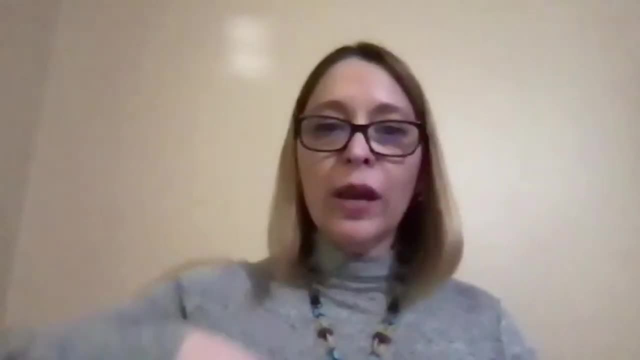 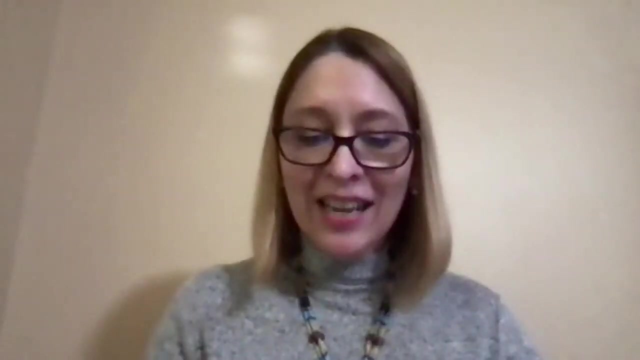 that's coming in. so all of a sudden now you have to replicate that model four times. so you create, you create four instances of the model And then what happens- which is very interesting is again, models are very data dependent, right? So if you start load balancing, 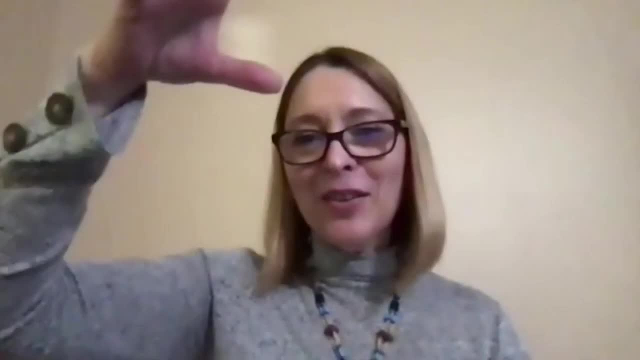 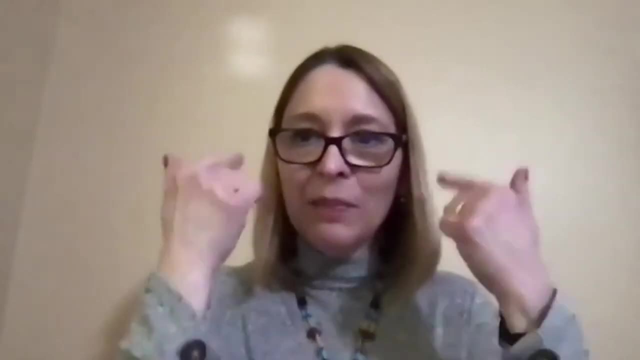 different data starts going to different instances of the model and now you have four identical models that are performing in the data science sense very differently and anyway. But those are examples of things that we have to keep in mind of. would anything have been done different? 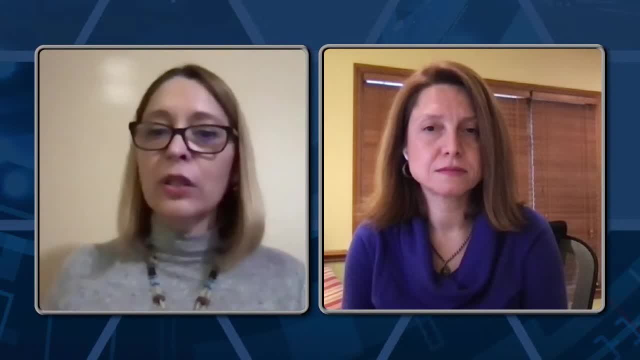 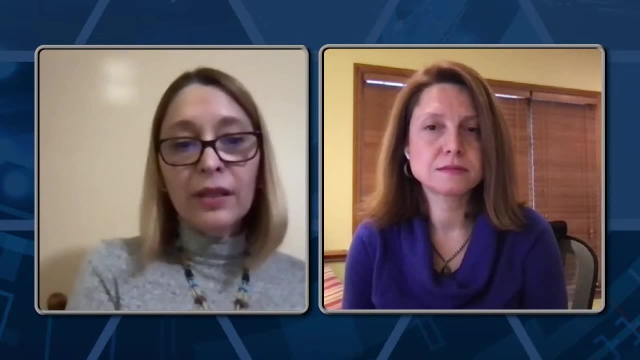 by the data scientist if the data scientist knew, for example, that the model was going to be replicated for time? Or would the data scientist would have done anything different if the data scientist knew that the data was coming in at this speed instead of that speed? 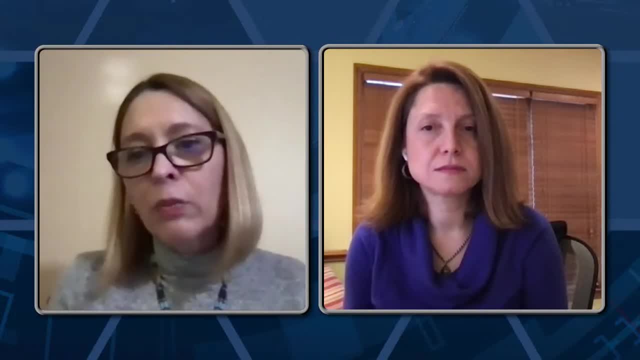 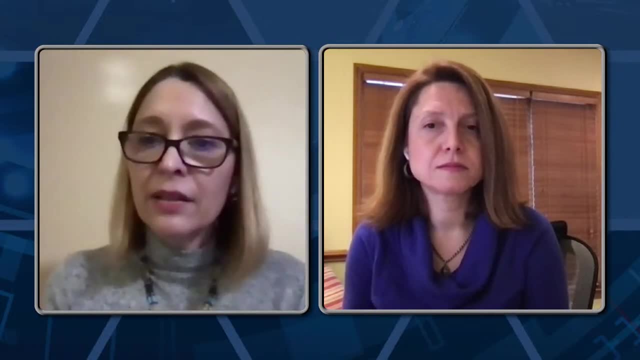 So, yeah, there are many like that. I think the main one is performance and scalability. Those are ones that are very dear to our hearts as software architects, but it's just not something that the data scientists envision. They just produce a model, and they produce an awesome model. 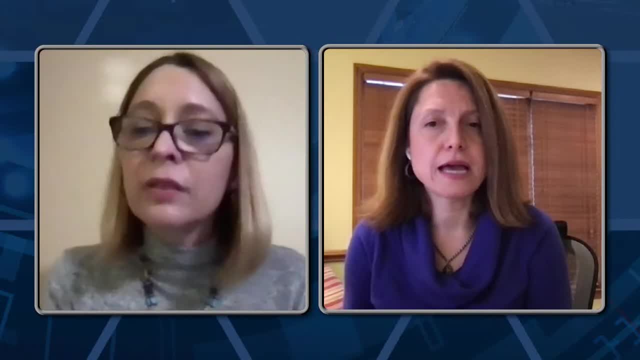 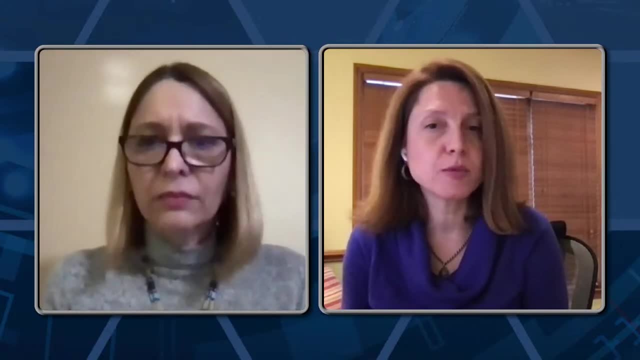 But thinking about how to put it into production, it's a whole different conversation. And the monitoring aspects and how the data engineering and data pipeline aspects there were. so I guess, in short, yes, there were quite a number of those that were identified and we're actually actively working on. 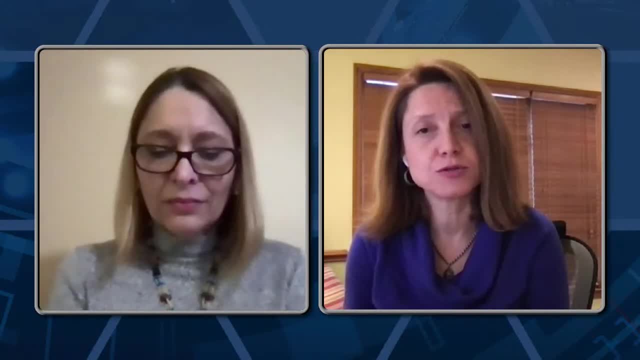 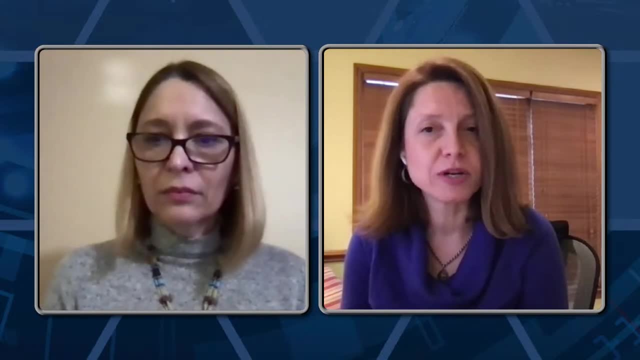 both doing case studies, working with our organizations, as well as our research. So once we have more substantial information accumulated, we'll definitely come out and do another webinar and address this, for sure, in detail. So, Grace, in the interest of time, let's move on. 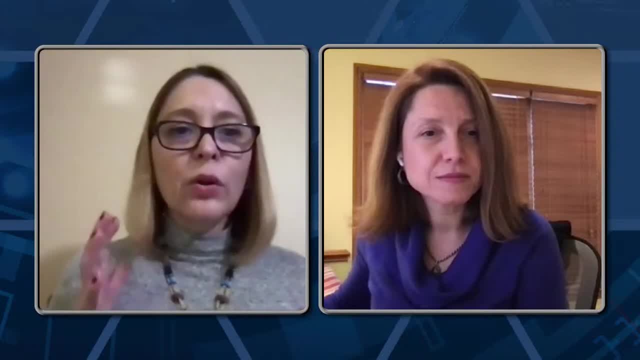 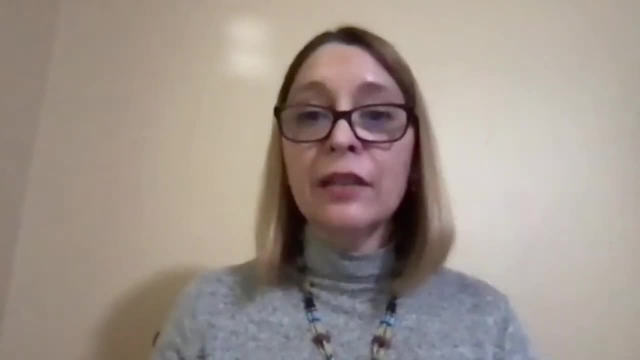 but there are great questions coming. Oh, thanks, that's great. So now obviously we came up with the mismatches. now we needed to validate it And basically we conducted a survey where the main question was: how important is it for you as a practitioner? 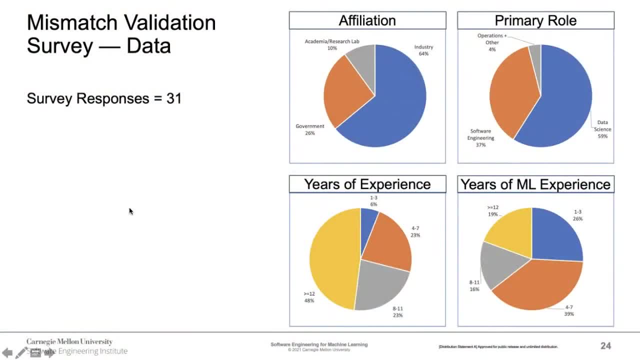 to be aware of this information in order to avoid mismatch. We had 31 responses to our survey, not as much as we wanted to, but then again, we were very specifically targeting people that were involved in the development of machine learning enabled systems. 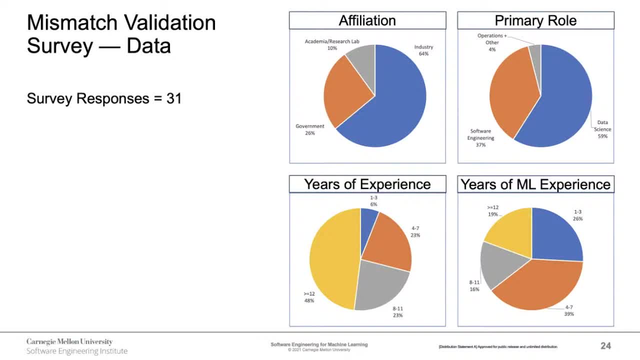 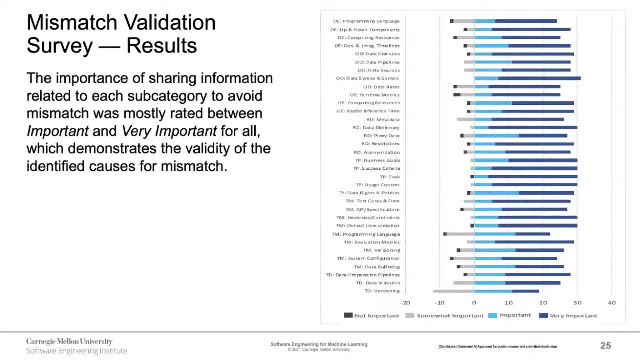 And because this is kind of a new discipline outside of the large companies, it's hard to get people that are working exactly in this area and it was great. I mean, the results were great, As you can see in the diagram. the importance of sharing information. 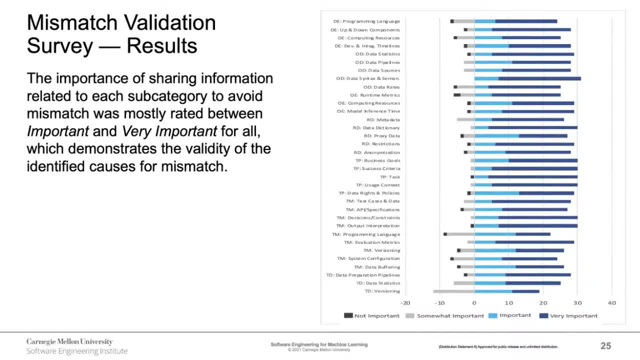 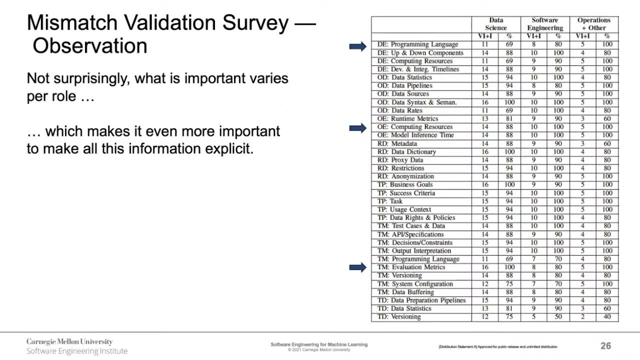 for every single category, was mostly rated between important and very important, which was good for our study, because it showed that the information that we had gathered, at least, was representative of information that these survey respondents thought should be shared. Now an observation, and this shouldn't be surprising. 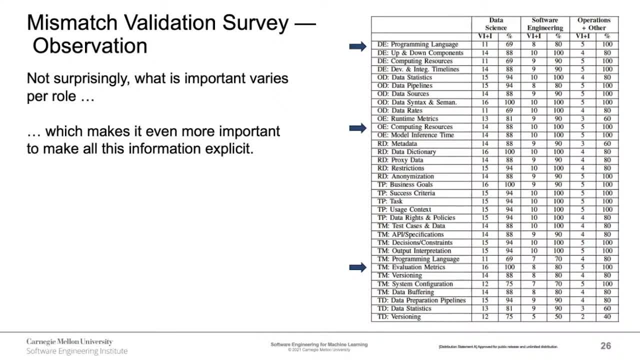 to anyone. but what is important varies per role, And those three they're a very interesting example. So, for example, knowing the programming language, It's funny because those of you that are here, for example, that I imagine maybe come from the software engineering domain. 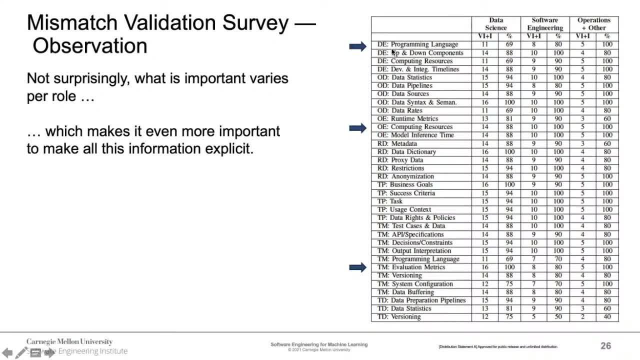 software engineering institute right. So, for example, knowing the programming language used in the development environment or sharing that information, for software engineers 80%, for operations 100%, but for the data scientists only 69%. Knowing what computing resources are available: 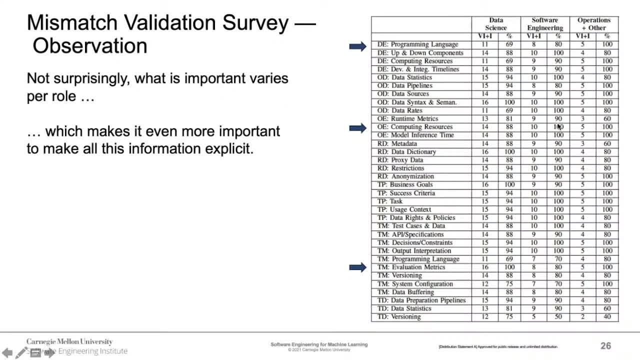 in the operational environment: 100% for both operations and software engineers. data science: 88% Evaluation metrics. I am so sorry For the data scientists: 100%, because this is what they need to have in order to do their job. 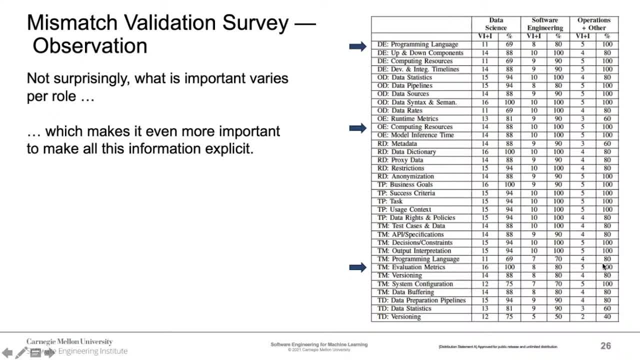 Whereas for software engineers, for example, it was only 80%, But again for operations, 100%, because this is something where these two perspectives are the ones that are most involved. So I think, even though it was a small-scale survey, this particular observation to me is: 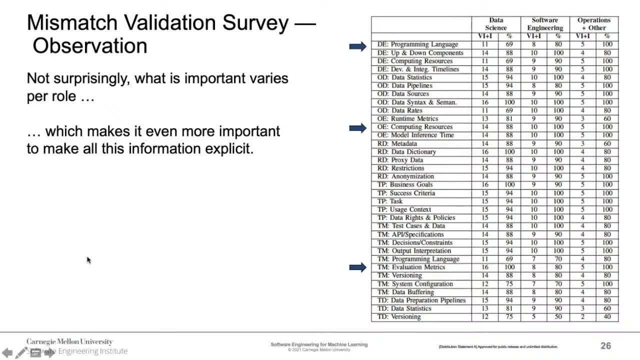 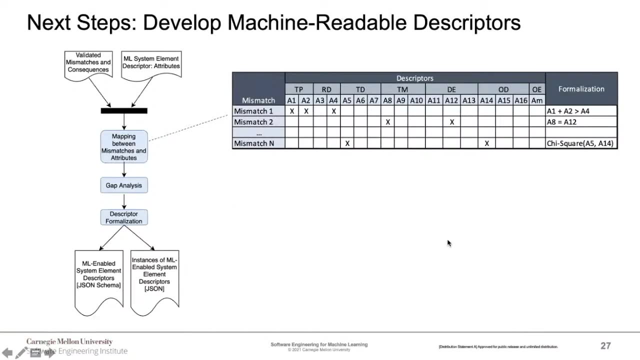 very important, because I think it makes what we're doing even more relevant: The fact that for different roles, different things are less or more important, but that you need to look at them together because they're important for somebody. And so that finishes the results of phase one, And this is what we did in phase two. This was 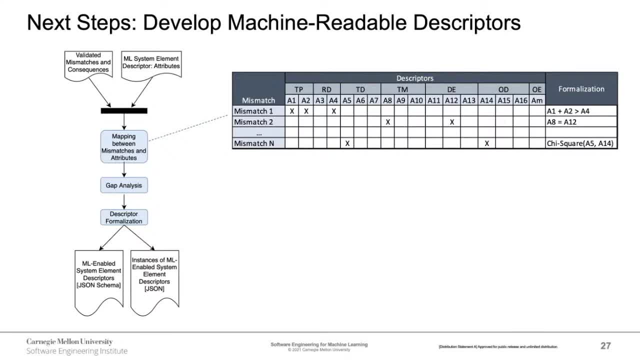 already concluded but we're not reporting on this. So after we had the validated mismatches and the consequences and the system element descriptor attributes from the multivocal literature review, we did a matching between the two. So basically we have this huge spreadsheet where we had all the mismatches here as rows. 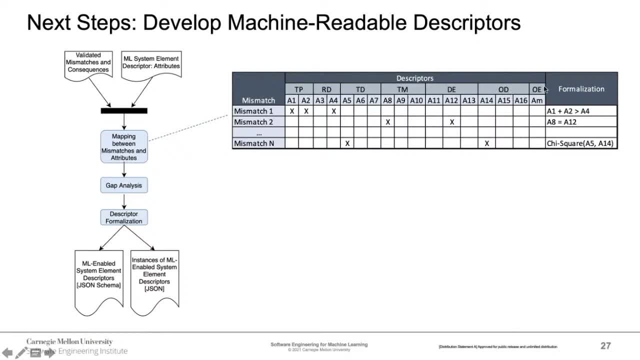 and then we have the different descriptors on the top as descriptors and their attributes. So this is trained model, This is training data, raw data, Operational data, task and purpose And what we did was a formalization. So formalization, what this means, is what would indicate that there is a mismatch. So, for example, 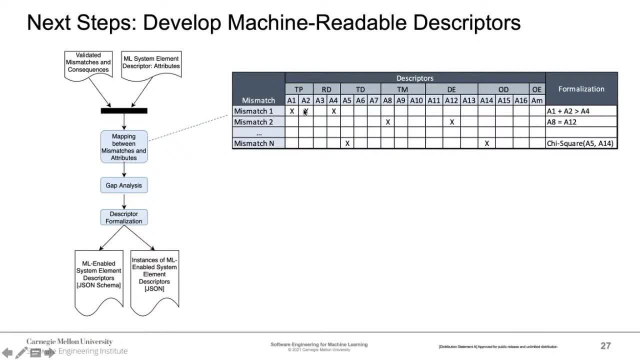 in this particular case, there's a mismatch when, if you add A1 and A2, that's greater than A4. Or there's a mismatch when these two are the same- Actually, that probably should have been different. Or there's a mismatch when, if you do a chi-square test between these two attributes. 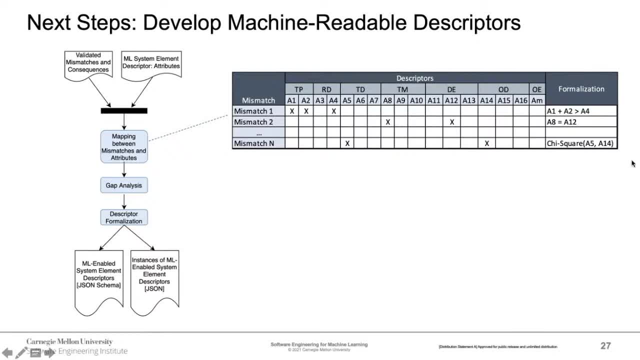 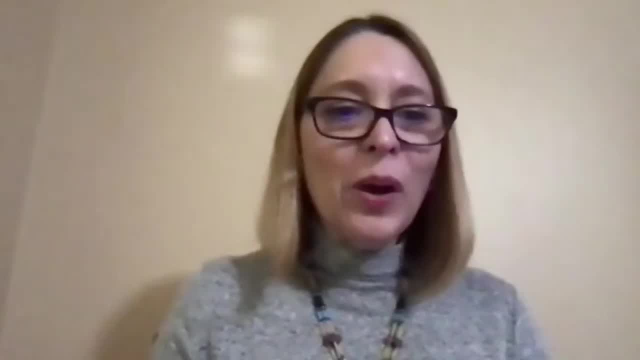 it doesn't fall within the threshold. So that's what we meant by formalization- is understanding which of these attributes could lend themselves, going back to what Ipek said, to automation. So we did that. So then we did a gap analysis. I briefly talked about this before. So, for example, 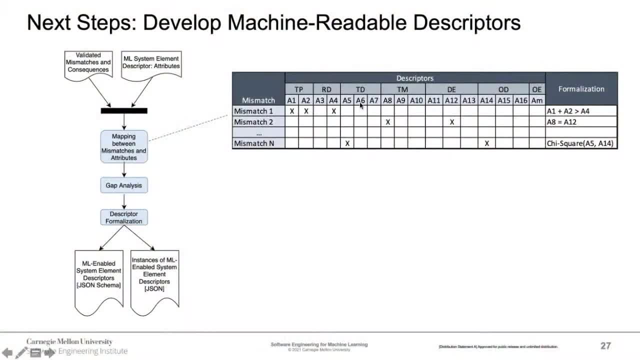 I mean, this is a very small example but for example, this attribute right here, it doesn't contribute to any mismatches. So we did analysis as to why And is there maybe a mismatch? that wasn't mentioned, particularly in the interviews, but maybe came up in the literature review as 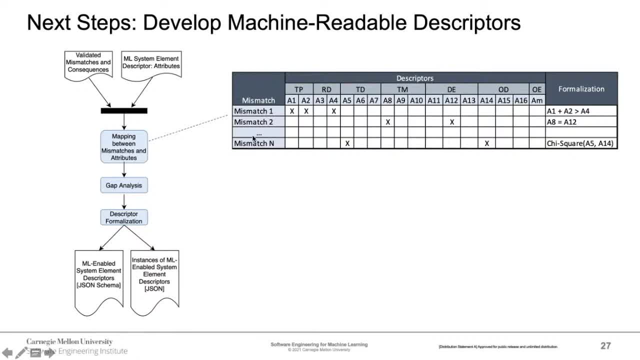 something that we should be watching. So that's what we did. So that's what we did. So that's what we did. So we did analysis for it. And the other way around, for example, this one: right here there is a mismatch, which I guess you can call it five, that of the attributes that came out of the 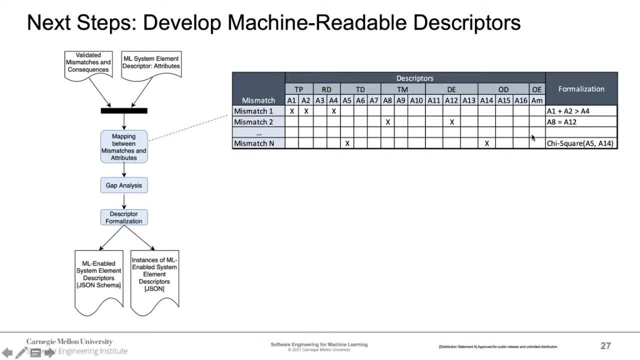 reviews. it didn't really. it doesn't seem like there's a way to detect those. So maybe that's an example of one of those. that is probably not. we can't formalize that particular one, But it was important to know which ones we could and which ones we couldn't. So after we did that, we did. 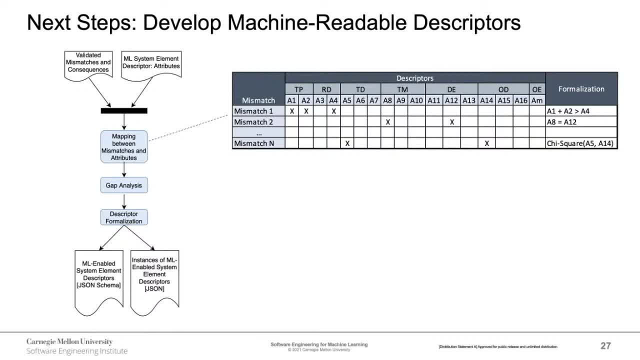 descriptor formalization And basically, what we created was adjacent schema and where we have, there's adjacent schema descriptor format And what we did was we created a description schema and we, for each one of these, for each one of the seven categories, 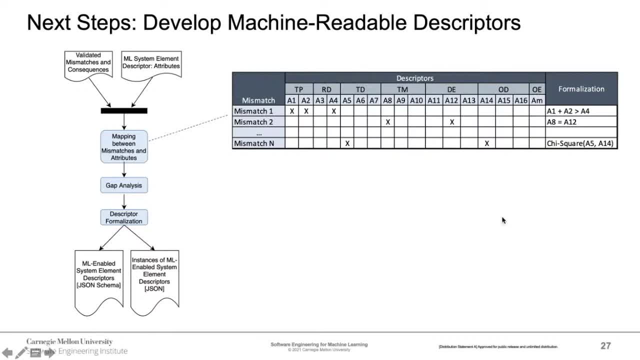 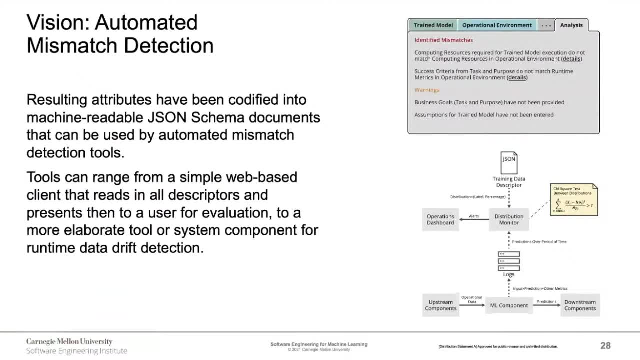 and then the attributes are encoded using JSON schema: notation, Oops, And so our vision. I just want to- we've said this many times, but our vision is automated mismatch detection. Like we said we already, all those attributes have been codified into machine-readable JSON schema. 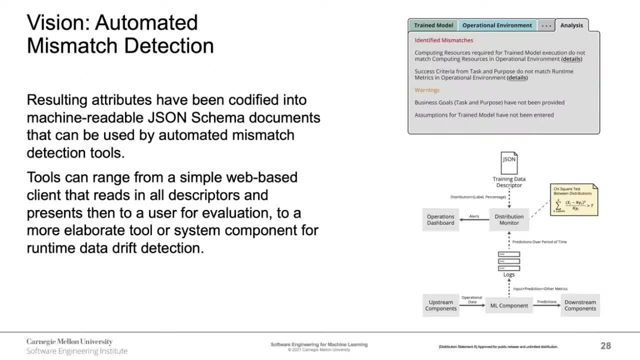 because we want to be able to create tools- us and the community that use it and say okay, because using this information, I was able to create a tool that, at development time, for example, as opposed to deployment time or runtime- 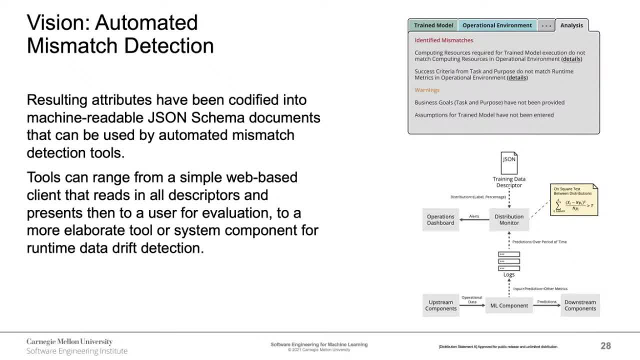 was able to detect that there was a mismatch. There are so many forms of automation and so many tools that we can envision Going all the way from what I would call. the most simple of the tools would be one that, basically, is able to read in the JSON schema. 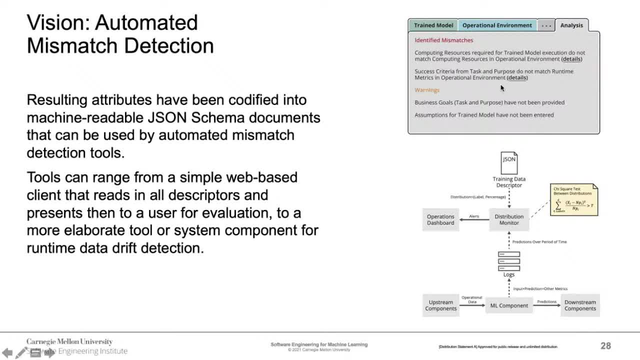 and is able to provide a user-friendly environment so that people, different stakeholders, can fill in the different descriptors for all these and then, for example, have an analysis tab that you say analyze data and would say: hey, here are some mismatches. 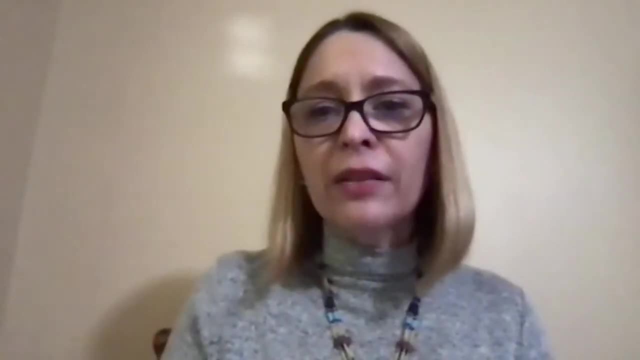 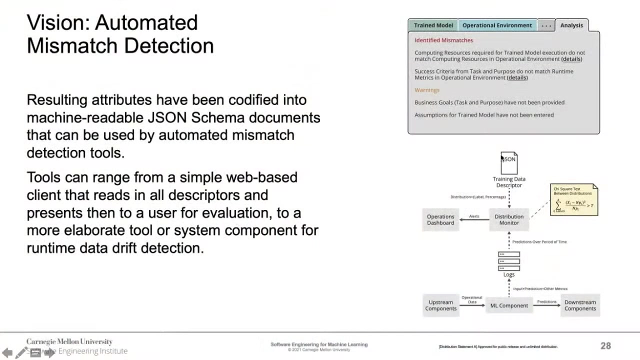 that I identified and some warnings, especially for those that couldn't be fully automated. Or you can have something more complex where you have something called a distribution monitor that is reading in data from the training data descriptor and is doing a chi-square test to compare distributions. 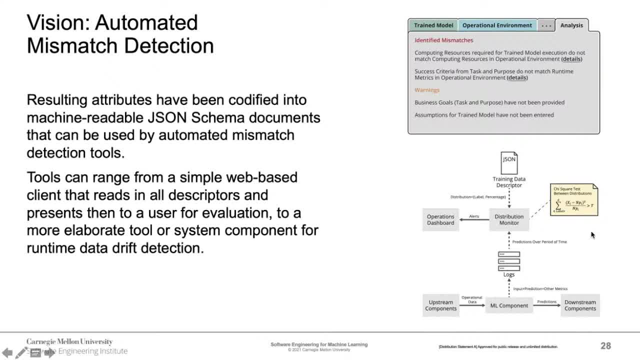 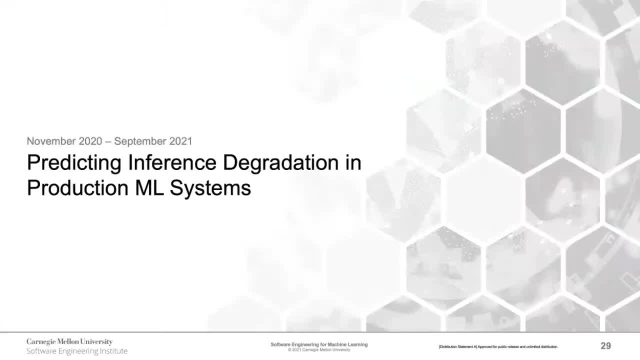 between the operational data and the training data to be able to detect that there's a training serving skew. So with that, Ipek, and before I jump into the next project, do you have any questions? And please give me a time check. 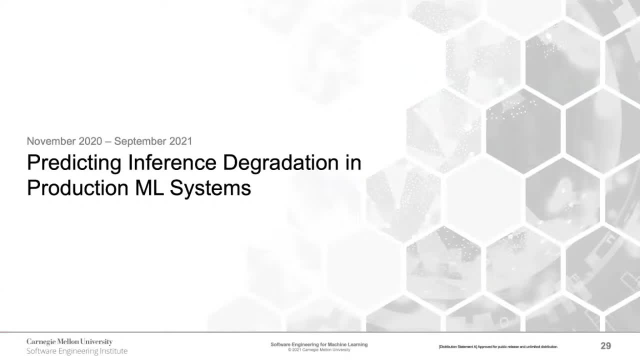 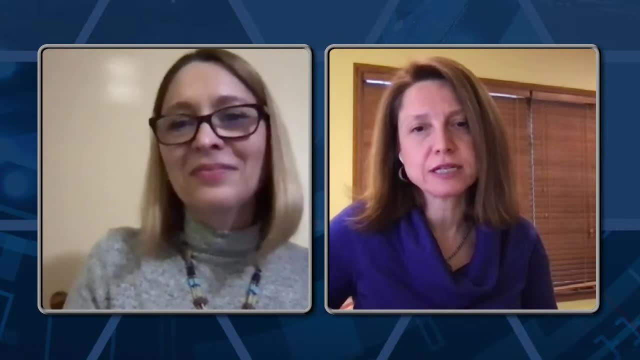 We have about 13 minutes or so, so I think we're doing fine on time. And the next set of questions are actually interesting because it heads into some of the existing tools and the frameworks and what we can do. So let me ask a couple of those. 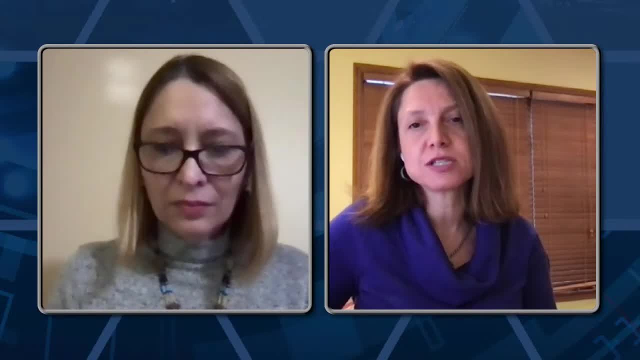 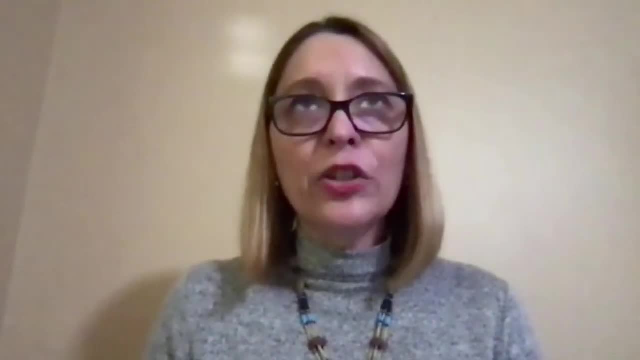 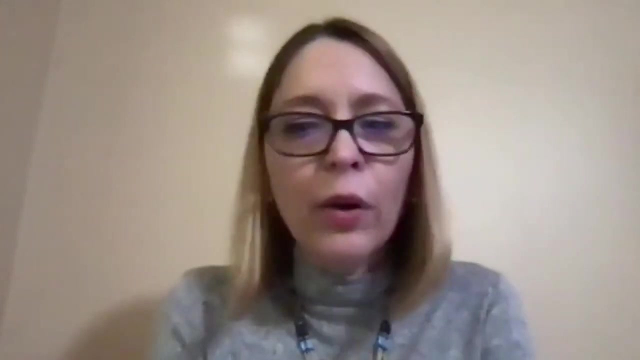 Dwayne asks: do platforms help reduce the risk of such mismatch, such as Azure ML Studio? So I'm not familiar with Azure ML Studio, but I'm going to assume- and you can correct me if I'm wrong- that this is an example of an AutoML tool. 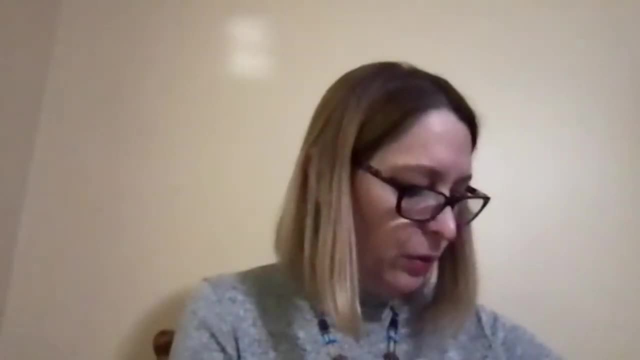 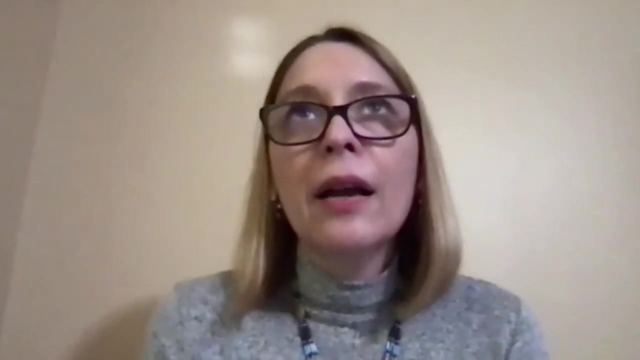 If that is the case, meaning that it's a tool that is going to help me with model development, I think that's a good question. So I'm a software engineer, not a data scientist, so let's keep that in mind as I answer this question. 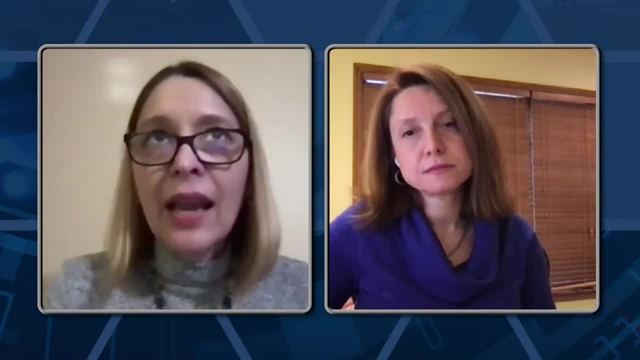 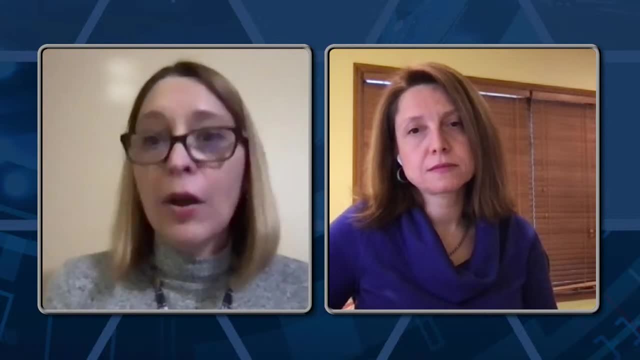 I think those tools are beneficial for the data scientist- and I think that's a good question- And I think those tools are beneficial for the data scientist scientist and for producing a, a, the best version possible of of a, of a model. so a lot of those. 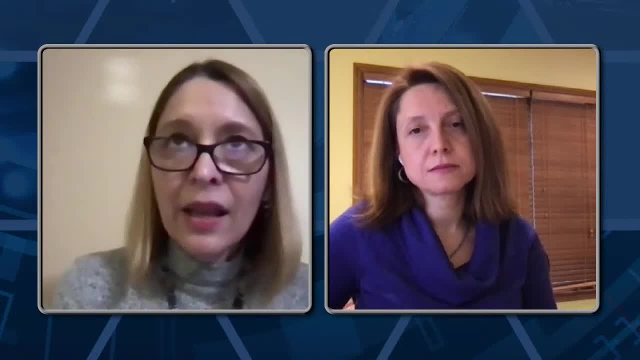 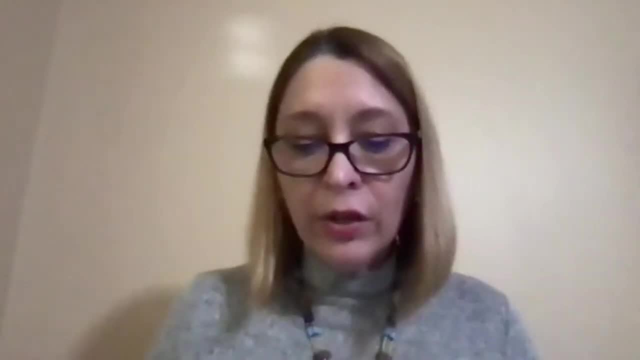 tools, i believe, are more beneficial to the data scientists than to the software engineers or the or the um or the operations staff. however, when those tools are integrated into end-to-end tool chains, like, for example, where i can say, okay, i'm going to produce this model now, i'm going to wrap. 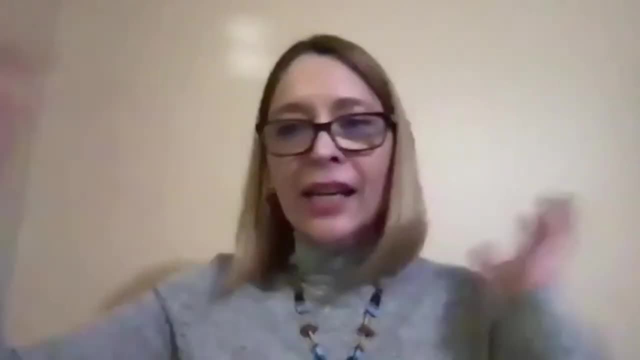 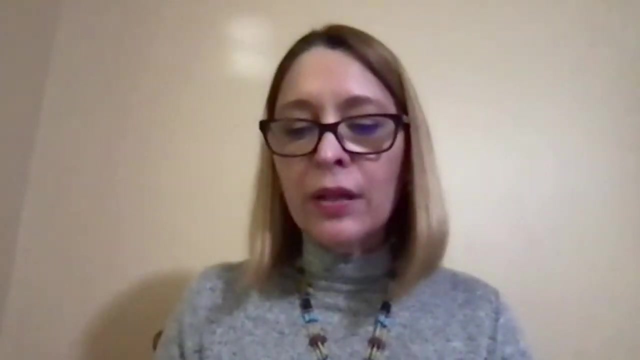 this model as a- i don't know a flask app, and now i'm going to put that inside a container or something like that. i think those definitely definitely help with the mismatch, with some of the mismatches, because, for example, once, if, if you, if you define that in your organization- train. 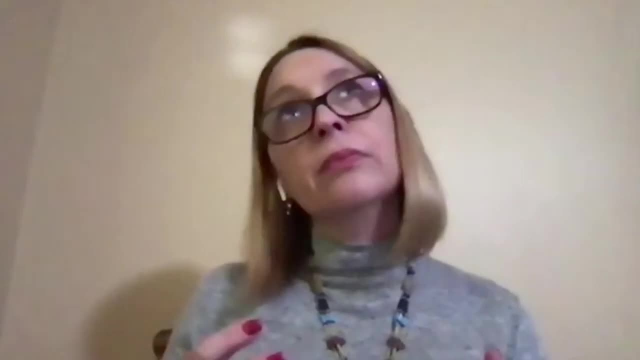 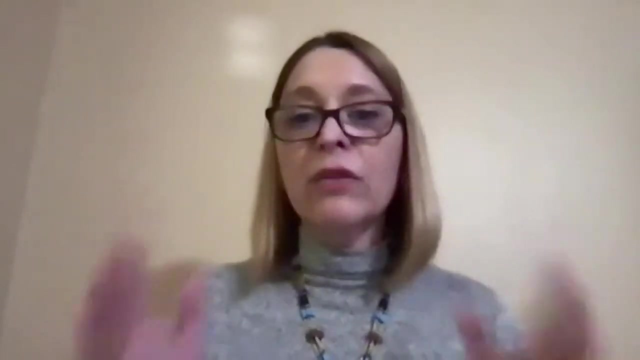 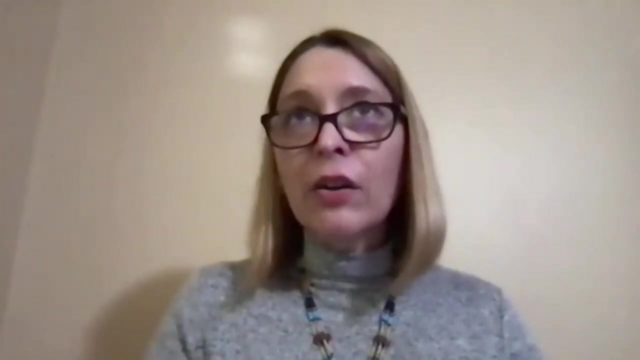 models are going to be um handed over as, for example, containers, uh, or models within containers. that means that you have taken the time to define a very clear api because basically you want to be able to use that, use that container basically as a service. so definitely there are things within tool chains that can help with that, but i would 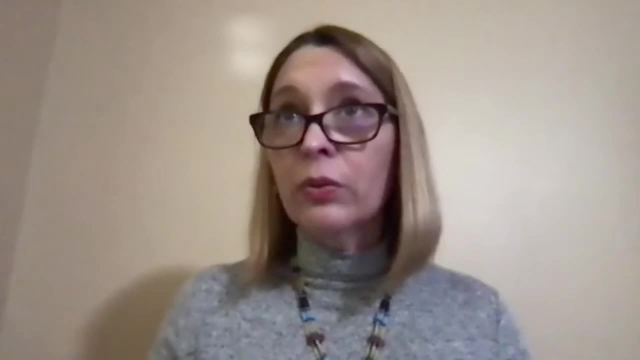 say, if azure ml studio- i'm not familiar with that tool- is similar to to- i would say like to more like pencil flow or or, for example, data robot. i think those are more beneficial for the data scientists and help in creating really, really good models, and michael did clarify that it is. 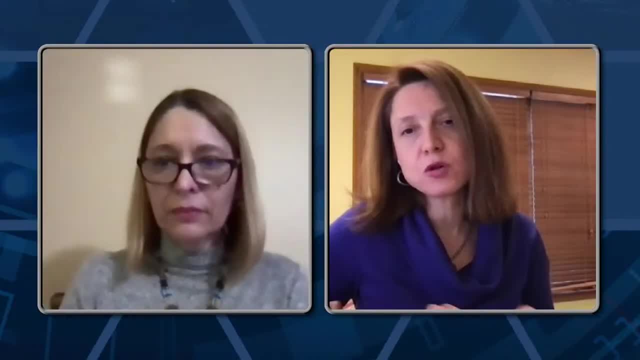 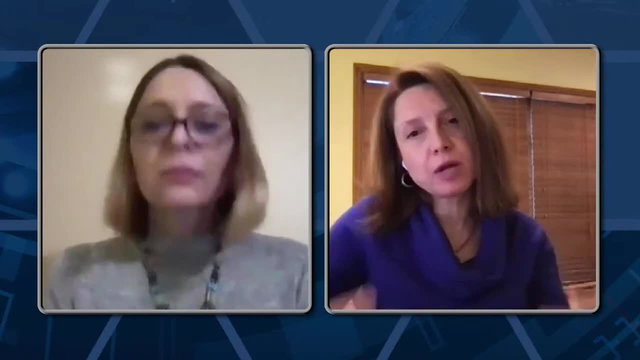 similar to ml model development. so i think you're right on like: yes, those tools have a place to help data scientists, but the overall goal of this is end-to-end system development where ml components is a part of. so it only can go so well, because if you're not, 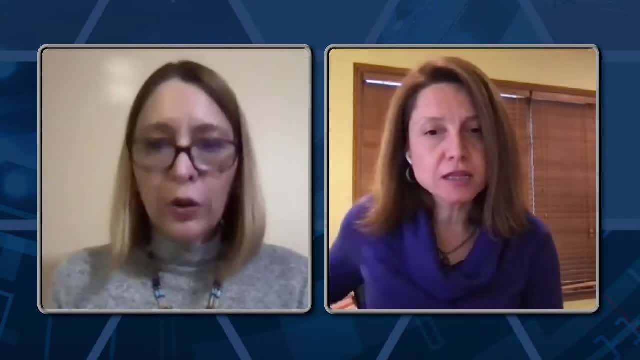 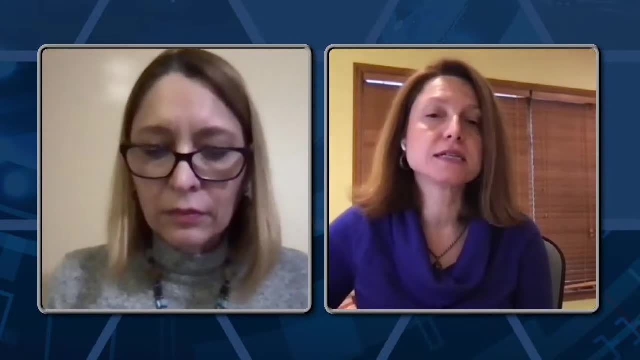 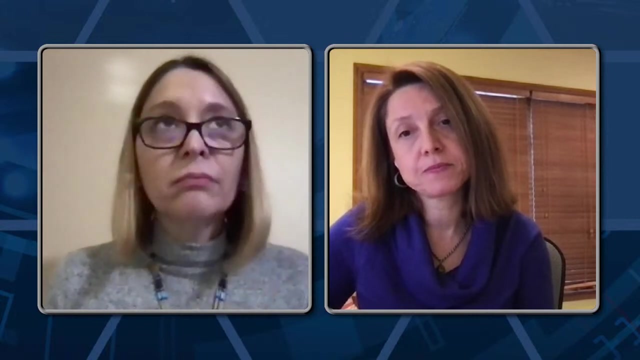 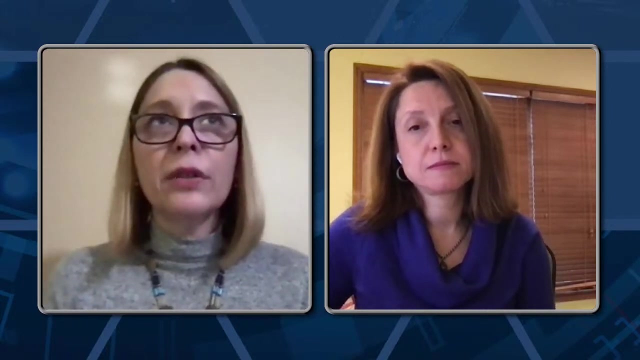 talking from the same sheet of music, you will have similar mismatches correct. the next question is somewhat in a similar lane. looks at goes after data. michael asks: did having democratized data sources, such as data lakes, lake houses, improve around mismatch frequency? i don't know the answer to that because i don't think we got into the details of 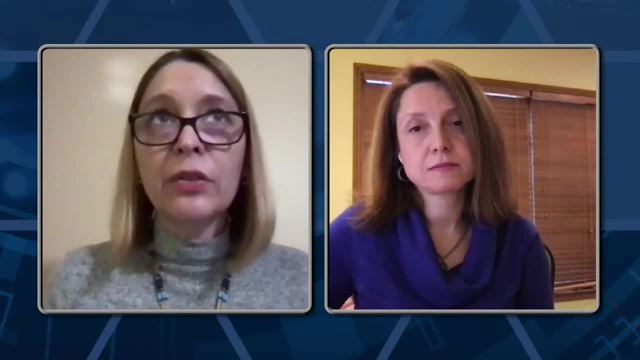 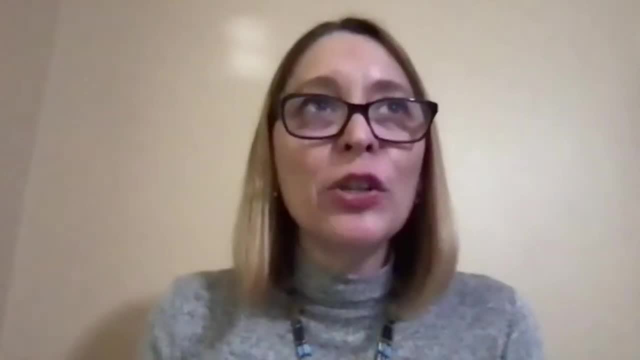 the difference of the different, at least in the interviews. we didn't get into the details of how things were deployed. however, i mean, i'm making a huge assumption here. maybe i need a mismatched descriptor, but i'm making a huge assumption here that those types of of data lakes of what i would 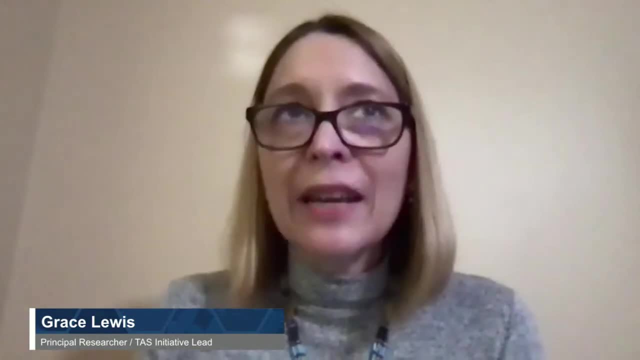 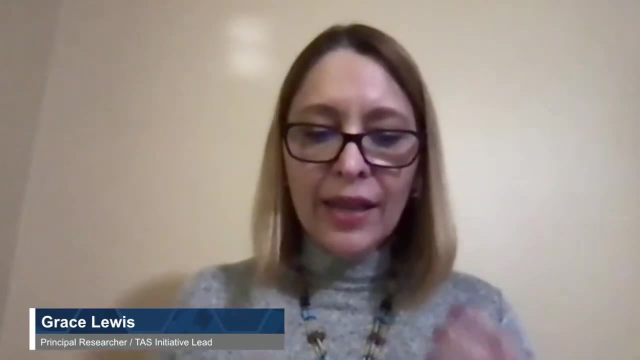 call data. what would i call it like data discipline? i think those would definitely help with mismatch, because you, when you create a data lake or when you create a, a data store of some of some sort, and you and it's in its organizational, enterprise-wide, you would. 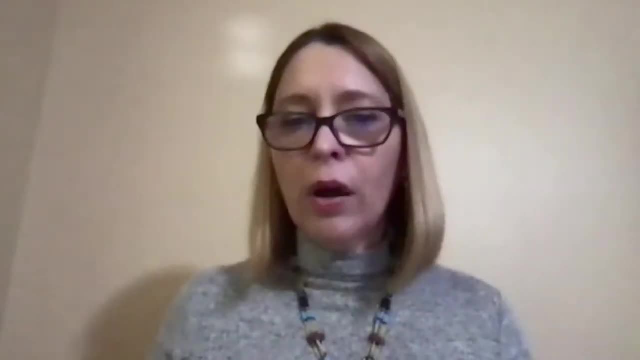 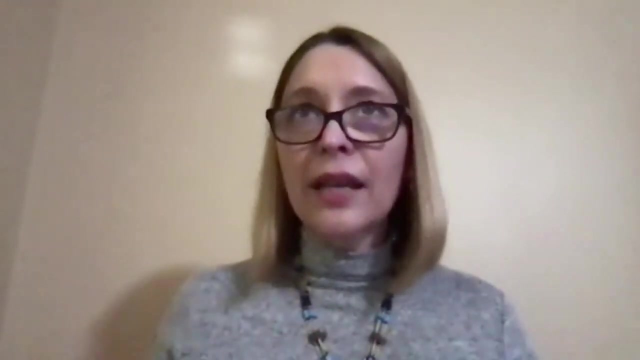 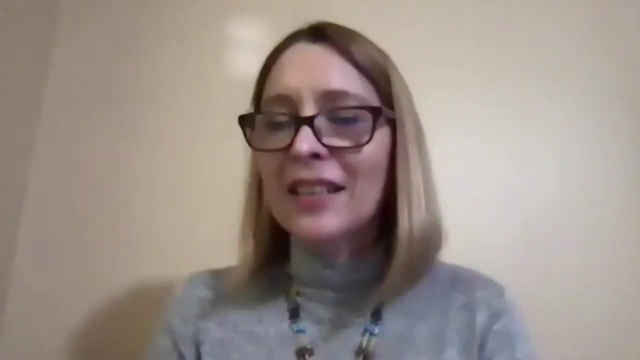 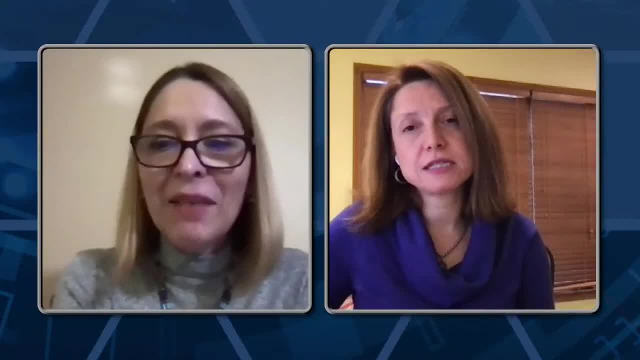 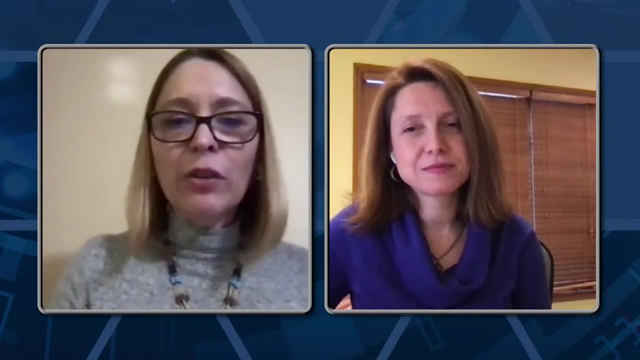 how it's documented. that can definitely reduce mismatch and i'm getting it. i'm getting a 10, i i'm getting a 10 minute time, so let's continue. right, that's okay, and we- and this is very short, but we're going to be talking about this a little bit, if i can just add to that in a minute. 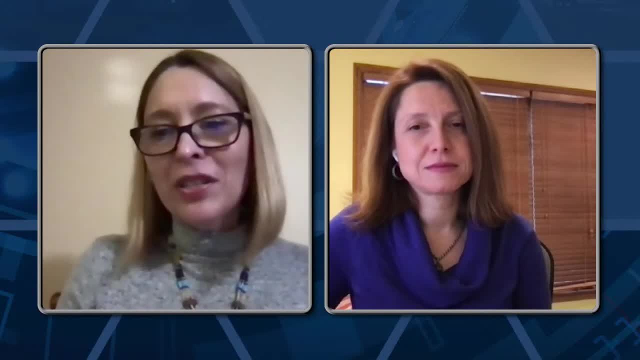 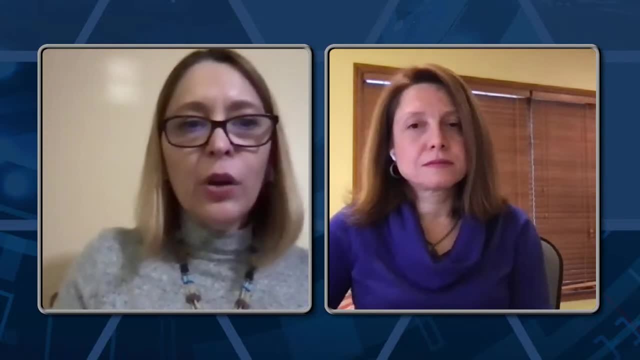 um, the data lake is a very interesting project and we're going to be talking about it a little bit in the next slide, and this is a project that we have started with the msb project. so it was done in june 2020 and it literally just started. actually, it didn't even start november 2020. it. 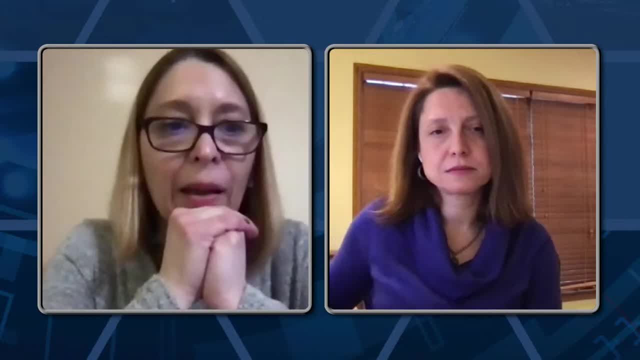 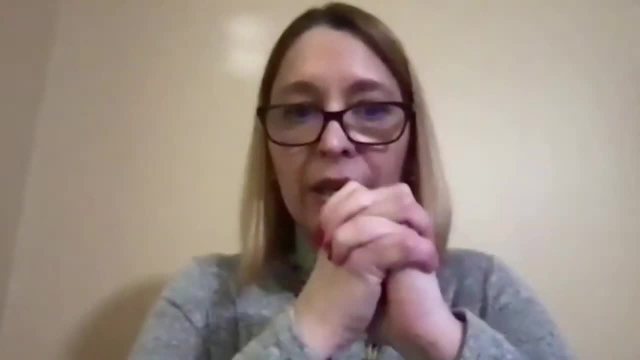 started january 2021, but it's predicting inference degradation and production and now systems somewhat different from what i just talked about, but definitely also in the vein of software engineering for machine learning. It's a fact of life and we're calling it inference degradation. 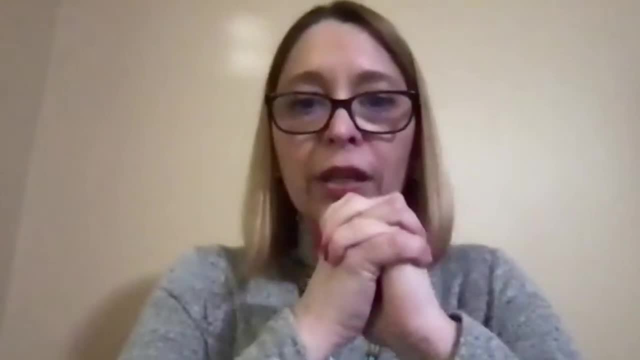 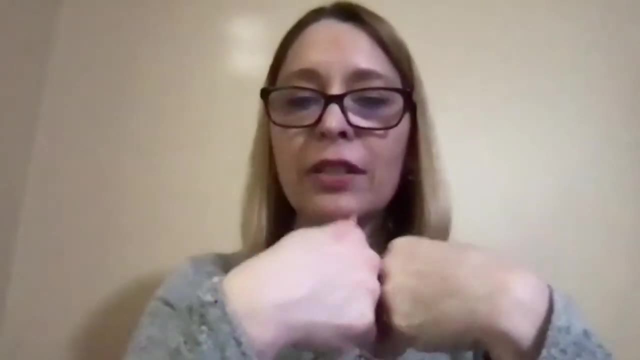 The way that industry deals with inference degradation, especially in large organizations, is they just do periodic retraining. So what happens is that they're not really monitoring to see if inference degradation is happening. they just evade it. they just say: okay, if we constantly retrain. 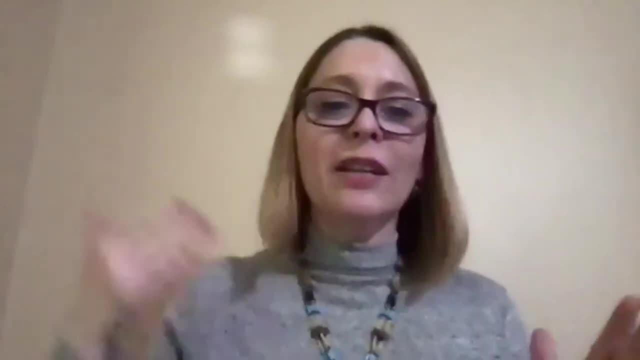 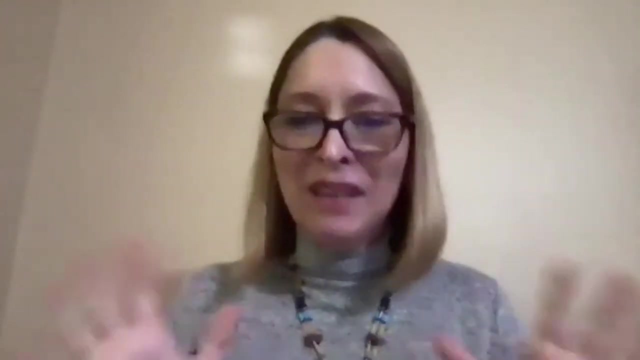 we don't even have to worry about this because basically, you're deploying a new model every day. There are some stories out there that the large companies deploy multiple times a day. That sounds crazy to me, but I believe it. But what we're trying to say here 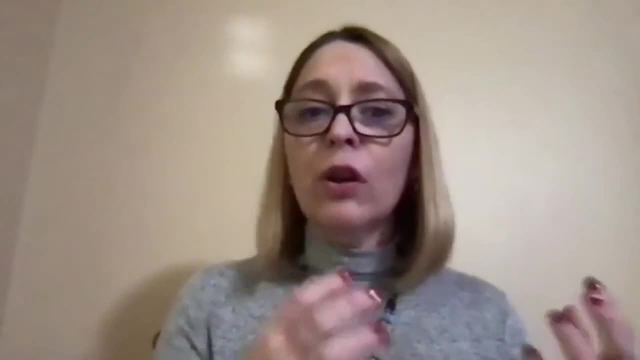 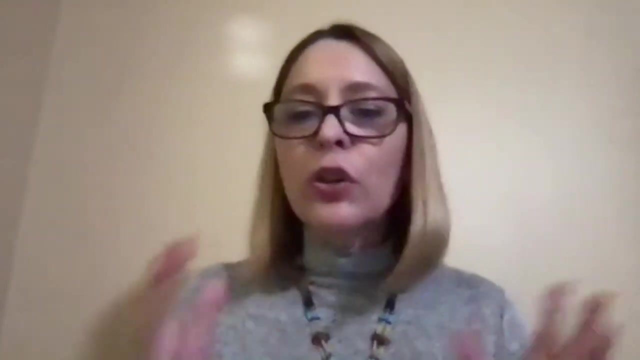 the motivation here is that, while that might be great for large organizations that have lots of data where they can actually do this and they can do a periodic retraining, there are so many more organizations where that is extremely risky. So, for example, looking specifically at DOD applications, 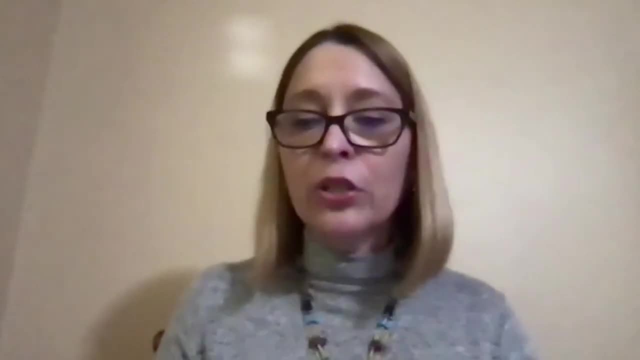 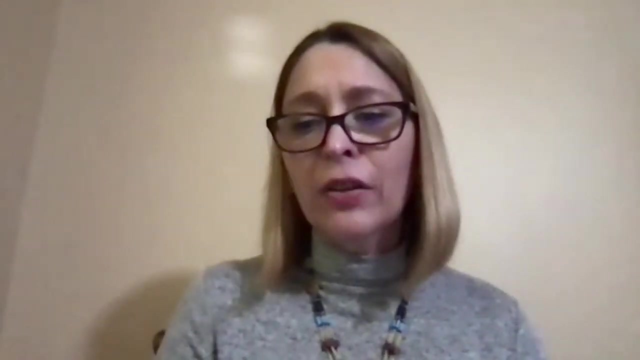 you see that there's a spectrum from enterprise AI to what they call operational AI, which is what's deployed in the field, And when you have AI applications that have fast tempo and where the implications of failure is significant, we think that it's extremely risky. 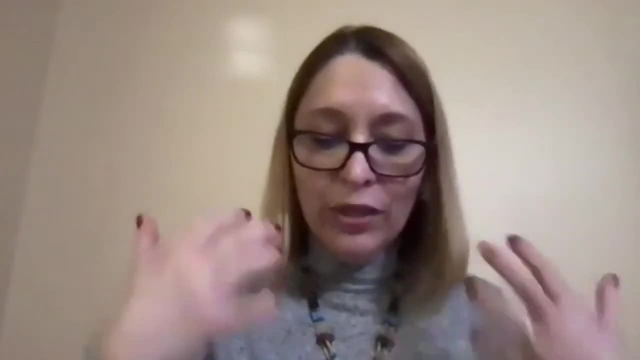 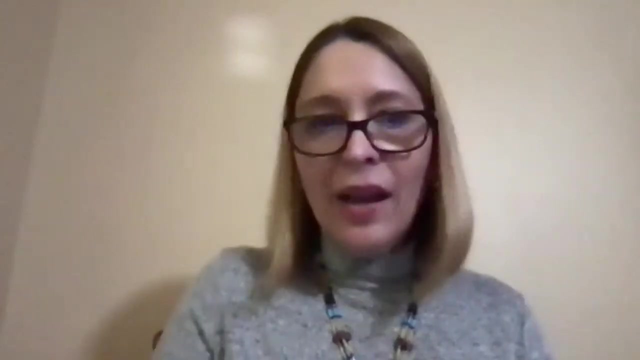 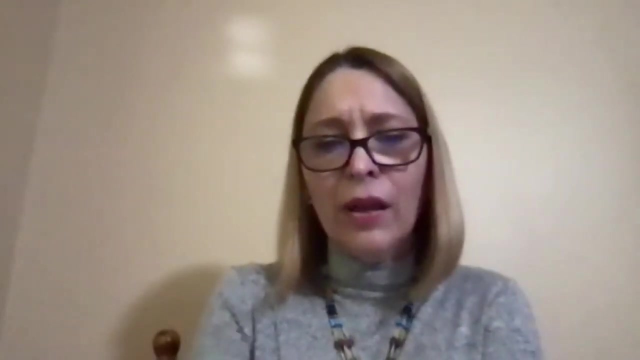 to do a periodic retraining and redeployment strategy if you really don't have, like, a very, very strong infrastructure in place To back that up. the problem that we see is that inference degradation is really it's hard to detect in a timely and reliable manner. 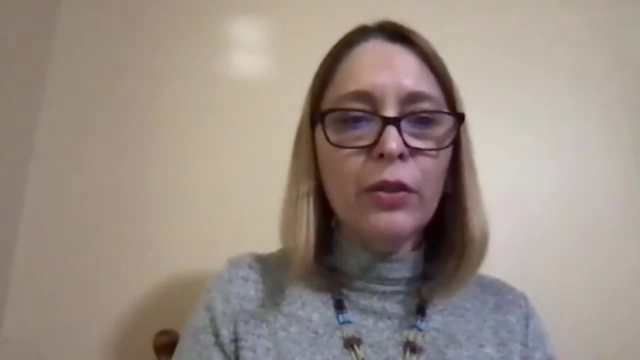 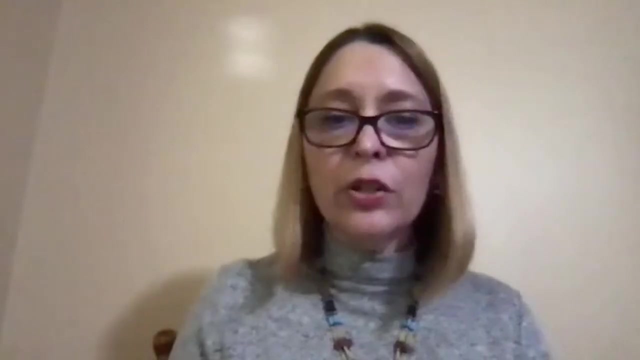 For example, if we look at this graph, let's say that this is over time and this is inference quality. So basically, what this is showing is that the inference quality of this particular model is degrading over time, and this red thing right here is our threshold. 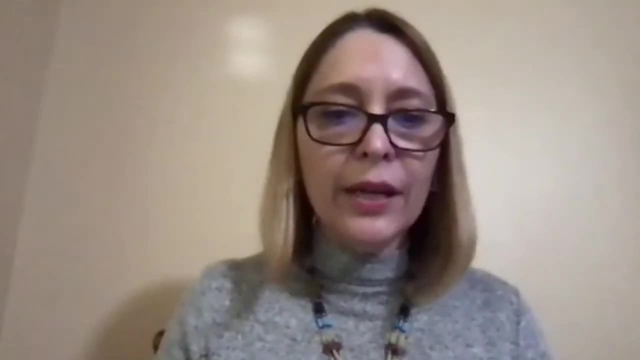 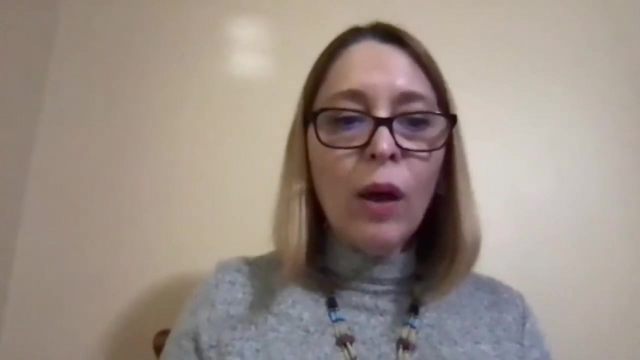 Let's say this is our threshold for acceptable inference quality. So what happens is that if I retrain too frequently, like if this is my threshold, and I'm retraining right here, I'm wasting. I'm wasting resources that I might not have. 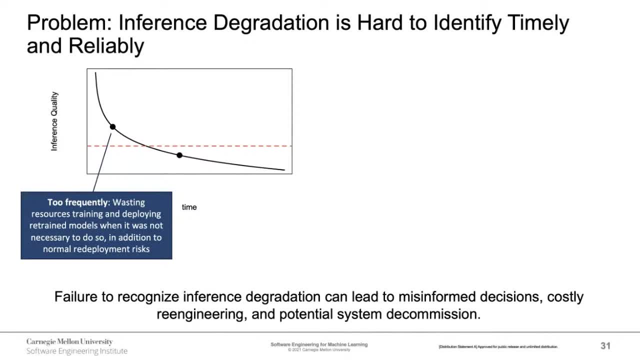 you know, training and deploying retrained models when I didn't have to do so- and also just a normal redeployment risk. Every time you try to redeploy something, it's just an inherent risk. It's just, again, fact of life. 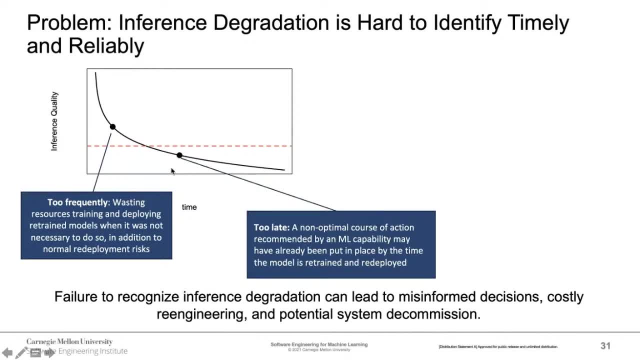 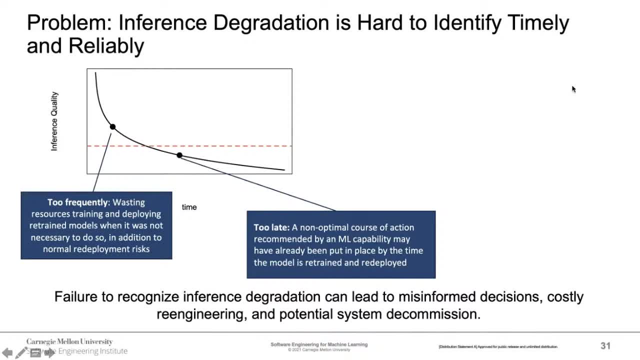 I might be like way over here, So that's also. that's also a problem. On the other hand, inference, quality or drift in this case, isn't always nice and nice and you know, nice curve. It sometimes could be something like this: 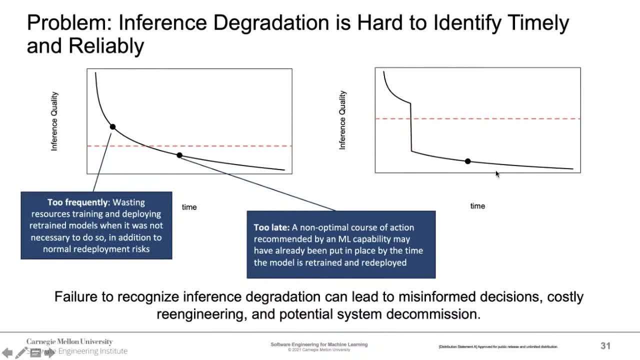 This is. this is an example of a of abrupt drift. So what happens in this particular case is that I would like to know, as a, as as the operator, as the operator of this model, I want to know when this happens. 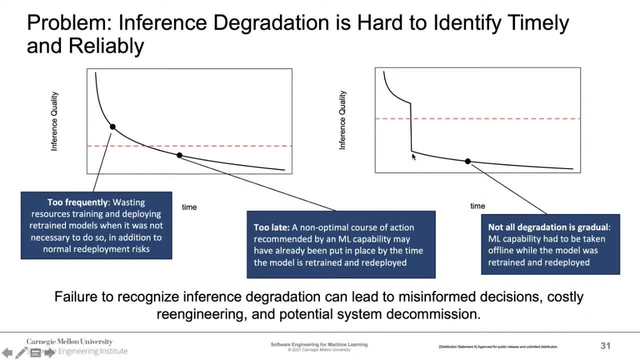 because this this bad of a such a sudden drop in inference quality. it might mean you know what I need to take this model offline. I really can't continue operating this way because it's it's extremely suboptimal. 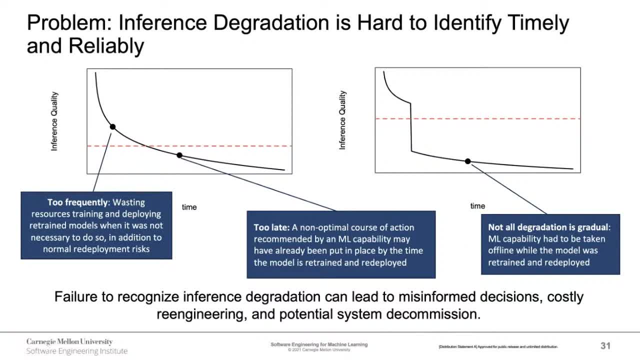 So what we're saying is that if you, if you don't recognize inference degradation in a timely manner, there are so many bad things that can happen, especially when you're dealing, for example, with, with, with situations like this. So what this particular project is is is trying to do. 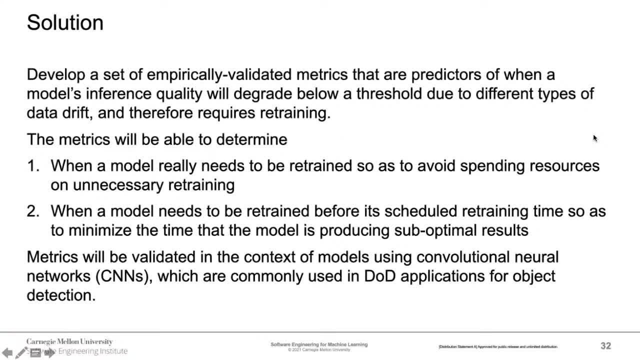 and we're and we're doing it right now- is that we're wanting to develop a set of empirically validated metrics that are good predictors of when a model's inference quality is going to degrade below a threshold due to different types of of data drift. 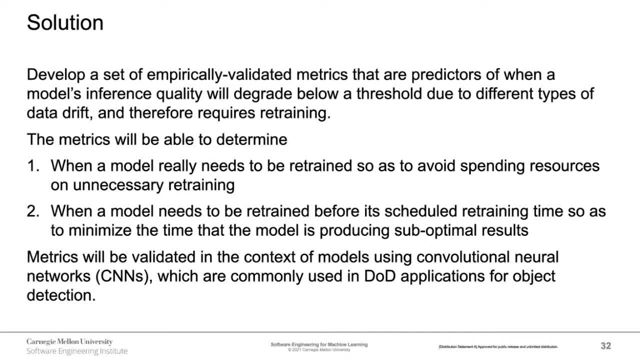 The metrics are not only going to help us determine you know how the model is going to degrade below a threshold. the metrics are not only going to help us determine when a model really needs to be retrained, as opposed to just relying on periodic retraining. 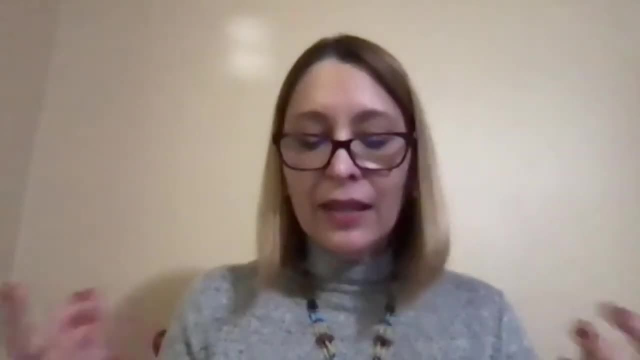 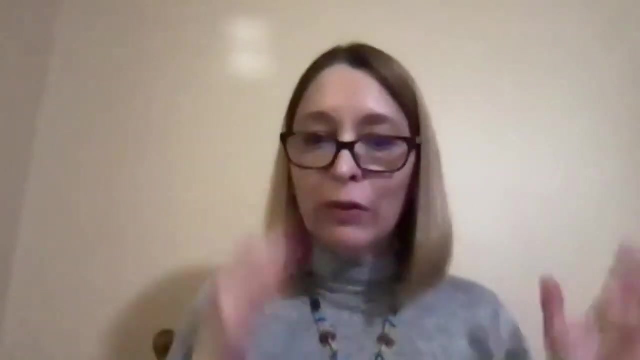 but also tell us like if I, if I know that a model takes- let's say I don't know- 10 hours to train, then I better find out at least 10 hours before so that I have time to retrain the model. 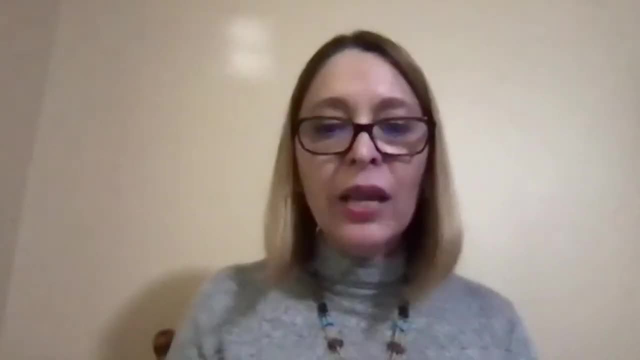 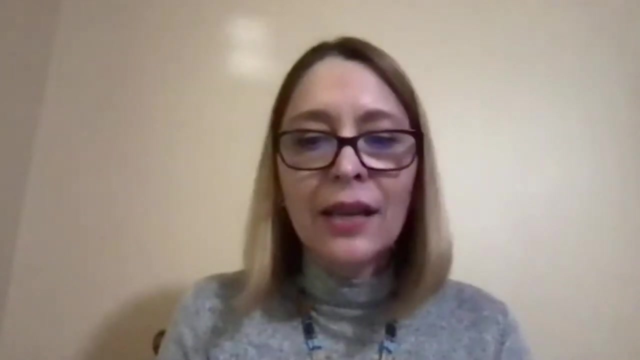 before it goes into a suboptimal- a suboptimal situation Because this is a one-year project. we're specifically going to restrict our our project to to looking at CNNs, which are very common, commonly used in DOD applications. 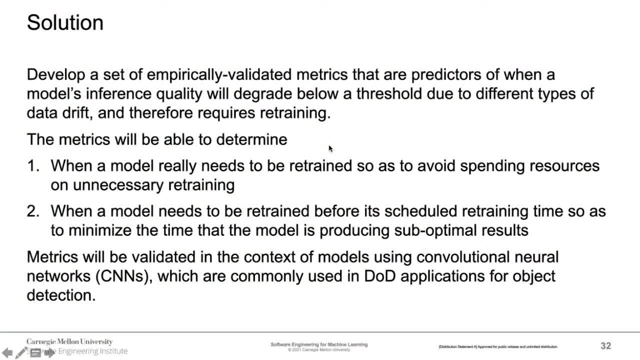 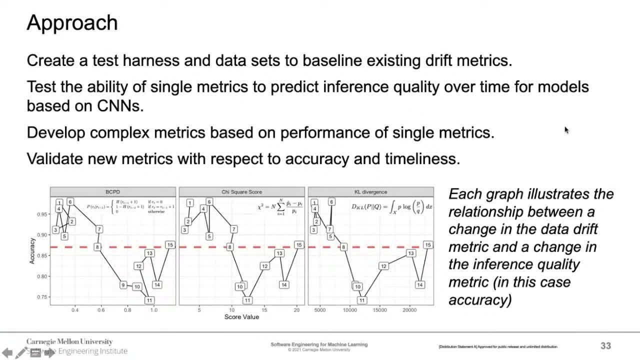 for object recognition. If we're successful, we hope to be able to expand to other types of models. So the approach that we're going to follow is basically we're going to create a test harness and data sets to baseline existing drift metrics. 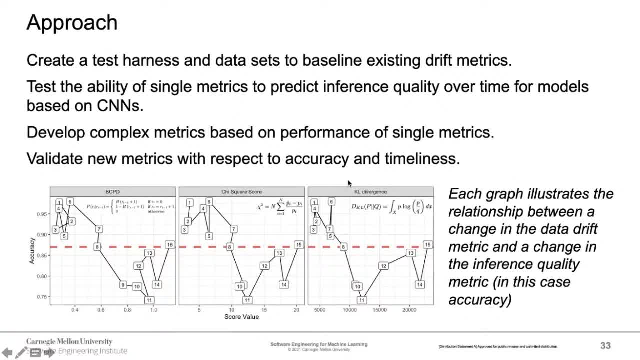 And here are some examples of existing drift metrics: eCPD, chi-square and KL divergence. And we're going to be able to. we want to test the ability of the single metrics to predict inference quality over time for models based on CNN. 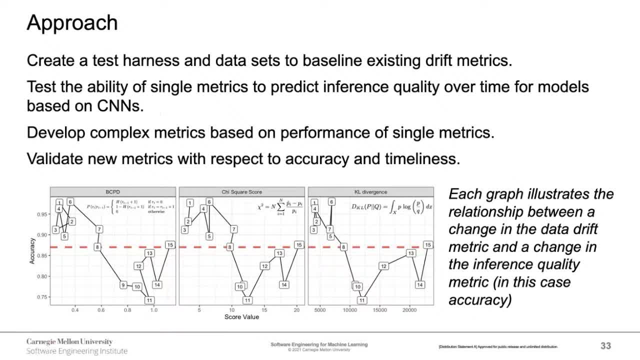 So basically, we have a data set that right now we're doing some data perturbations to it to introduce, to introduce, you know, data drift into them and see how long it takes for these particular metrics to detect that drift has occurred, Once we have a baseline of existing drift metrics. 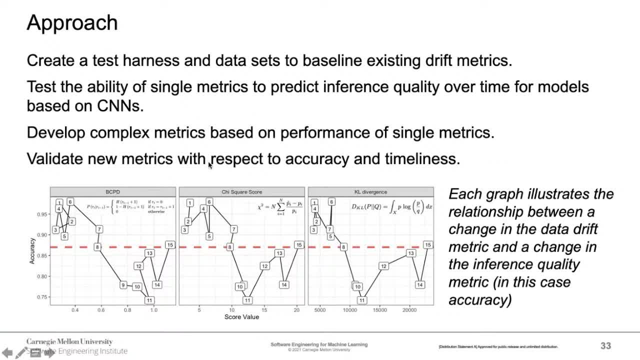 what we want to do is we want to start combining them and developing complex metrics to see if maybe a combination of metrics is a better thing to have, because that way you can detect different types of drift, Because it could be that, for example, KL divergence is good for detecting one type of drift. 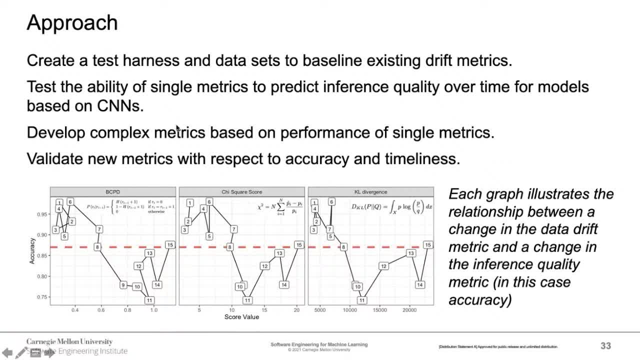 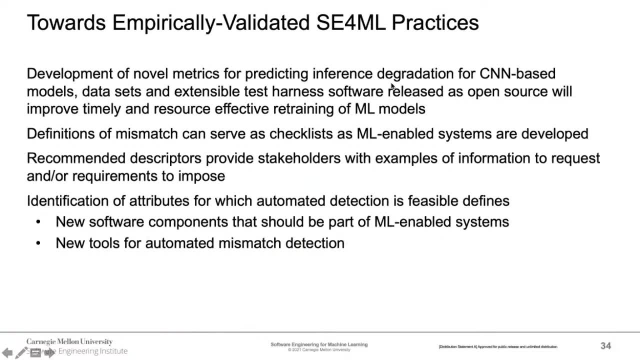 but BCPD is better for detecting some other type of drift And obviously we're going to validate these metrics with respect to the baseline. So- and this is my final slide, Ipek- So our goal is really empirically validated SC4ML practices. 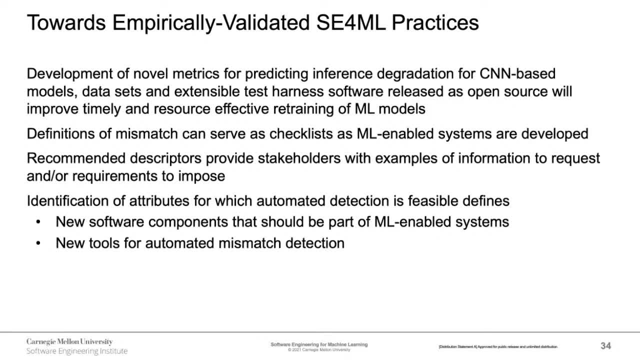 That is the goal of the group in which I work. So, in this particular case, developing these novel metrics and also the test harness and making it available as open source is going to- we hope is going to- improve the practice of effective retraining of machine learning models. 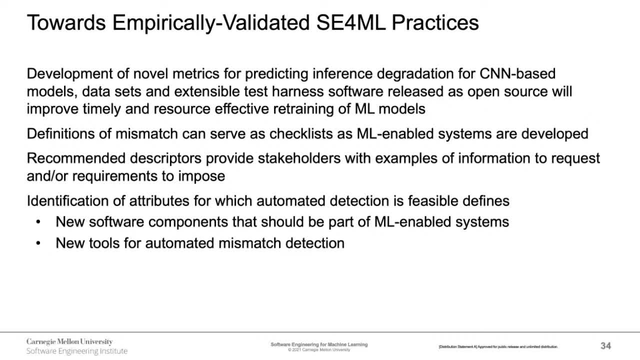 The mismatch, the descriptors that we talked about before. we are, we envision them, and we hope to continue doing so, that they serve as checklists as these types of systems are developed and that, for example, these descriptors are starting to be used as kind of like requirements. 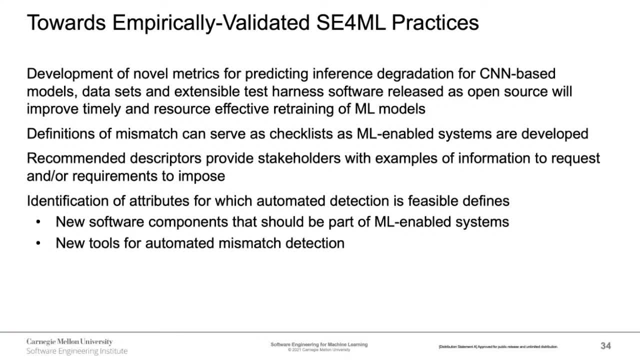 when people develop different types of parts of the system. And obviously our goal, especially for the first project and obviously for the second, because eventually we do want to be able to integrate these metrics into a tool- is that we want to be able to do automation. 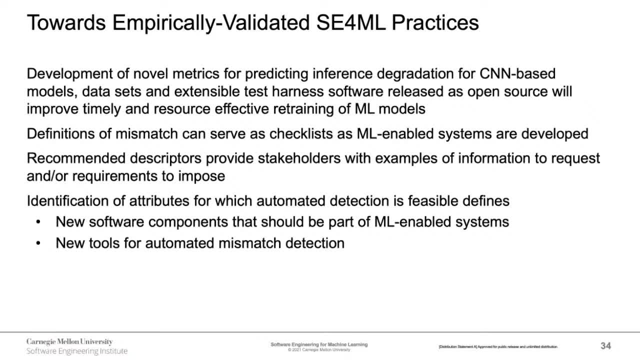 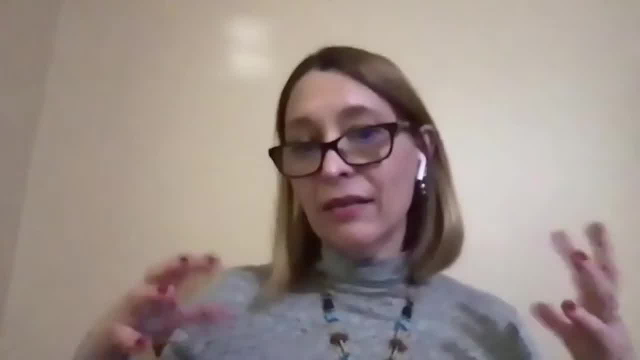 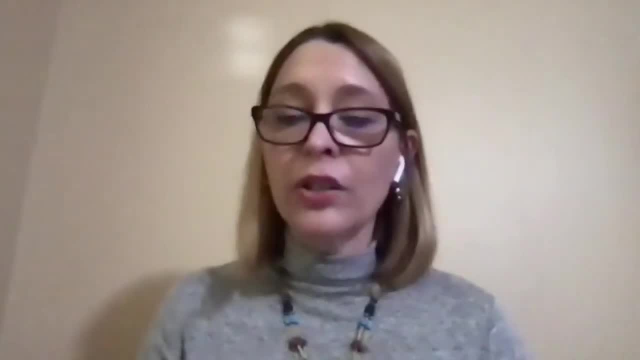 new automation when it comes to mismatch automation for determining, for example, if I want to detect mismatch at runtime, which are different system components, that could be part of the system- or automated mismatch detection. it could be design time or runtime. and if we take it further into the second project, 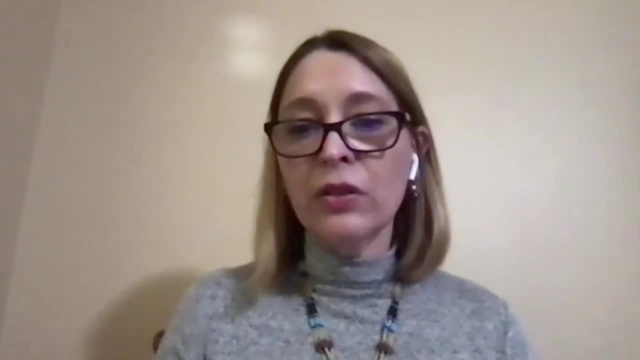 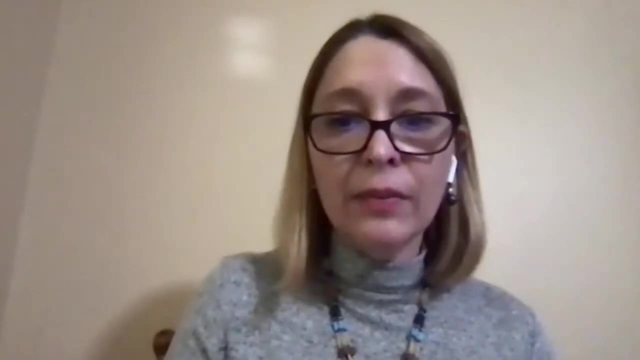 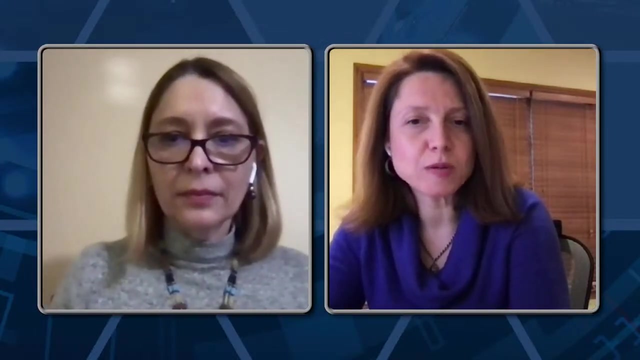 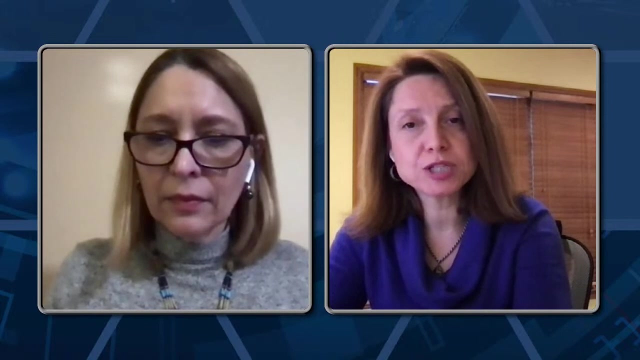 imagine having these metrics built in to monitoring systems to be able to inform different stakeholders that it's time to retrain a model. And with that, Ipek, I am done with my presentation for today. Hello, All right, sorry, hello. 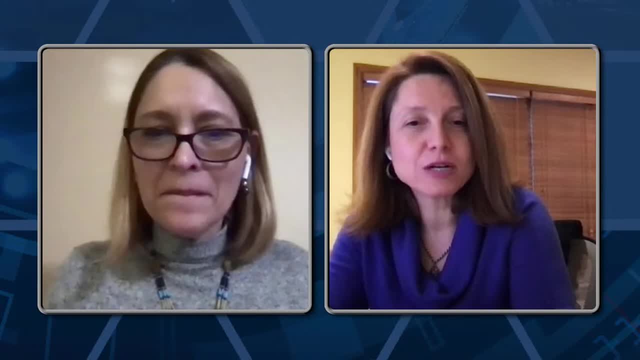 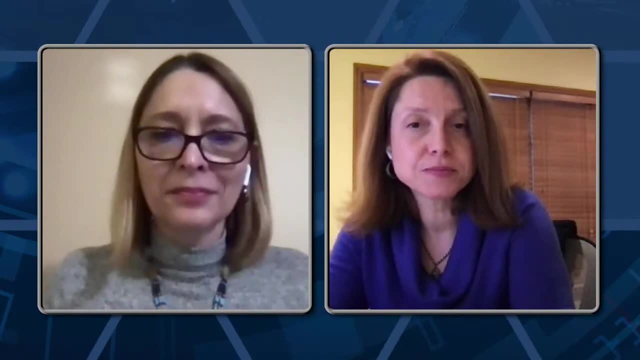 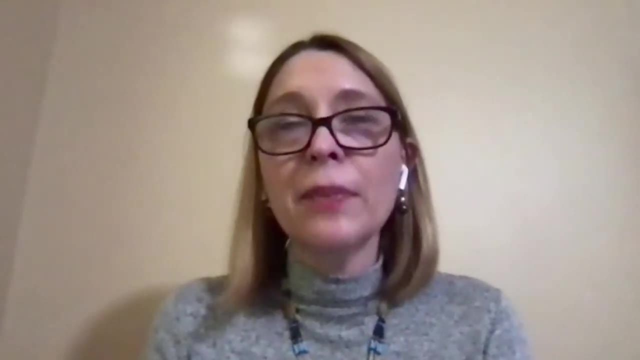 I'm going to take one last question and then also end with a comment. The question comes from Mike and the question is: would you envision this automation as part of the build pipeline, or even earlier, Even earlier, definitely even earlier, because some of the mismatch, for example, 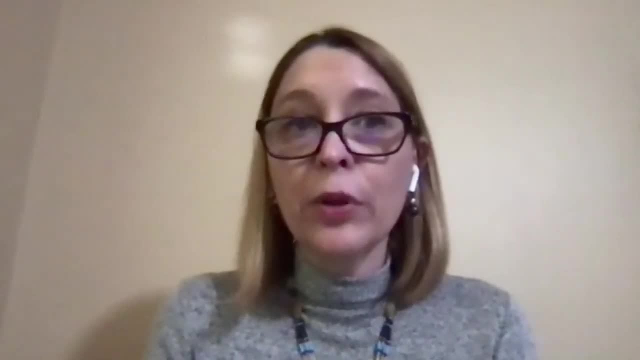 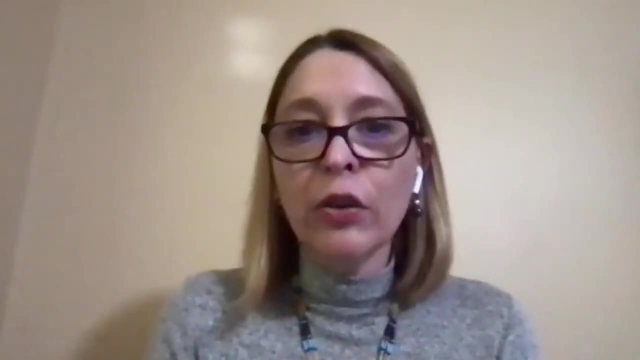 if, as a data scientist, I am aware of the computing resources that are going to be in the operational environment- because that's one of the descriptors- I might make different decisions or make different trade-offs, saying: you know what? I want to get a model. 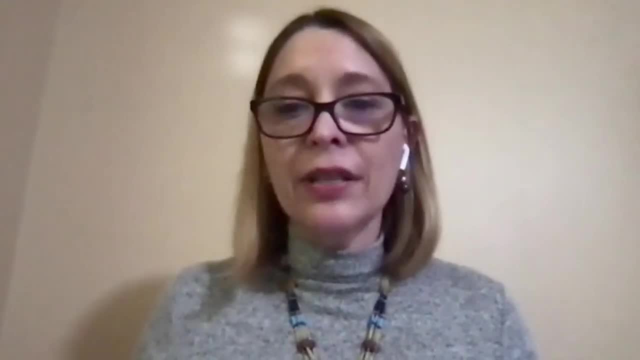 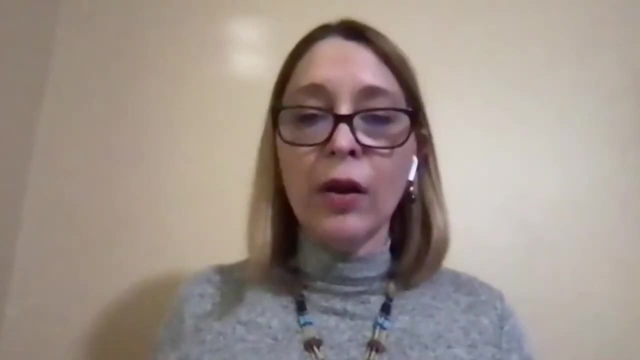 that's 99% accurate. but it's going to be impossible to get that accuracy if that model is, if I'm not going to have the resources at runtime to execute that model. So definitely way, way, way before. or, for example: 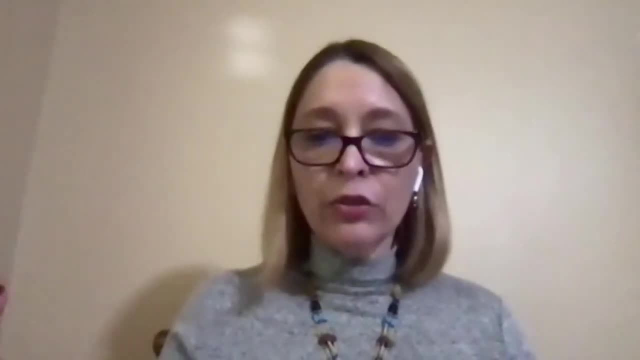 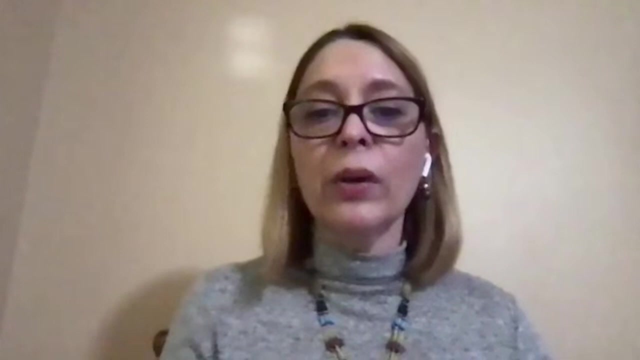 if I know what the API is of the different components of the upstream and downstream components of the model. again, as a data scientist, I can take this into consideration when I'm building my data pipeline in my model, and it goes the other way around. 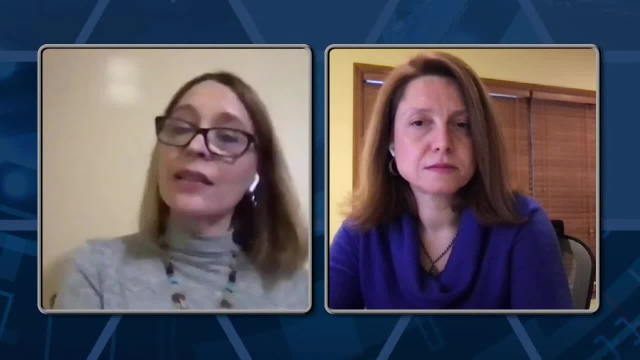 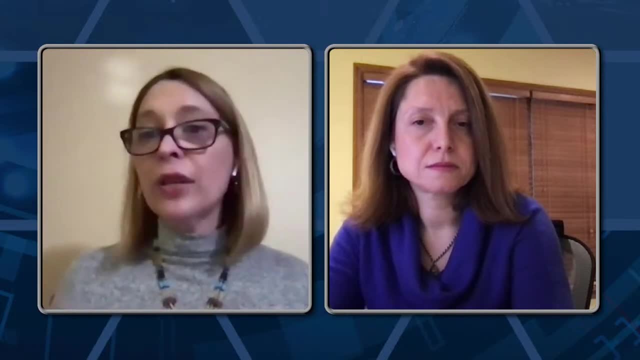 If I know the language that the data scientists are using- and I'm a software engineer- I might make different decisions as to why. I might make different decisions as to what language I choose and also, for example, schedule decisions, depending on whether I decide. 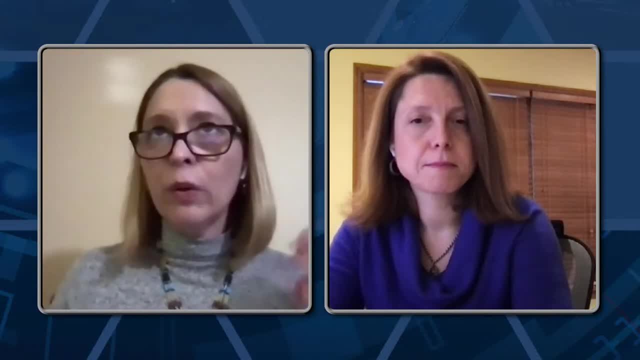 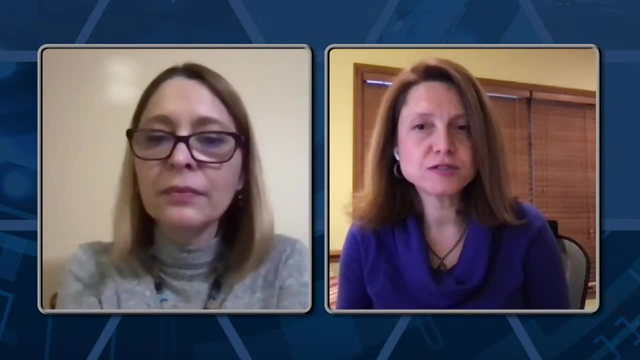 to port that or not. So definitely way, way before We see these being used both at design time and runtime. Yeah, so there's definitely an end-to-end perspective and an opportunity, Correct? So I think, in the interest of time, let's stop here. 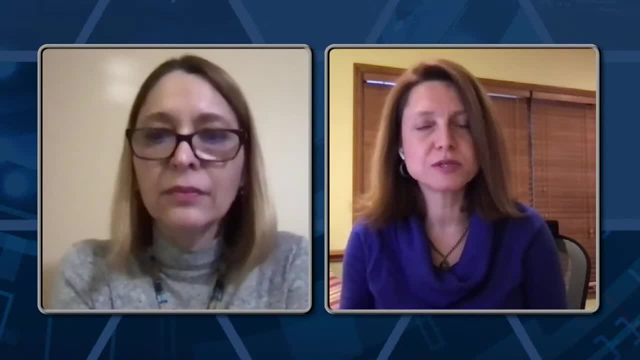 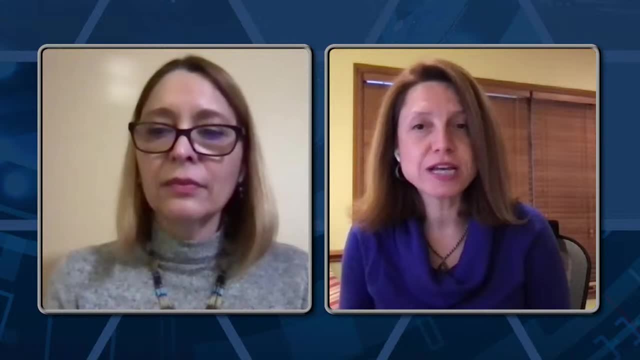 Thank you very much for updating us all on the progress on the projects and some of the what's upcoming. We will definitely come back and do more of these, both from us and other members of our team, And I'm going to end with a comment. 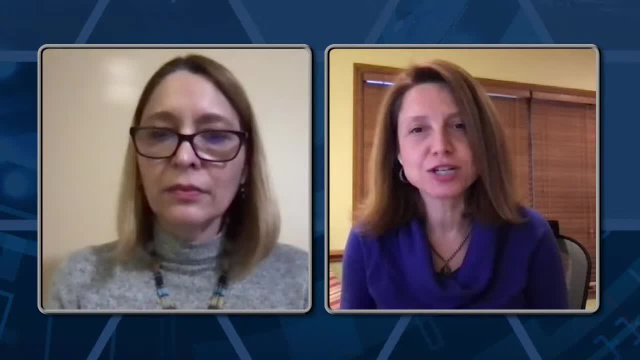 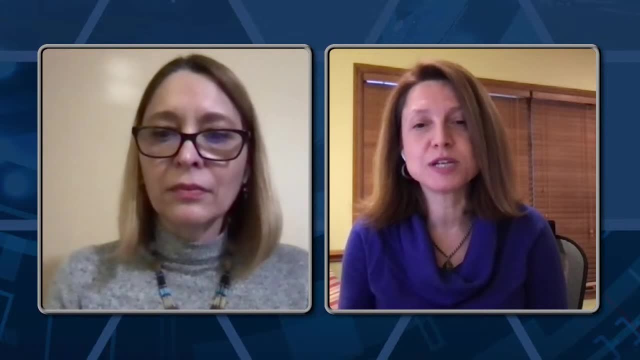 that Peter Boatman put on the chat- and I apologize if I'm not doing justice to these names- And the comment is: I'm a software engineer, not a data scientist. Well said, Grace, you speak for most of us, And all the data scientists we talked to did actually say: